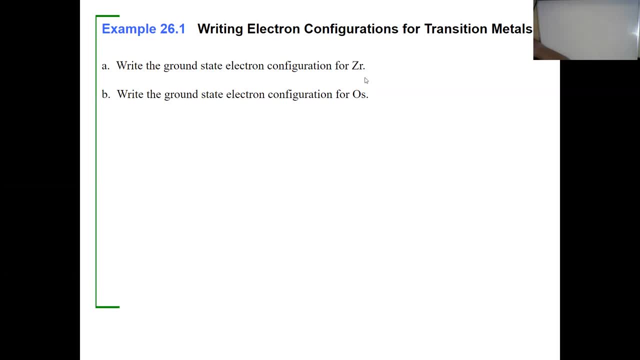 Okay. so it's important first to know how to write the electron configurations of your neutral ions. Now I think it's a good idea to kind of use your periodic table as a guide for this. All right, so I am going to. 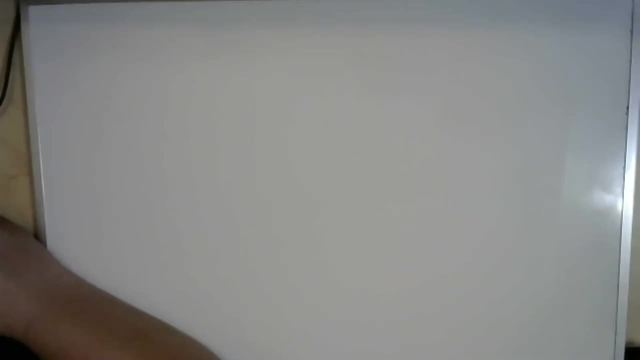 I'm going to share my my desktop real quick And we are going to look and see how we can find the electron configuration, The electron configuration of zirconium, using the Like, just using the periodic table. Okay, Sorry, I'm not very tech savvy, so it takes me a second to do what I want to do. 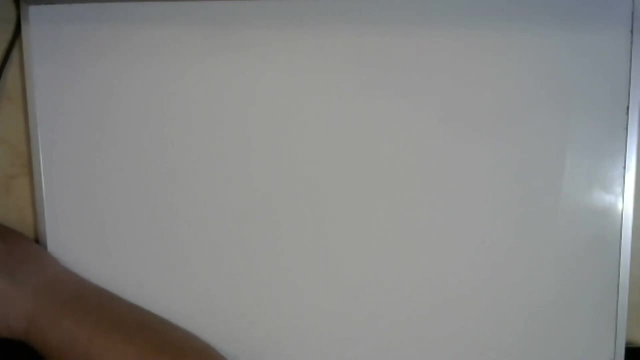 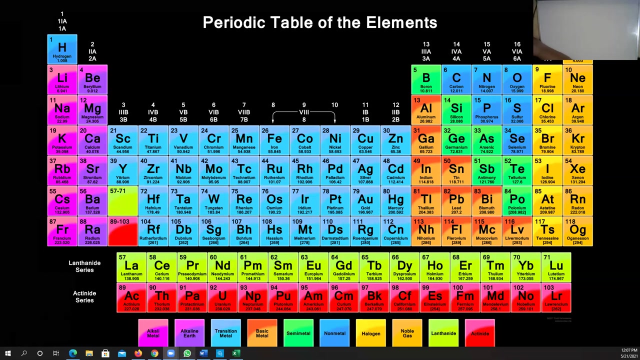 All right, Okay, Move this here. Okay, So now I'm going to share. So now you guys can see my periodic table. Hopefully I'll laugh if that's not true, And we're going to actually use my little spotlight. 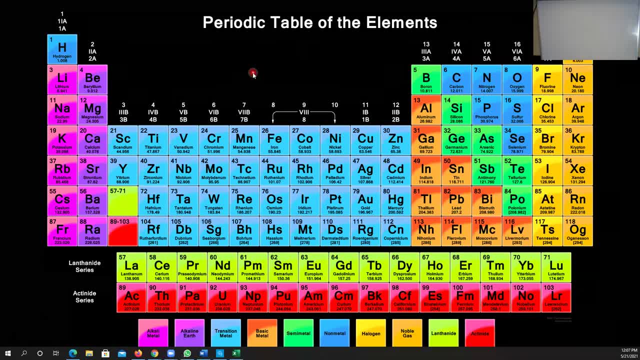 I'm going to show you how I write out the electron configurations using my periodic table. We're going to start with the zirconium electron configuration. Okay, so the first thing I'm going to do is I'm going to find zirconium on the periodic table. Okay, it's over here. it's number 40.. All right, and I would like. 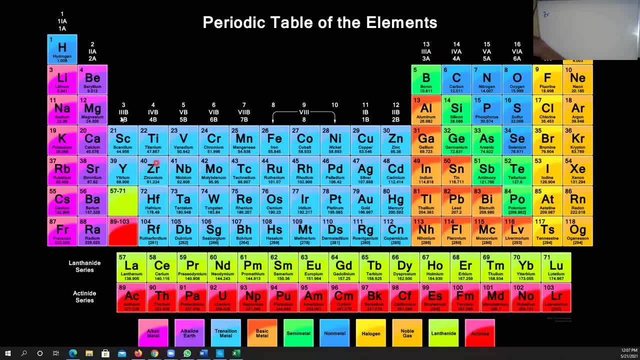 to remind everybody about the different blocks of the periodic table. now, The first two columns are called our s block- Okay. our last six columns are the p block, and this inner rectangle here is the d block. Okay, and then these two rows over here which are expanded below, this is our f block. 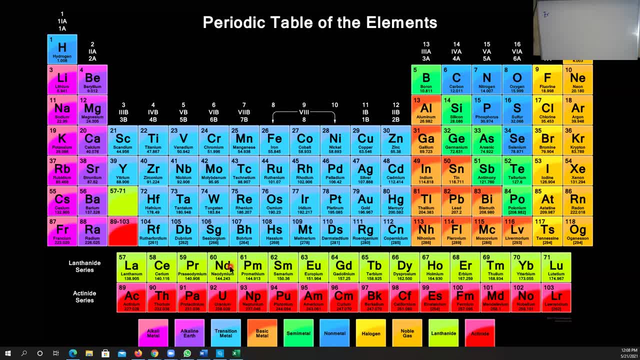 All right, and that's going to be describing the types of valence electrons that these things are going to have. All right, now, if we're going to figure out the, the corresponding energy level for each of these letters, which represent sub-levels, we can look to the rows. the row: 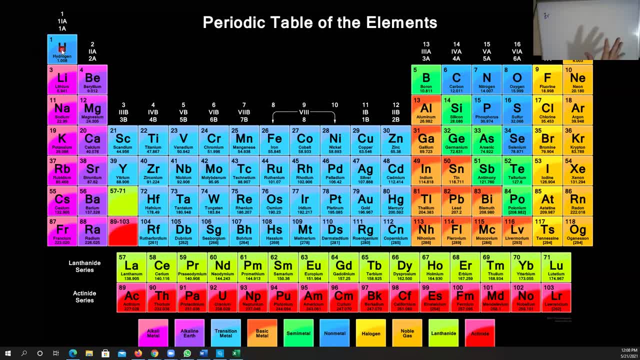 number for each of the periods To find that principal energy level. So row one is going to represent our 1s group. Row two will be 2s, 3s, 4s, 5s, 6s, 7s, Okay, and the the n value for your s sub-level will be the same as for your. 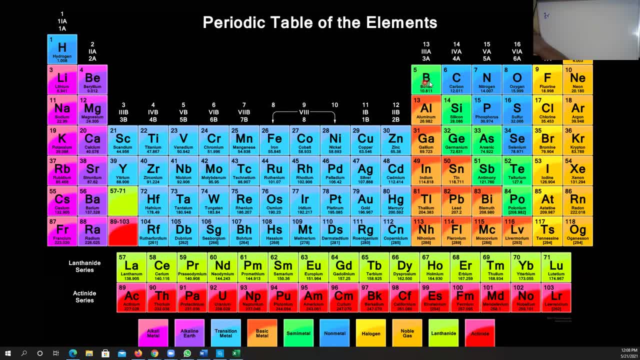 p sub-level. So if you have like 2s when you come over here, this little row here of 6 elements will be your 2p elements, These are your 3s elements and then these will be your 3p elements. Just know that this helium, even though it's over here, you can imagine that it sits right. 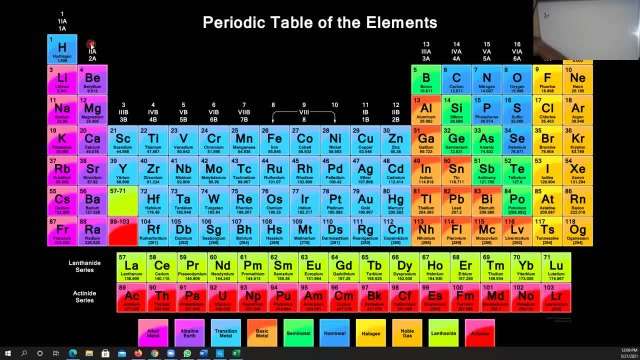 here next to hydrogen. So hydrogen would be 1s1 and helium would be 1s2, because those are the only two elements that only have period one electrons- or energy level one electrons only Once we move on to the d block of elements, which is where we spend most of the time in this chapter. 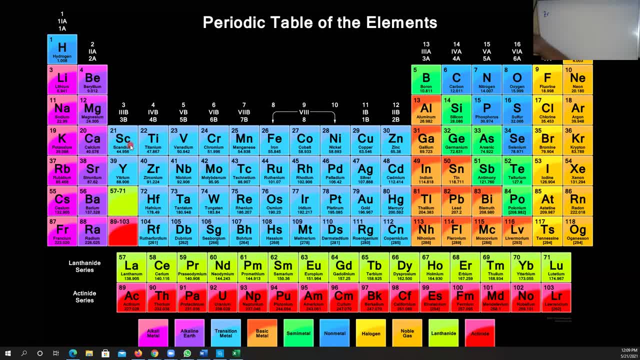 we have to remember that the d sub-level corresponds to one principal energy level below the s level that precedes it. Okay, so for this first row of our d electrons here, we are going to be in the 4s sub-level when we're in, you know when we have our first, our potassium and our calcium here. but 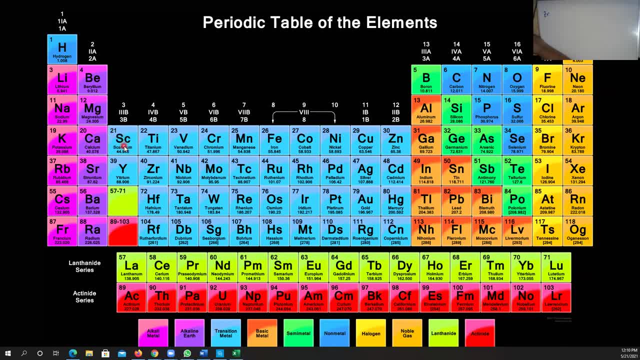 when our our d electrons start, scandium starts with 3d1.. Okay, so this is 4s1, this is 4s2, this is 3d1, then 3d2, 3, 4, all the way up to 3d10.. When you move over to gallium, you jump back up to n. 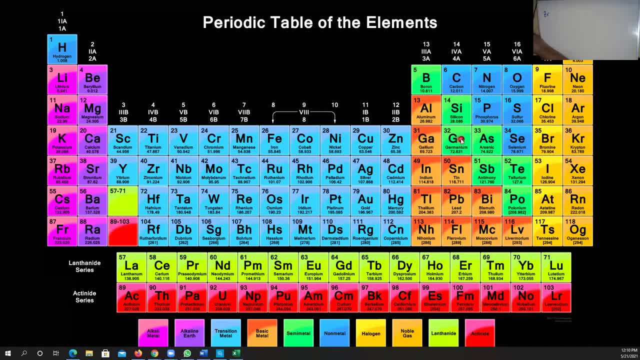 equals 4.. So this is going to be 4p 1, 4p2,, 4p3, up to 4p6.. All right, and the same thing is going to happen here. this is 5s1, 5s2.. 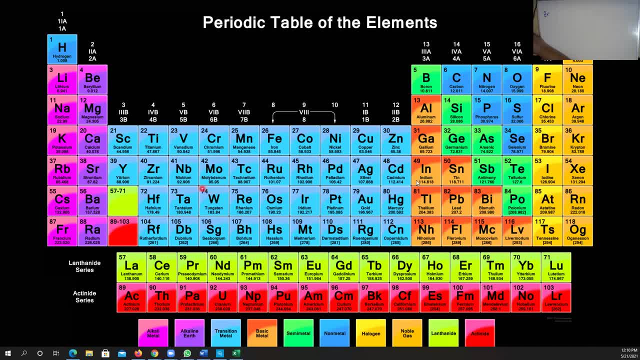 Atrium is 4d1 up to 4d10 and then it jumps back up to 5p. All right, so, like I was saying with zirconium, the way that I would write my electron configuration for this is: first I'm going to find zirconium and then I'm going to go back to the noble gas. 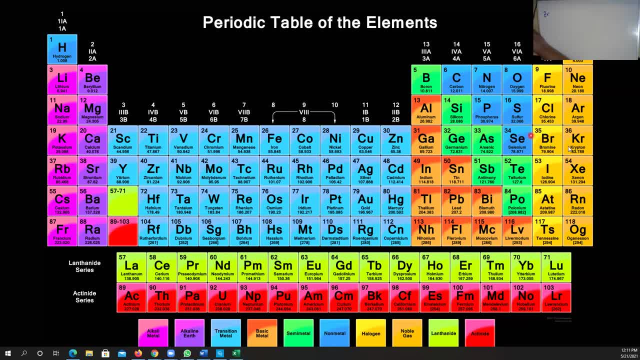 that comes right before it, Okay, so that's going to be noble gas. 36, krypton: Okay, and I'm going to put krypton in brackets, Okay, and then I can use my periodic table to fill in the rest of the electron configuration, because I know that this, right here, this is my 5s sub-level, this is 5s1, this is 5s2.. So I know that. 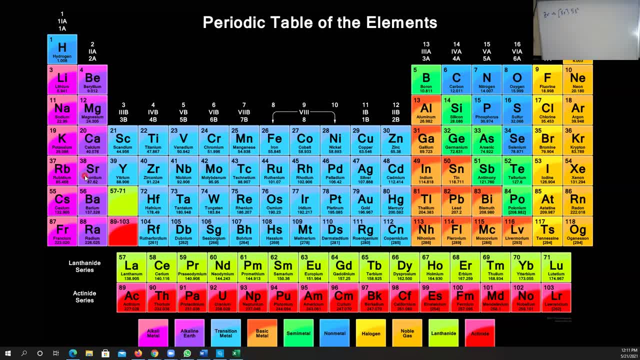 both of those 5s electrons are going to be used. Zirconium is only 2 into our 4d block, So I'm going to have a an electron configuration that ends with 4d2.. If I was ending with molybdenum, it would be. 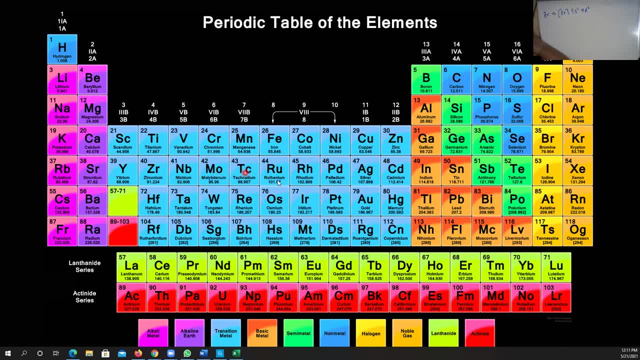 4,. well, let's not use molybdenum, because that's a little bit of an exception area. If I was ending with ruthenium, it would be 4d1,, 2,, 3,, 4,, 5, 6.. Okay, palladium would be 4d8.. 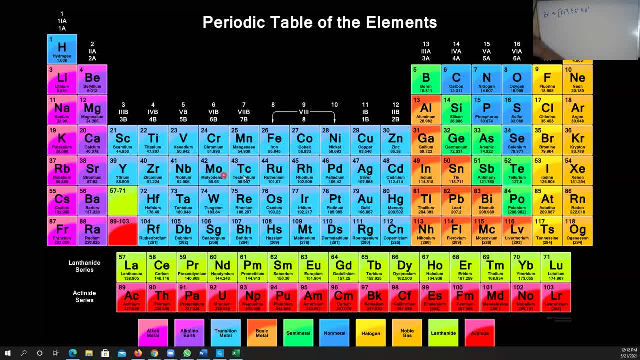 All right, so you, just you can count where we are on the periodic table and and there are some exceptions that we did cover back in chapter 8, having to do with half full sub-levels and full sub-levels- Right, so, like your chromium exception and your copper exception, 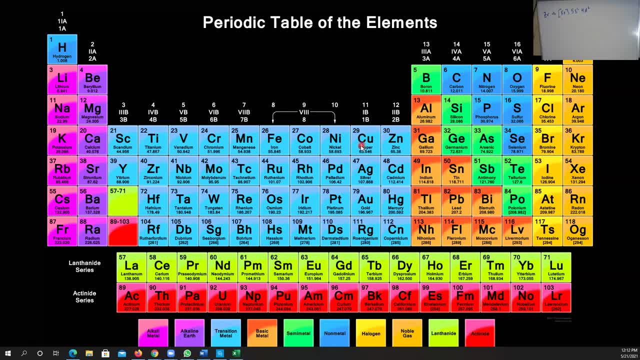 Those exceptions expand to more elements, but for the majority of them you can just count where they are on the periodic table to figure out how many d electrons are going to have. Okay, so our electron configuration for zirconium is kr 5s2, 4d2 and that's the neutral configuration. 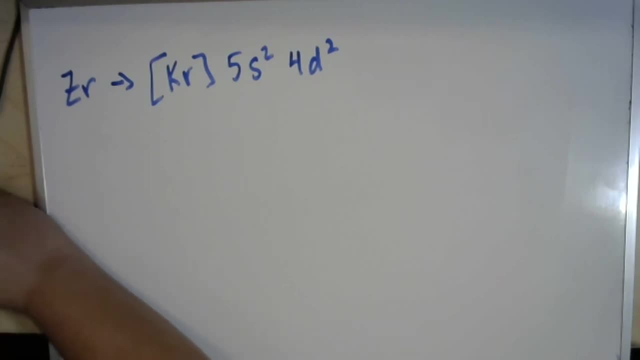 Okay, hopefully that makes sense. The second one. the second example was for osmium. Okay, so again, I would find osmium on the periodic table. it's number 76. I would go to the noble gas that precedes it, which means comes before it. 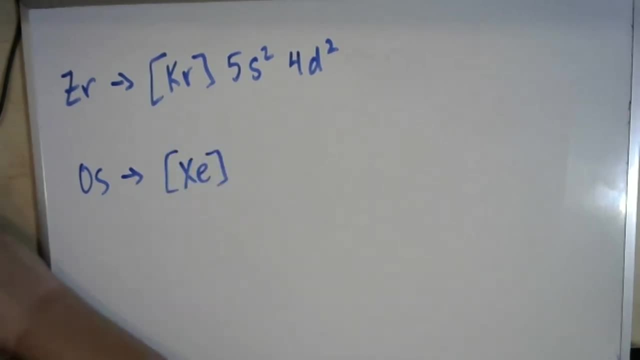 and that's going to be xenon. All right, then I'm going to use my periodic table to count all the electrons that are used until I get to osmium. Okay, so osmium is in the sixth row, which means I'm going to start with the 6s2 electrons. 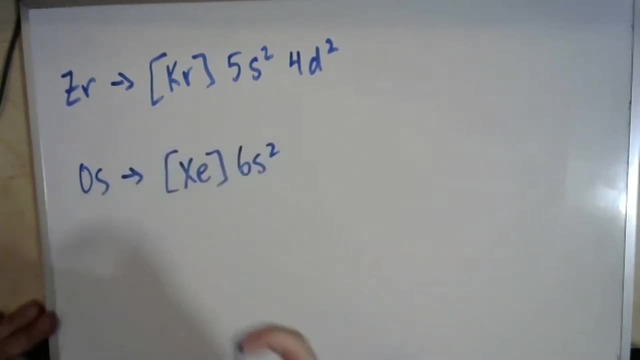 Okay, and then I'm going to run into my lanthanide series. Okay, before I get to the rest of my d block, I'm going to run into that lanthanide series. Let me just pop up that that share screen again to show you what I'm talking about. 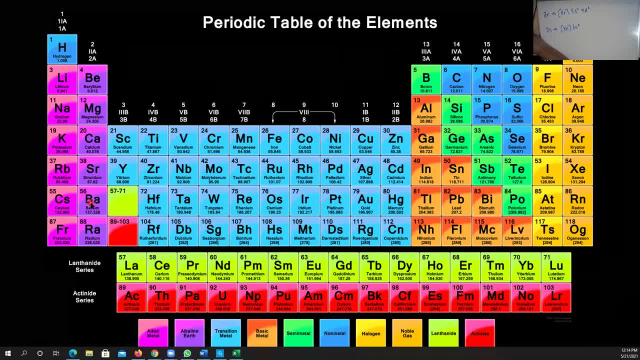 So I'm in my sixth row here and this is 6s2, But before I can get into my d electrons, I have to deal with the lanthanide series. Now, because I'm looking specifically at osmium. I know that I'm gonna be filling all of the electrons. 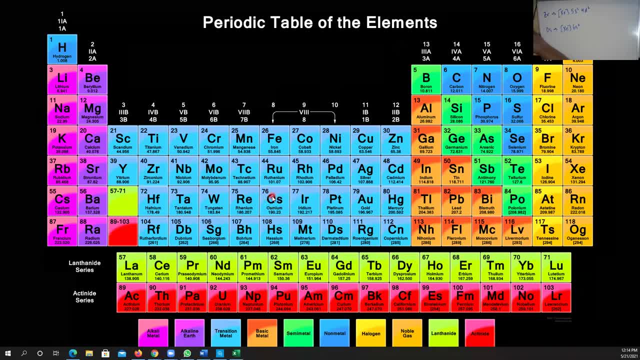 Now, because I'm looking specifically at osmium, I know that I'm gonna be filling all of the electrons. Now, because I'm looking specifically at osmium, I know that I'm going to be filling all of the electrodes, So I'm going to take 12 times more. let's justoperate and we can just. This is aniex solo. 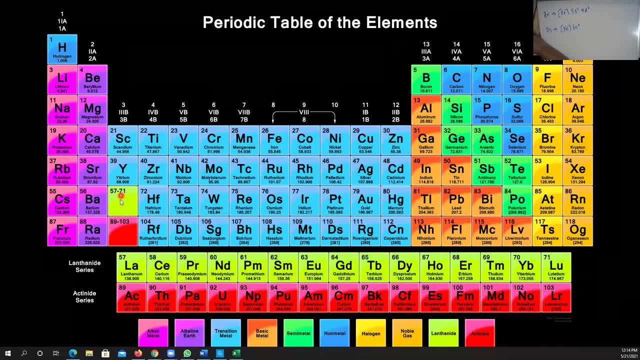 Let's justoperate and we can erkennen each electron late, all of the electrons in my f block here. okay, and your f block is going to be numerically two principal energy levels lower than your s block. so, because this is 6s, my f block is going to be in principal energy level 4.. 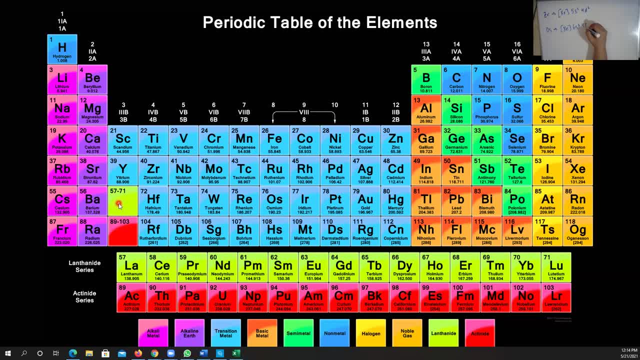 and i'm going to use all the electrons in principal energy level 4, so it's going to be 4f14. and then i'm going to use all the electrons in principal energy level 4 and that's going to be 5d. okay, after i'm done with my f block, i'm going to jump back up into the d. 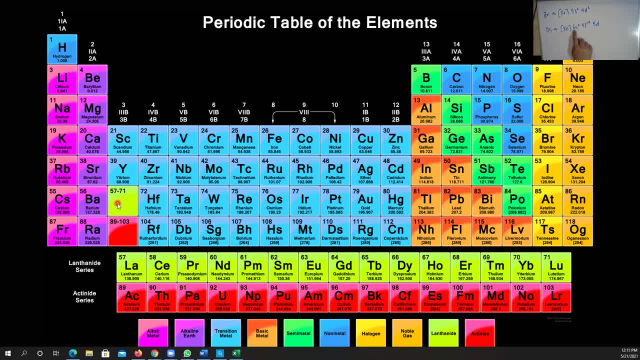 block and it's going to be 5d, because it's going to be one less than my my s sub-level value. okay, and then we can physically count over to osmium six. all right, so that's how we're going to write electron. neutral electron configurations. 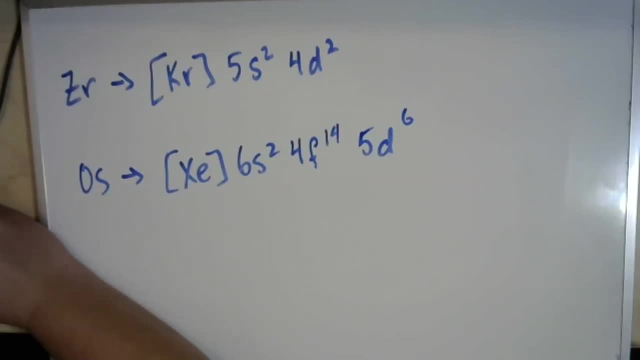 and we spent the time looking at this because we have to be able to write correct neutral configurations before we can write ion configurations, and the ion configurations are incredibly important to the stuff that we do in this chapter. okay, so the next example is asking us to look at ions instead. let me pull it up here. 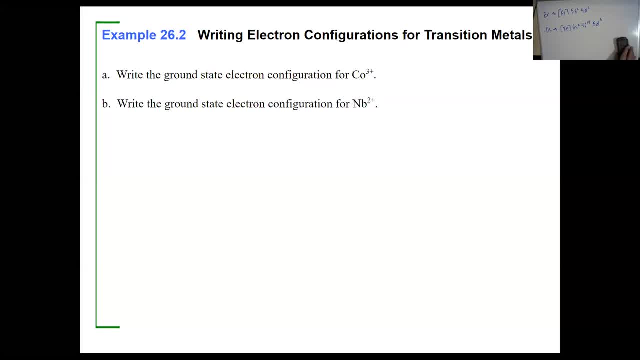 and we're going to look at co3 plus and nb2 plus, all right, so if you want, this would be a good time to just pause real quick and try them on your own and see, you know, give it, give it a shot, and then you can compare it to what i come up with. 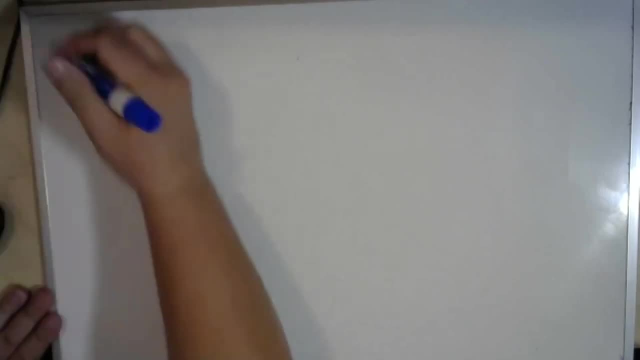 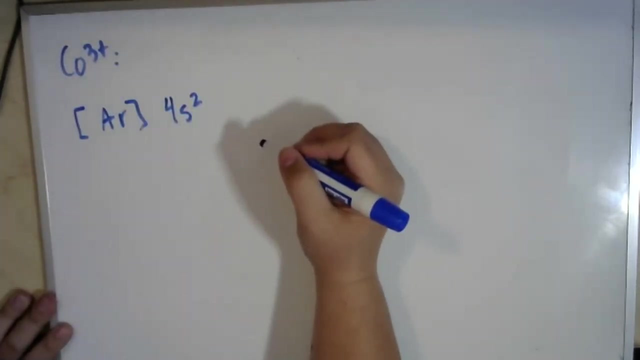 all right, but we're going to be doing co3 plus first, okay. so again, when i do this, i start out by writing the, the neutral configuration first, and cobalt is element 27.. so that's going to be ar, and then it's going to be 4s2, and then one, two, three, four. 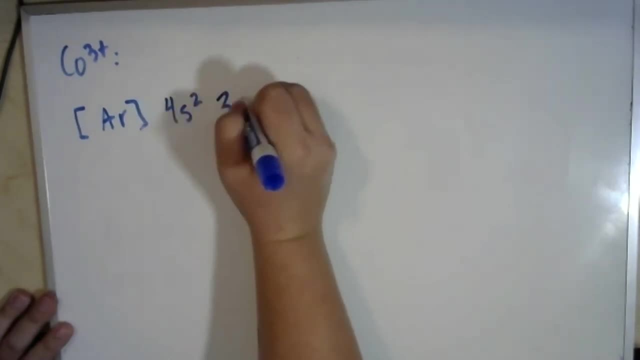 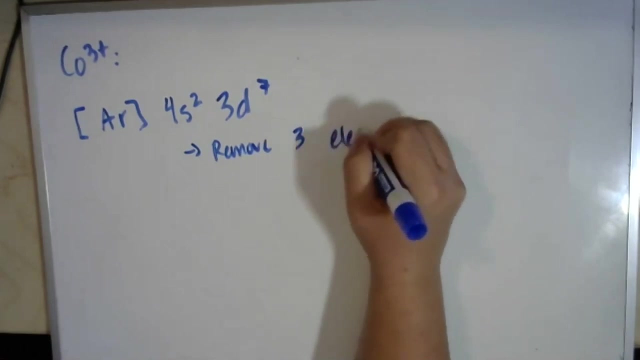 four, five, six, seven, three d, seven, all right. one, two, three, four, five, six, seven, okay. now if i want to turn this into cobalt, three plus, that means that i have to remove three electrons first, and then one, two, three, four, five, six, seven, okay, but you cannot remove any, just any electrons. 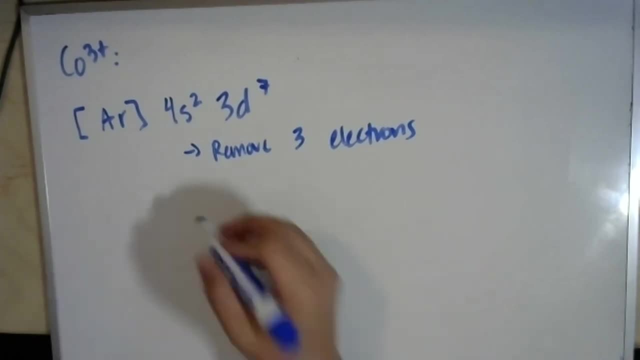 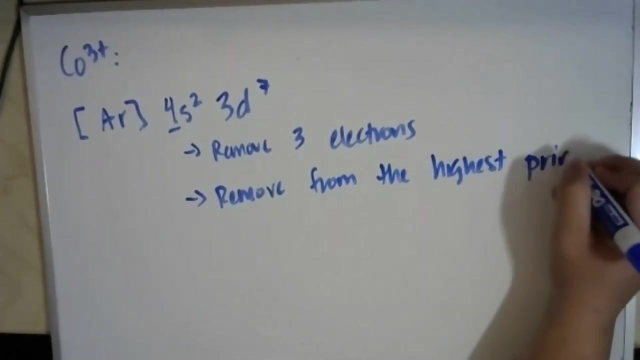 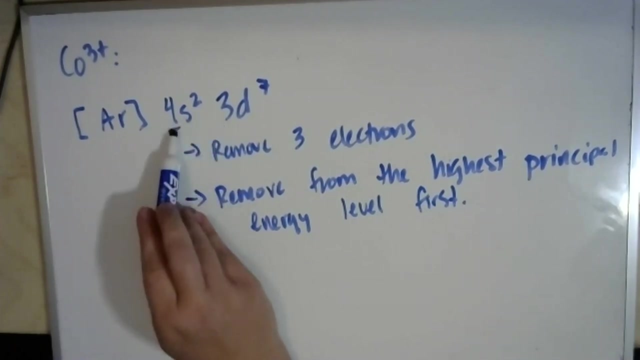 specifically here we have to start by removing electrons from the highest n level first. okay, so from the highest principal energy level. uh, i want to make sure that this is what it says. a, b, right. so if we look here, this is the um, the high ground that we've got. 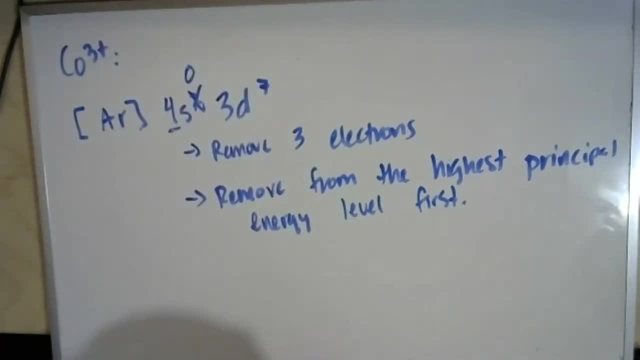 the fuel in the lake. septum reading. uh, that is really because there's zero, 0. okay, so we're going to remove that current leaving electron. we're going to remove the electrons to 0 configuration, for the cobalt three plus ion ends up being ar, and then you can. you don't have to. 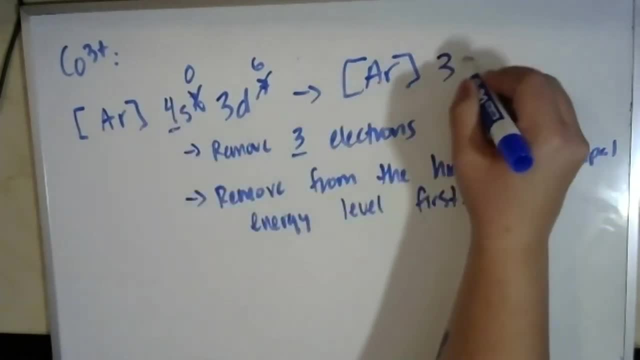 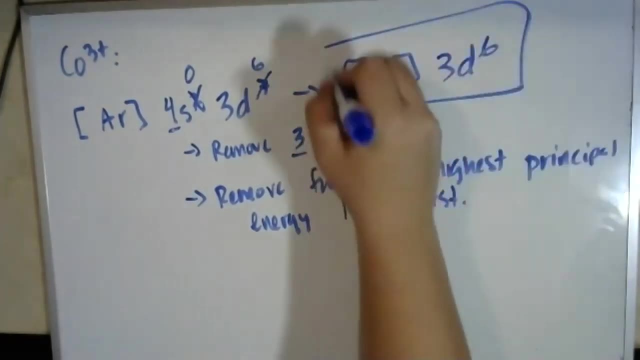 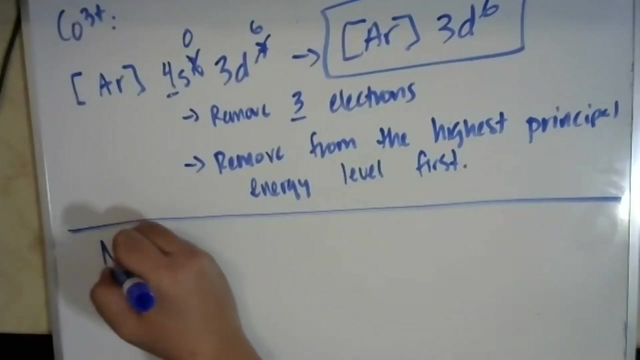 write four s zero. you can just skip that and you can write three d six. i mean, if you write four s zero, that's not a big deal, but this is what we end up with. all right, our next one is going to be nb two plus okay. so again, we're going to start by finding it on the periodic table. 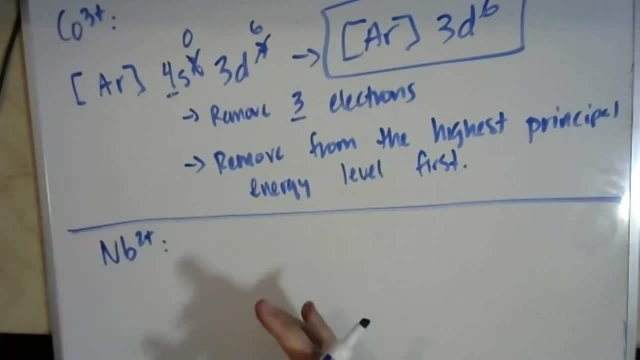 and then writing out the ground state structure. it's atomic number 41, so our noble gas that precedes it is going to be krypton and we're going to be in the fifth principal energy level for our s's, so it'll be 5s2. 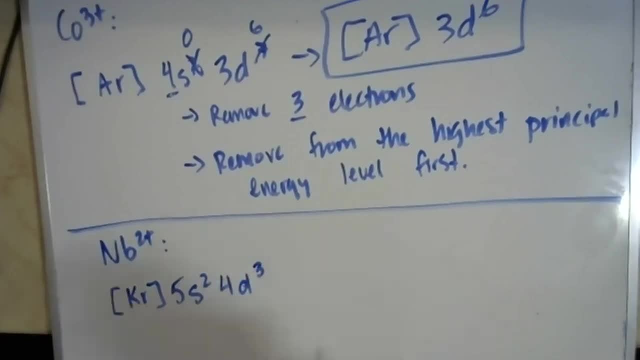 4d3. okay, and again to turn this into an ion. now i'm going to focus on the highest principal energy level first, not what i wrote last, what the highest number is, and this is going to be a positive two. so i need to remove two electrons, and these will be the two electrons that i remove. 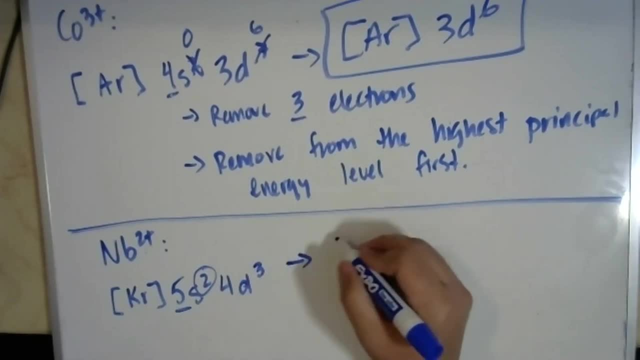 okay, so my electron configuration for nb2 plus is going to be kr 4d3. okay, so it changes. you know, making sure that you you're pulling electrons from the right place changes the value that you get over here, changes what your configuration of your ion is. 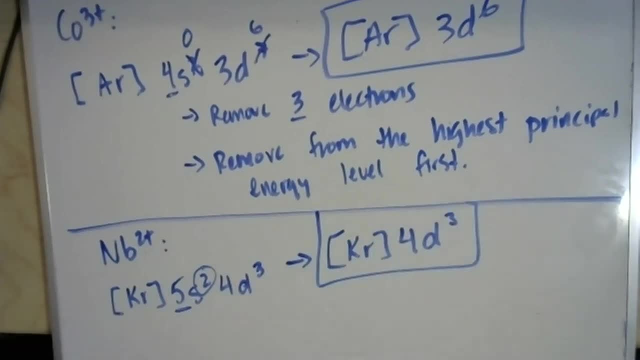 and that's going to be important later when you're deciding how many electrons are in your octahedral diagrams, right when you're looking at the magnetism. so it's very important to be able to to figure out how many electrons are in your octahedral diagrams right when you're looking at. 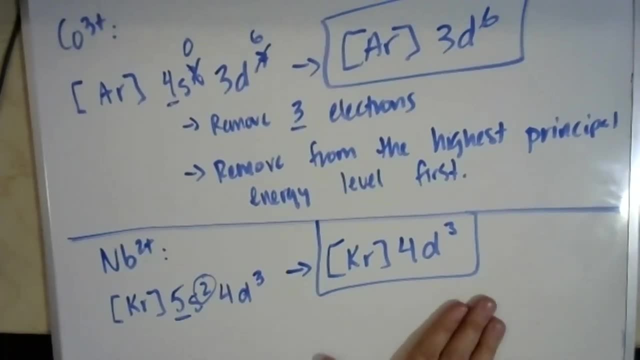 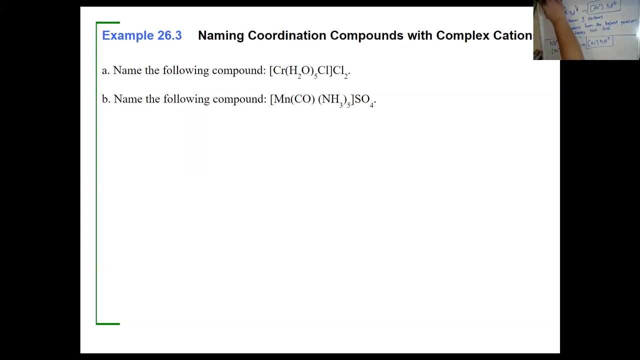 the correct electron configurations for these cations. all right, but a little bit of practice, it's not that bad. all right. our next question has to do with naming. okay, so we're gonna have to have a little discussion before we can talk about the naming, because i'm gonna blow through some stuff here and i don't want you to be like. 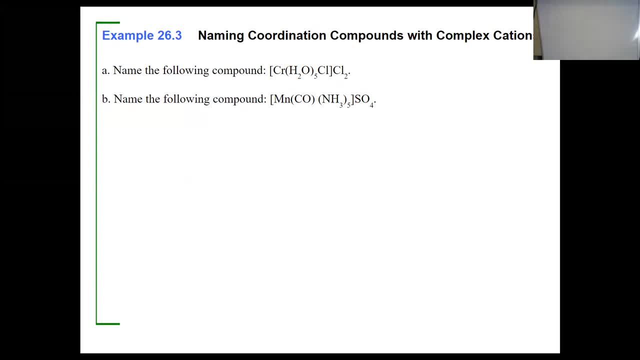 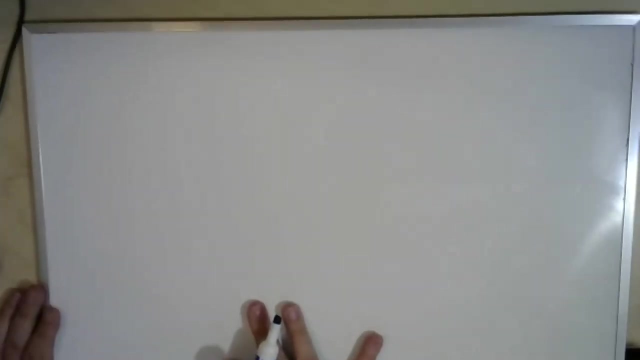 you know what are you talking about. when we're talking about coordination compounds, we're talking about a compound which is neutral, that's made up of at least one complex cation- maybe two, but at least one. okay, so you can write down these formulas real quick. when i want to go through a little bit of background, though, all right, 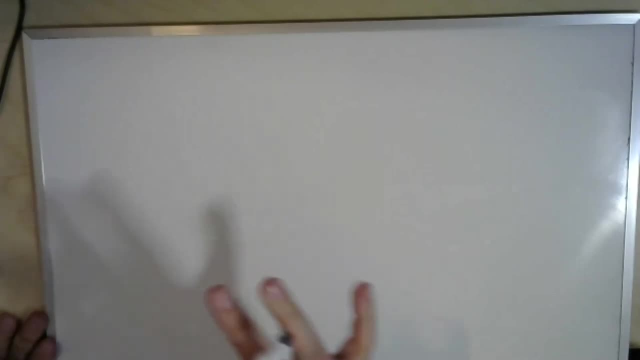 when you are looking to to name your coordination compounds. you have to understand that whatever is written first is going to be your cation and whatever is written second is going to be your anion. sometimes the cation is your complex ion. sometimes the anion is your complex ion. 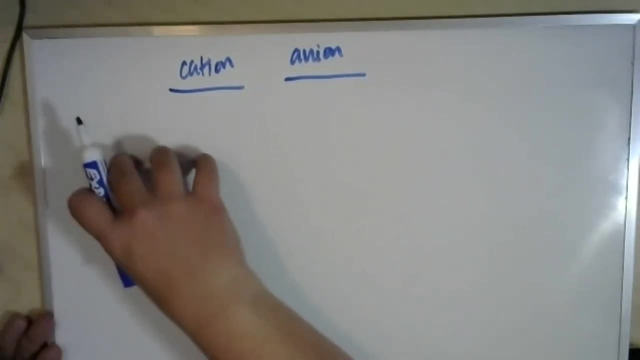 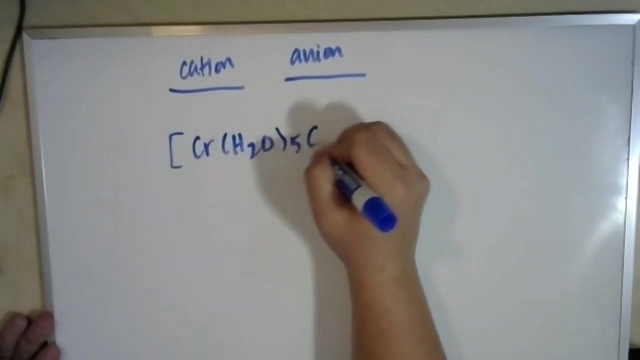 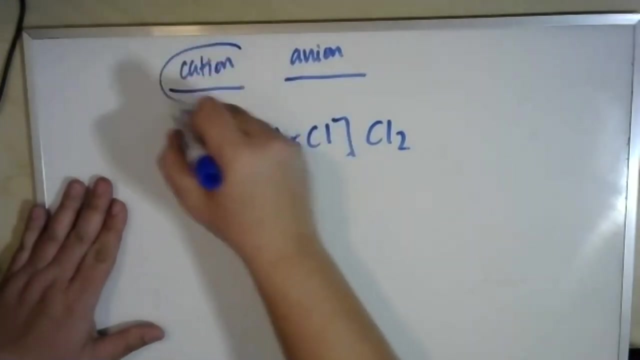 okay, and whether your complex ion is your cation or anion, changes how you name it. so one of the examples that we have here is cr. h205, clcl2. okay, the cation always comes first in a chemical formula. that means that this is a 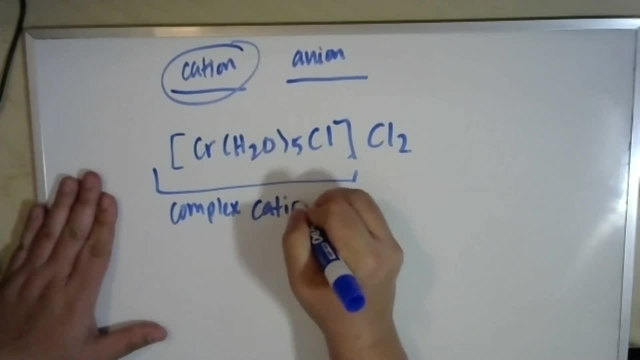 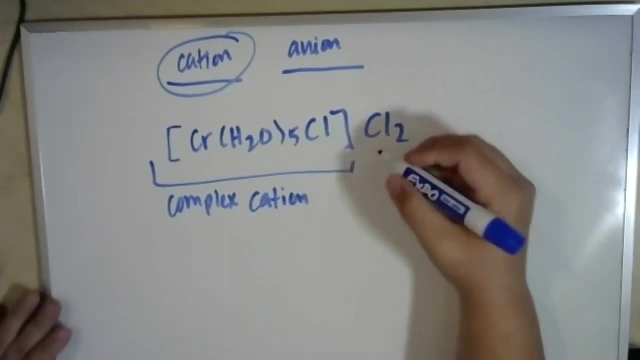 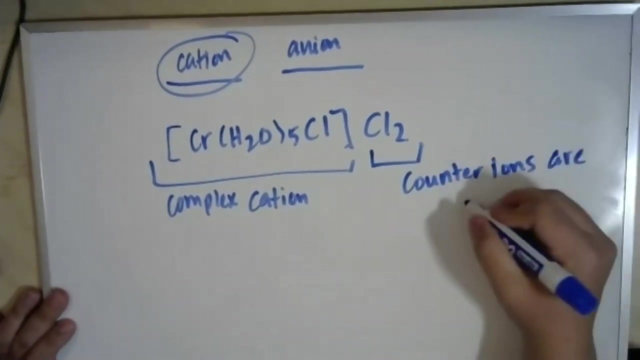 complex cat ion. you can tell it is a complex ion because it's in brackets. that's going to be your big hint there. and your counter ion? well, your counter ions are anions, and you know that they're anions because they come last in the chemical formula. okay, if you think all the way back to 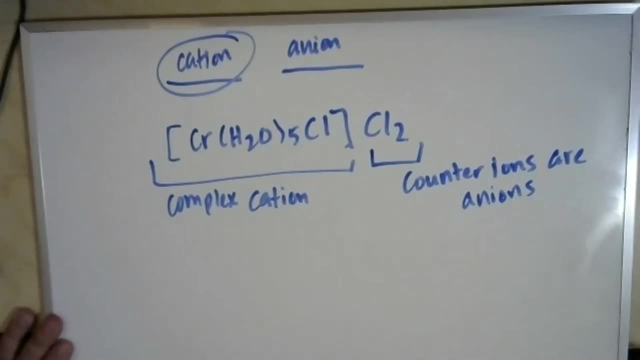 the beginning chapters, when we were first talking about chemical formulas. you should be comfortable with that idea by now, that your positive charges are listed first in your chemical formula and your negative charges come after. okay, now, in one of the next examples that we'll look at, you might 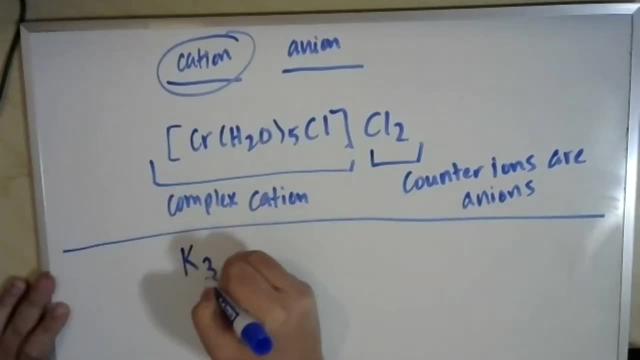 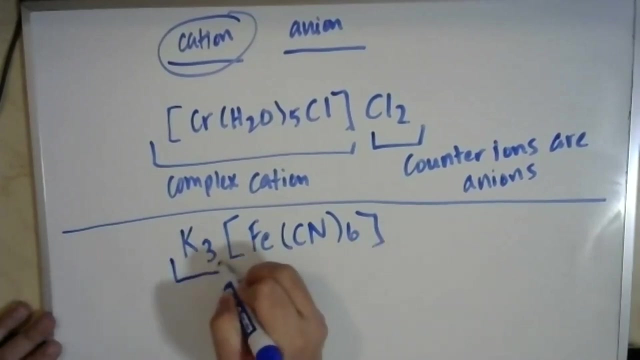 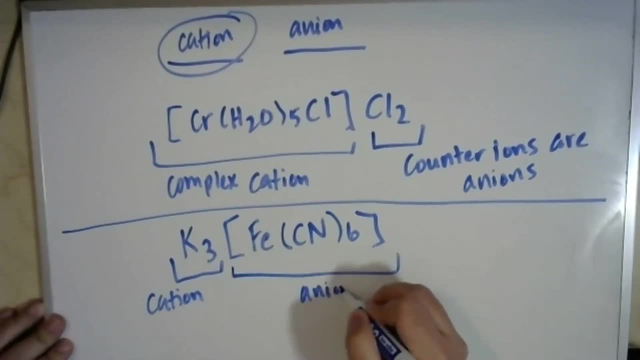 listed. second is your anion. okay, but this time the big guy in parentheses here is an anion, so we're going to call that a complex anion and your counter ions are cat ions in this one. all right, so when we're talking about the different rules for naming complex cat ions versus complex anions, 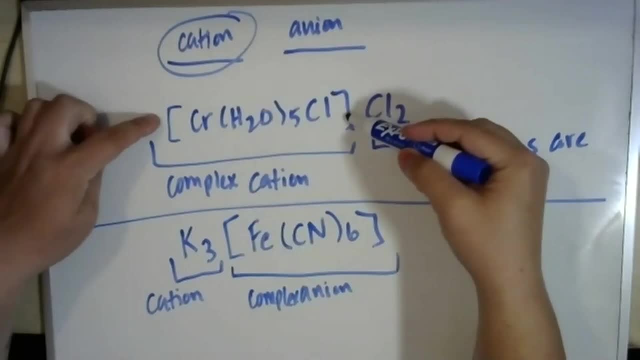 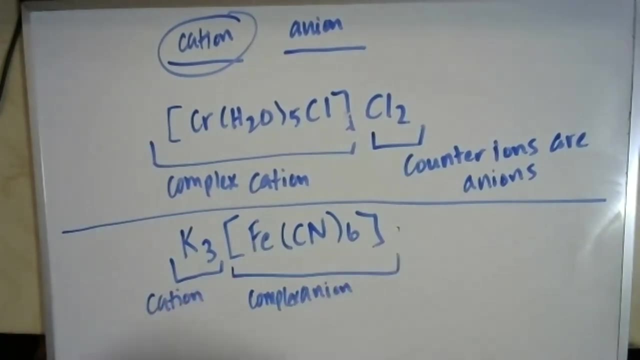 that has to do with whether your bracketed ion comes at the beginning of the chemical formula or at the end. okay, what's also true is that within your brackets, even if you have a complex anion, so overall here, an anion means that this is going to be have a negative charge overall. 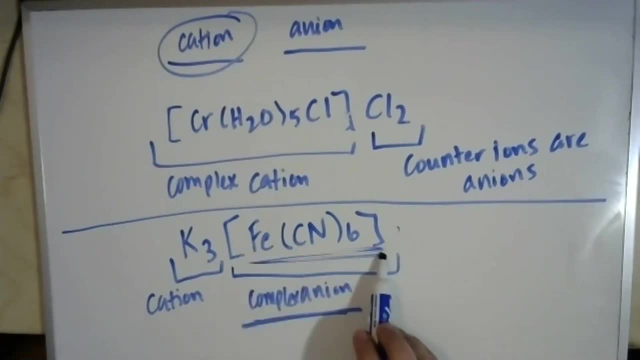 even though this ion has a negative charge overall, the charge on your metals are always going to be a positive charge, okay, like, if it's going to have a charge, it's going to be a positive one. your metals aren't going to have a negative charge, okay. so, even if the metal is part of a 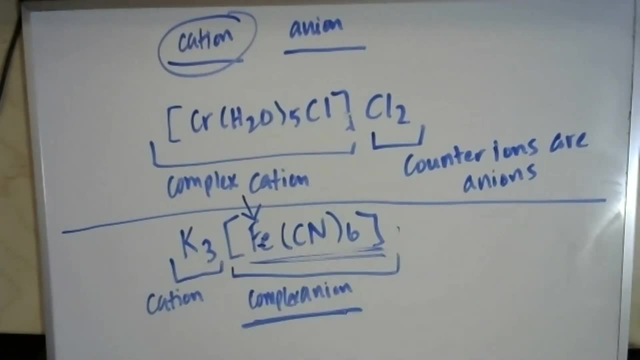 complex anion, the metal itself itself, is still going to have a positive charge, all right, um. so, that being said, let's move on to the next one and we're going to talk about the negative charge, all right, so let's look at. let's look at this. 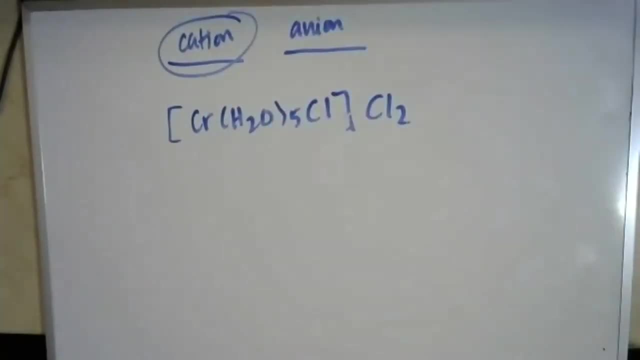 all right, so we're looking at this, this compound here, um, and your textbook goes through steps and i think that they're good steps. um, for naming these, they tell you first of all to look at the ligands and to just name the ligands. okay, so when you see h2o, which is water, the name of that particular ligand. 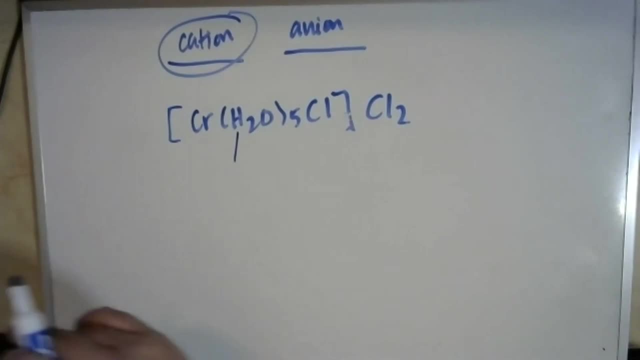 is going to be aqua, right? you have to know the proper name. you can't just write water in there. okay, the name for the chloride ion is going to be chloro, right, and you want to put these in alphabetical order? i would put them in alphabetical order. 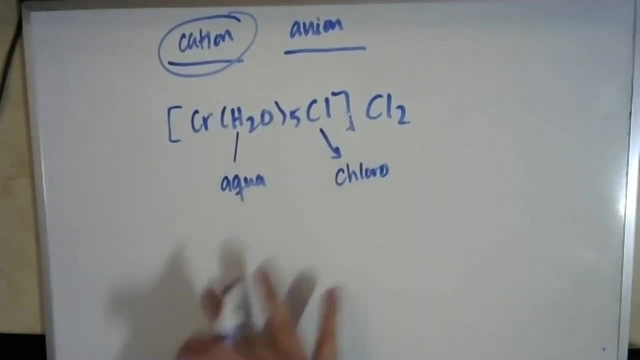 before you look at any of the subscripts and you try to like put prefixes on there, because the prefixes are not included in the alphabetizing. so a lot of times it's easier, before you even look at this five. just to make sure that these two things are in alphabetical order. 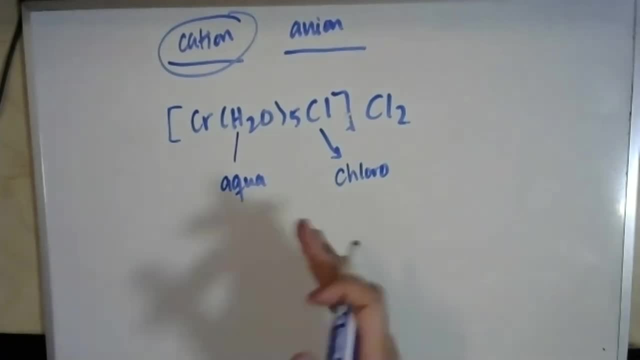 and they are right now, because a comes before c. now, that that's true. now they like, now that you've got that all set and you're like, yeah, that that's correct, now you can look at that five and you can put a prefix in front of the water. okay, so now you can call that penta aqua. 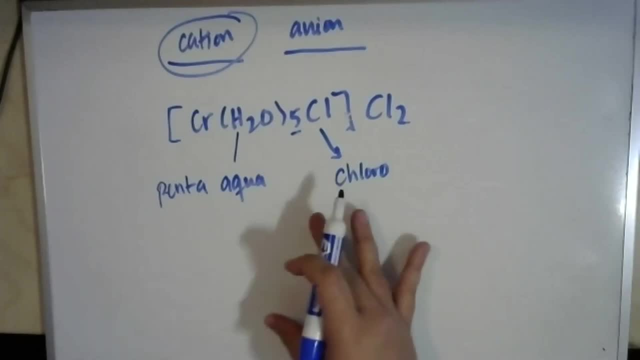 and also fix this up a little bit later. This is just how I go through and make my notes when I'm doing this. okay, The next thing that we have to do is we have to figure out what the charge or the oxidation state of the metal is, that's in the complex ion, okay, And we have to use all of the information. 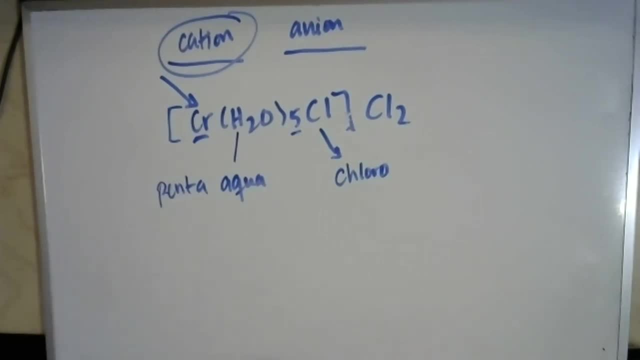 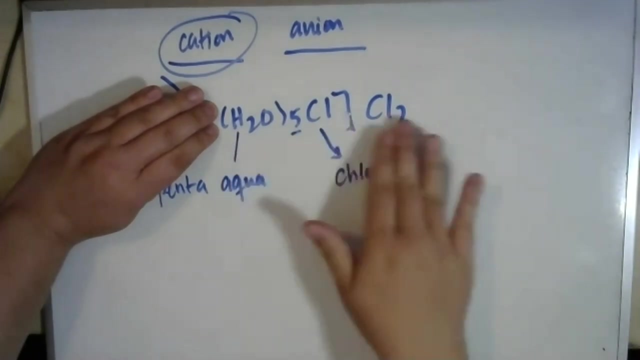 that's in that formula to help us out there. So what you're going to do is you're going to go through and you're going to assign charges to everything in this coordination compound except the central metal, And you're going to use all of this information to figure out what the 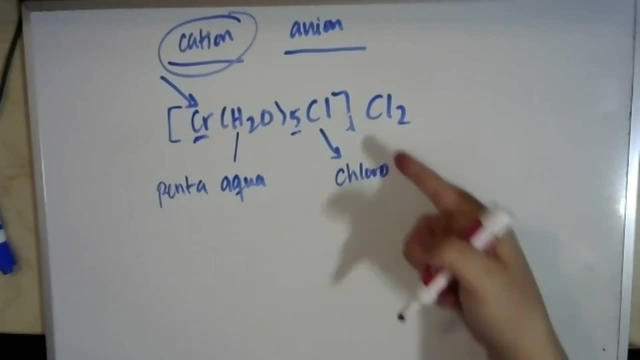 charge is on this, okay. So, for example, you know that every chloride ion has a negative one charge. right, And all together we have one, two, three chloride ions here. So then the chlorides are giving us a total of negative three. 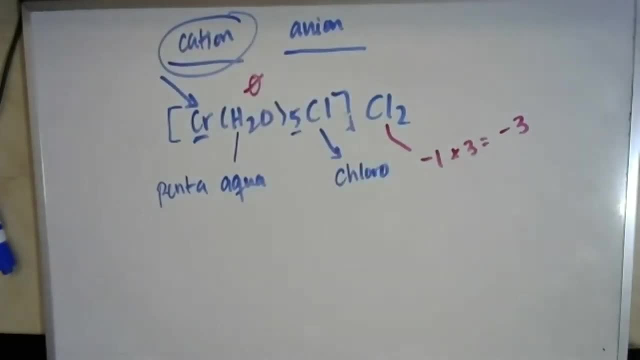 Water has no charge. got a charge of zero. So the other thing that we have to be aware of- and it's worth mentioning, because I did have a question about this- when we're looking at a coordination compound, meaning that there's a 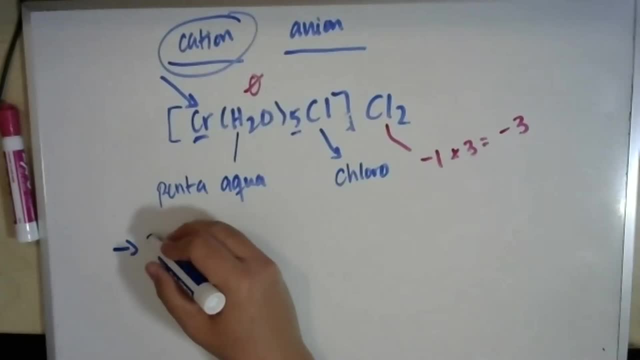 cation and an anion present. all compounds. all compounds are neutral, Okay, So they have no charge on them. That means that when we add up the charges of everything in this compound, it should add to zero. So that means that. 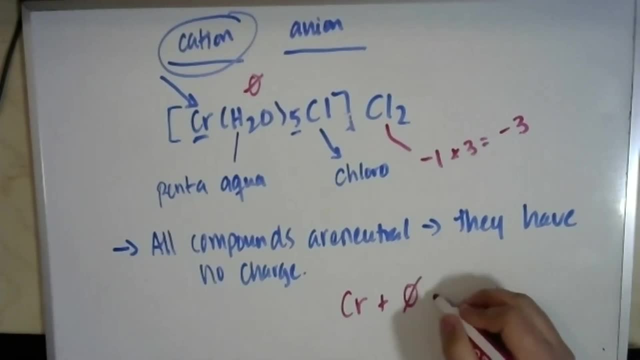 my chromium ion plus the water, plus the three chloride ions needs to equal zero, And what that means is that my chromium ion has a charge of positive three or an oxidation state of positive three. Okay, so using that method, we just figured out what the charge on the chromium is, and we need this charge as part of the name. 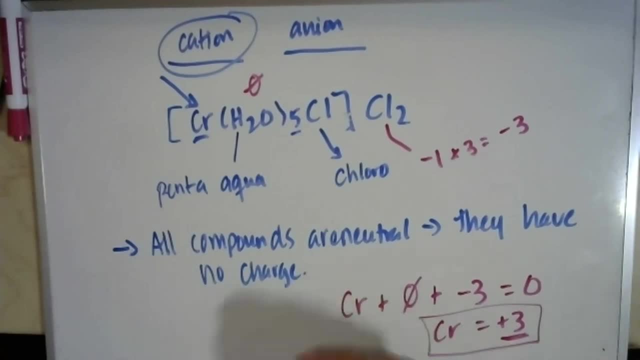 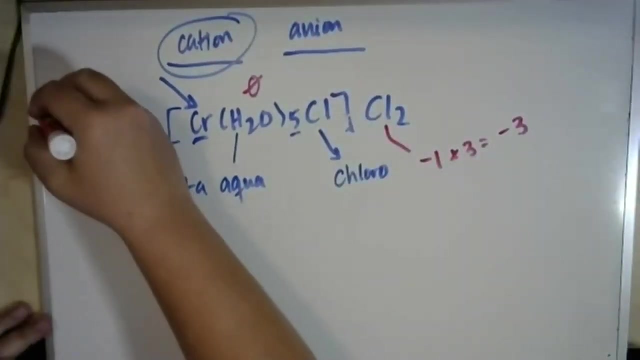 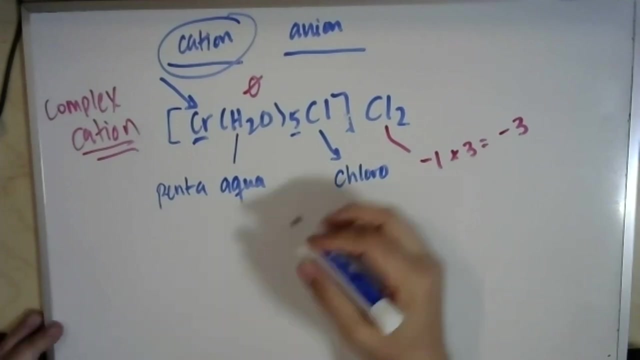 Because you have to name the charge along with the metal for these. Okay, so this is going to be chromium three, and notice that because my complex ion here is a complex cation, I'm not going to change the suffix of the, the ending of the metal, I'm just going to call it. 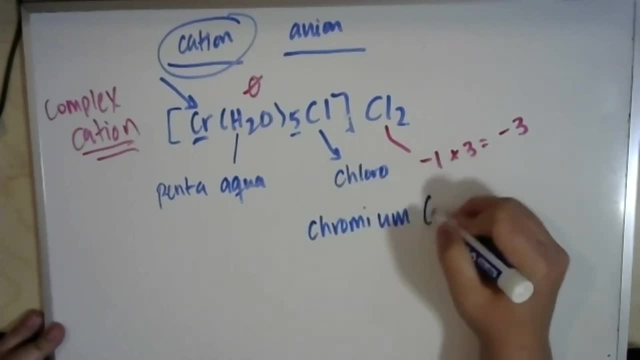 chromium and then a three in roman numerals. Okay, so now we're going to put this together and we're going to form the name. Like all compounds, you're going to name the cation first, the anion second, and if you're ever confused about that, bring it back to something that you know. 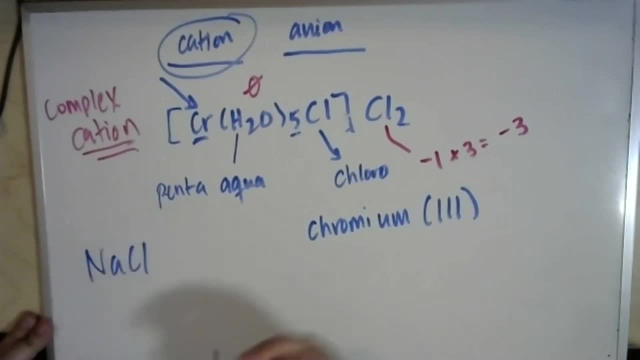 It'll be just like if you were naming NaCl: You name the cation first and the anion second. It's an ion, an ion second, Something that is similar to the Para lead, which is this: feminist arrived. you can't K. anion tier. You name the cation first. We're going to get rid of the NaCl here in just a little bit. All right, so this cation is also an added toxicIVE. So we already have our ligands. in alphabetical order, We're going to put eight. 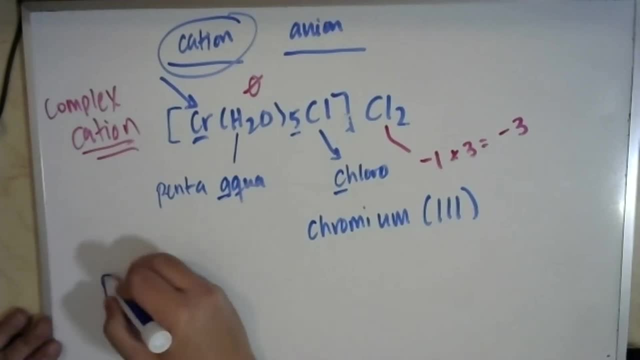 first, c second, so it'll be penta aqua. there's only one chlorine, so i can just write chloro. this is chromium three. and now i've named the cation. and now i'm just going to finish it up by naming the anion, and you don't have to do anything special to name the anion. it's. 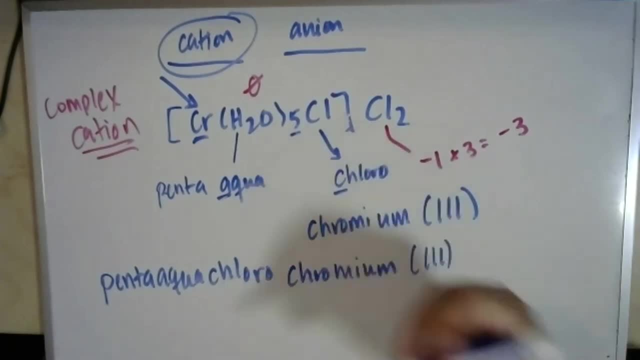 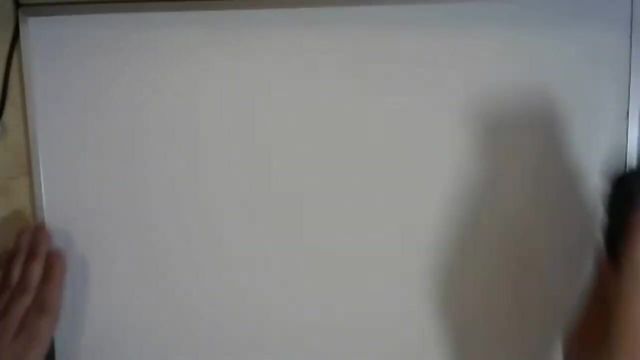 the same again, as if you were naming like nacl. so if you have two chlorines attached back here, that's just going to be chloride penta aqua chloro, chromium 3 chloride, all right, okay, let's look at the next example. it's going to be another cation, just so we can get another bit of practice with that. 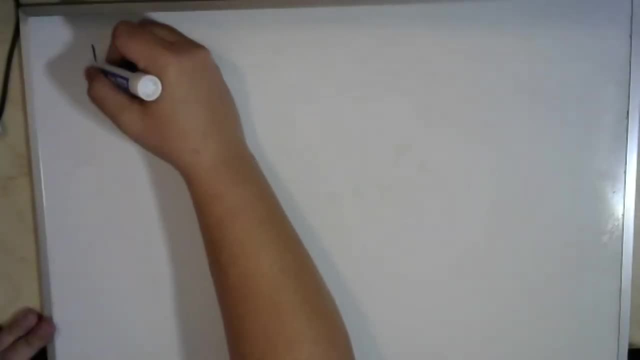 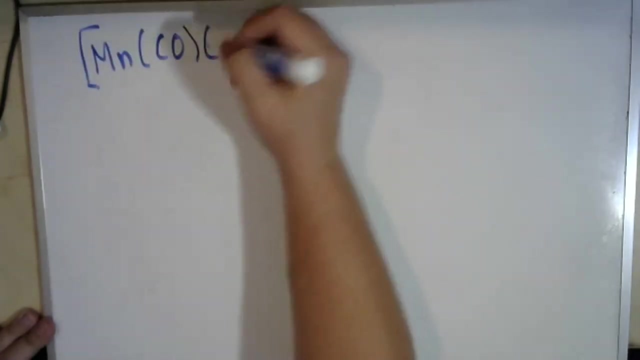 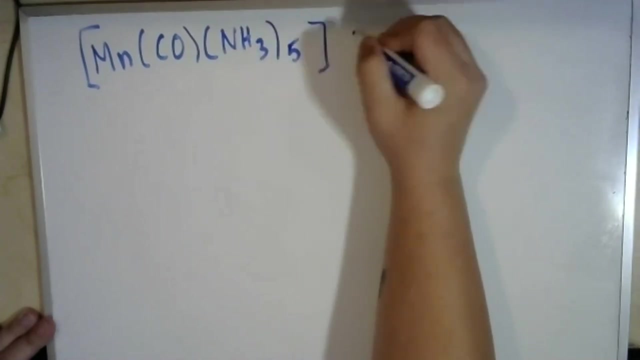 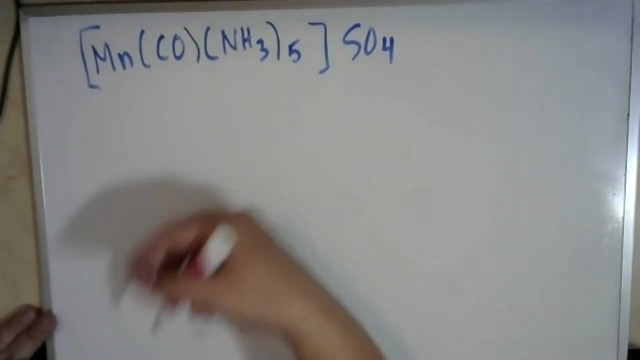 so, so okay, um, so again, you can maybe. maybe you can start by: uh, you could either start by listing out the ligands, like we did before, or you can find the charge first. whatever makes you happy. i like this naming the ligands first, though, so we can pull out that co. we know that the name for that is going to be carbonyl. 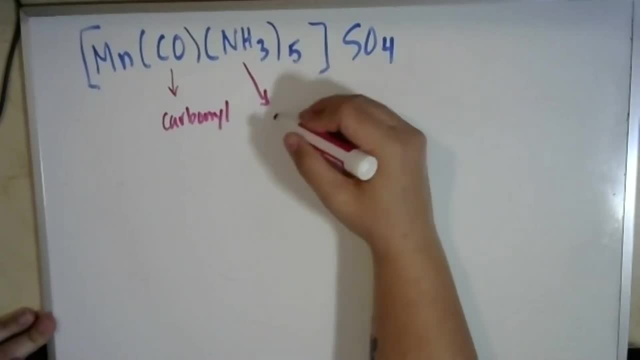 we know that the name for the ammonia is going to be amine, with two m's okay. so when we're putting these in alphabetical order, we know that the amine is going to have to go before the carbonyl, right, so we can put like a little arrow there. 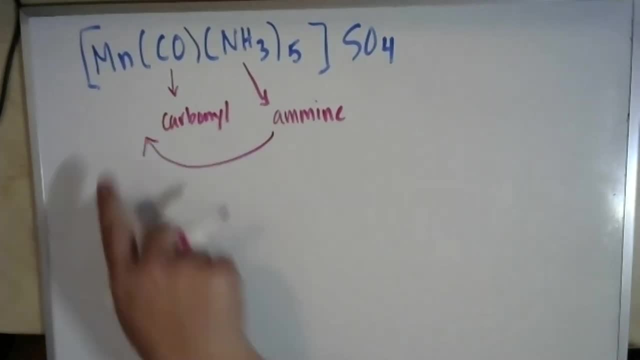 um, now to figure out what the charge is on our metal, we're going to look at the charges on everything else. okay, and we know that everything has to end up with a a with a neutral right. it's neutral, it has to end up with a zero charge overall. 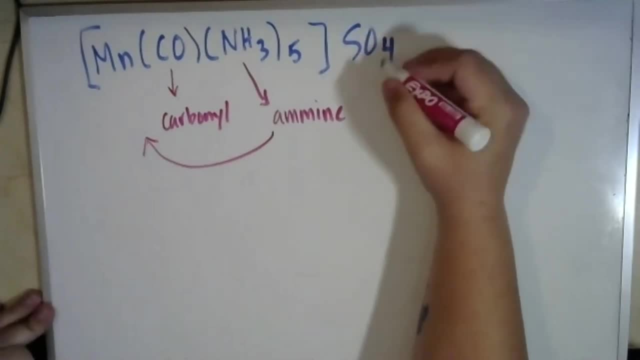 um, we know that the sulfate ion has a negative two charge. okay, and then you have to ask yourself: do any of my ligands have a charge? and in this case they don't. both of these liquid ligands have a zero charge. they're neutral. so we could put like little zeros here. 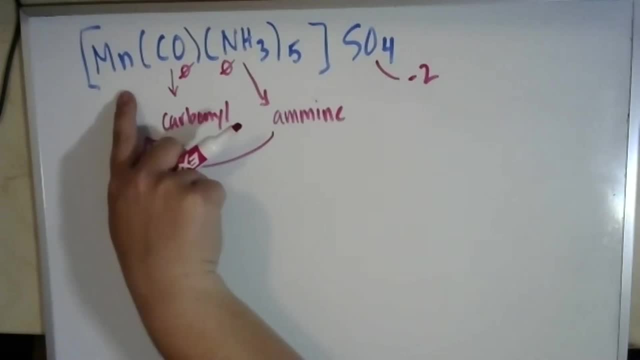 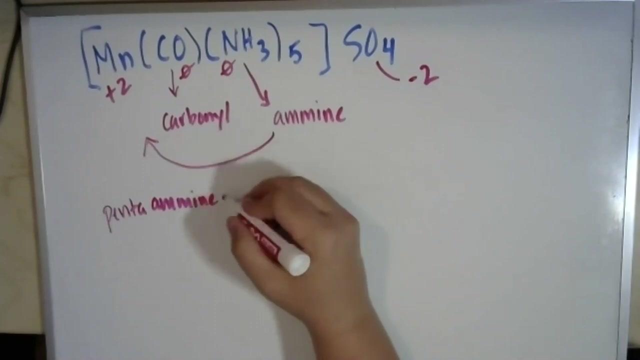 okay, so if my sulfate has a negative two charge, then my manganese has a positive two charge. all right, so that's going to be manganese two. so now i can name this. i have five amines, so that's going to be penta amine, and then i'm going to name the carbonyl. 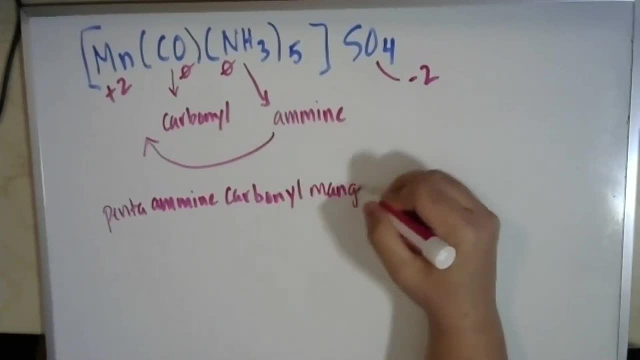 and then i'm going to name my metal including the charge, and i'll follow it with my oops, with my anion. okay, so now we can take a look at the complex anion naming so you can see how it's a little bit different, it's. 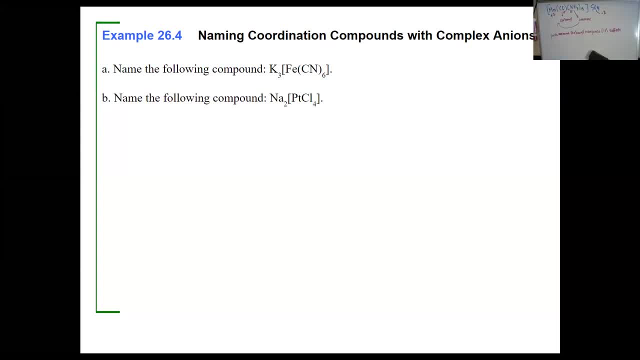 very small change. i mean, you're just going to be altering the very end of your metals for the complex anions. that's it, though the rest of this process is going to end up being the same. okay, so we have k3 brackets, fe, cn6, then we're going to have na2, pt. 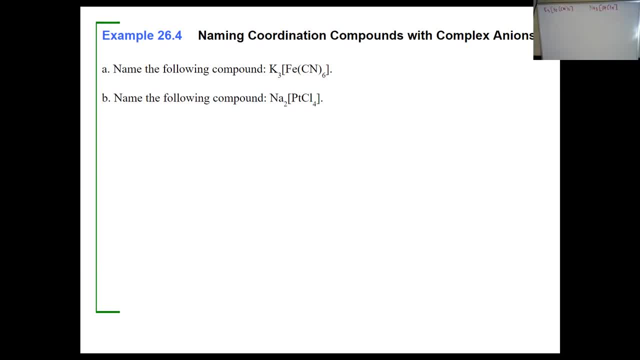 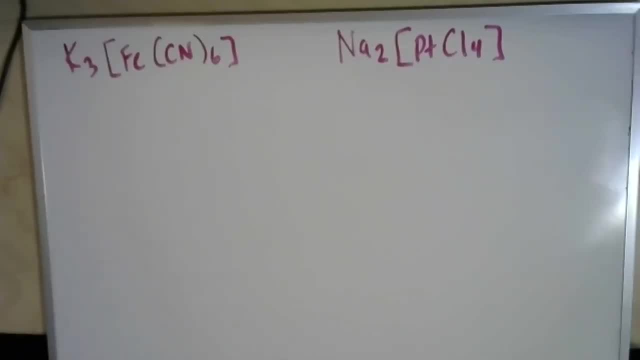 cl4. all right. so right off the bat again, we can tell that this is a complex anion because cations are first and ions are second, and when we have brackets around it like that, we know it's going to be a complex anion. all right, so we can start by naming our ligand. we have the cyanide ion in there. 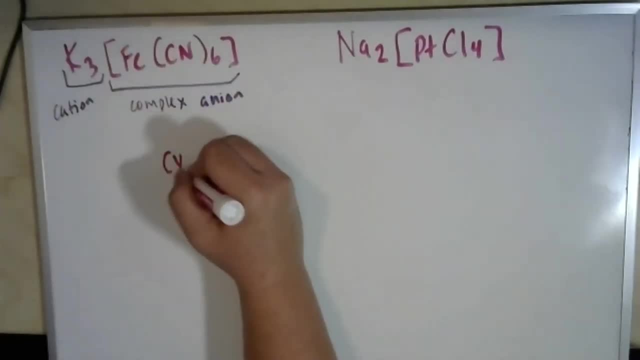 um, the name for that is going to be cyano, all right, and there's six of them, so we already there's only one type of ligand, so we don't have to worry about alphabetizing here. um, we do know that this is going to be hexa cyano when we're. 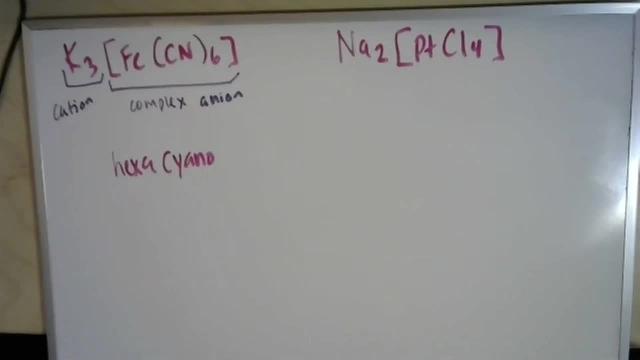 ready to to do that. but now we have to figure out what the charge is on our, on our essential metal in the complex ion, and we're going to do it the same way. okay, i know that we're in an anion here and sometimes that freaks people out a little bit, but you know you're going to go through the same process. we. 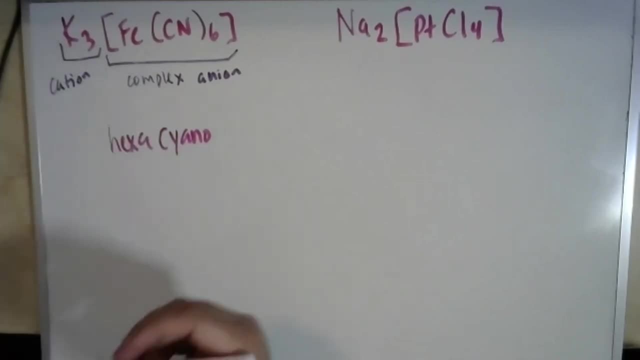 have three sodiums. if you look on your periodic table you see that sodium is a group of sodium. potassium: we have three potassiums. potassium is a group one metal. it has a positive one charge. okay, so we're going to do three times positive one means that you have a positive three charge from. 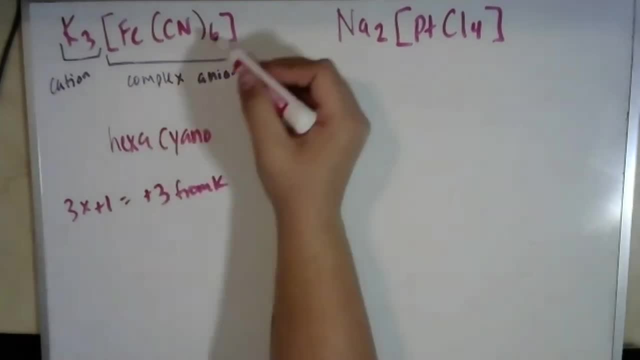 the potassium: okay, you have six cyanides. each cyanide, um. if you need a little reminder, cyanide is cn minus one, so each cyanide has a negative one charge. so we're going to have six times negative one which will be negative six from the cn minus. okay, so that leaves me with a negative three deficit. 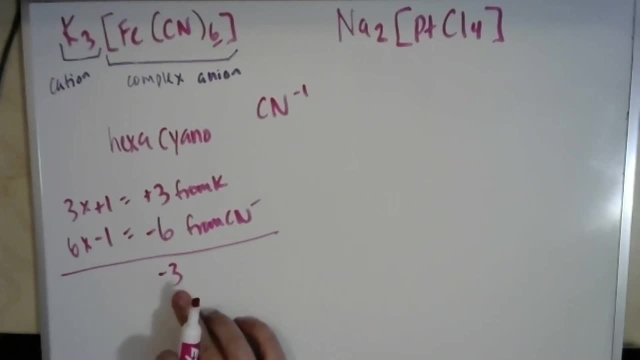 right now. that means that the charge on my iron is going to have to be positive three in order to make my compound neutral. all right now. the names for some of the metals change when we are working with complex anions instead of cations, which we talked about. 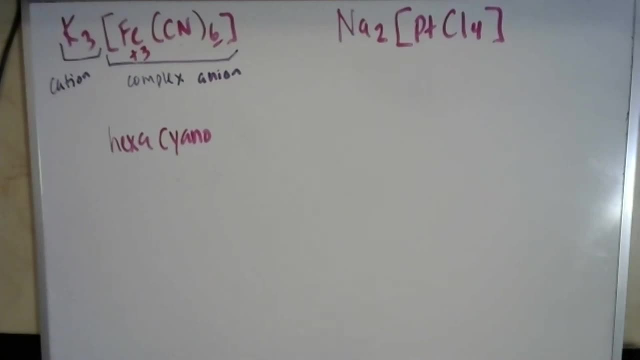 um. irons changes more than iron's name, changes more than most names, because instead of like just adding an a, t, e ending to iron, we have to change the name of it to ferrite okay. so we're kind of like doing a throwback to the older naming system with that. 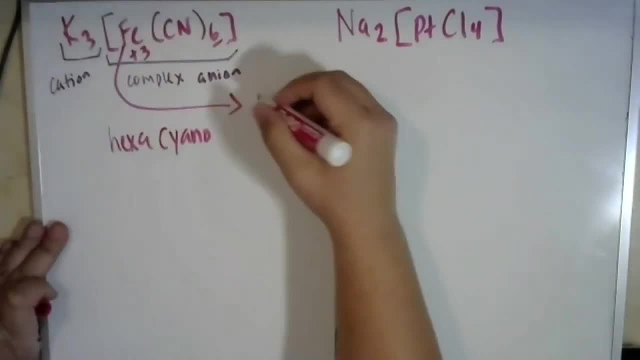 um, so we're going to call this the ferrite three ion, all right, but now we know everything, so we can name this, and we're going to start the naming with the cation, like we always do. we're always going to name our cation first. 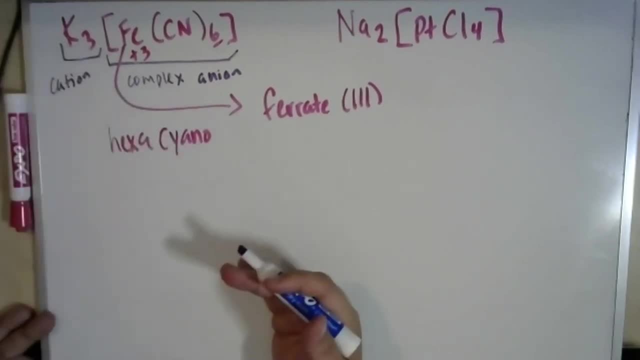 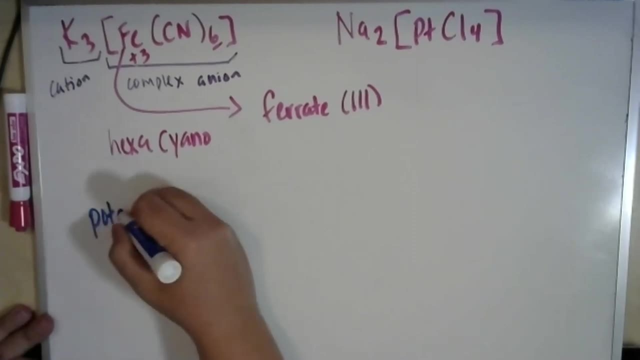 and this is a simple cation and just like any other ionic compound, even though there's three potassiums, we're just going to name it with the name of the metal, right? because when we have ionic compounds, um you know, if you have k2so4, for example, this is just going to be. 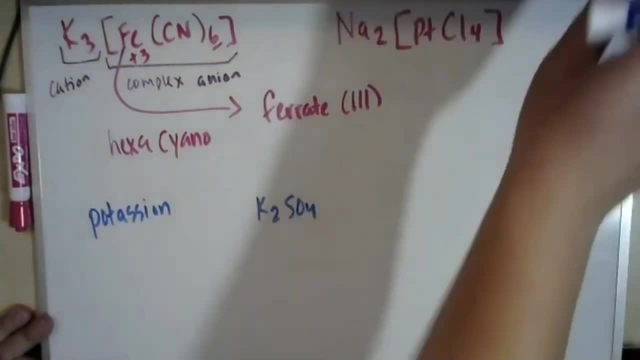 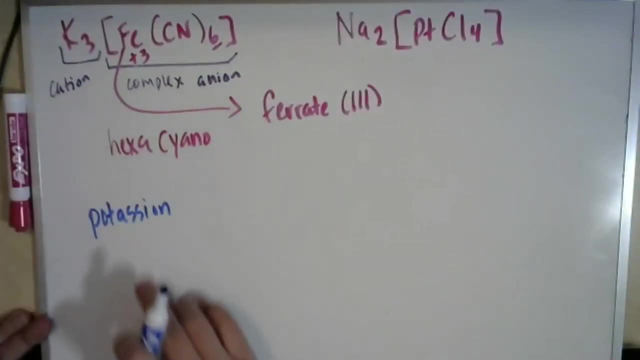 potassium sulfate. you don't have to tell us how many potassiums are there. we know how many potassiums are there based on the charges of everything. so we'll start by. we'll start by naming the, the metal, like the metal cation there, so it's potassium. 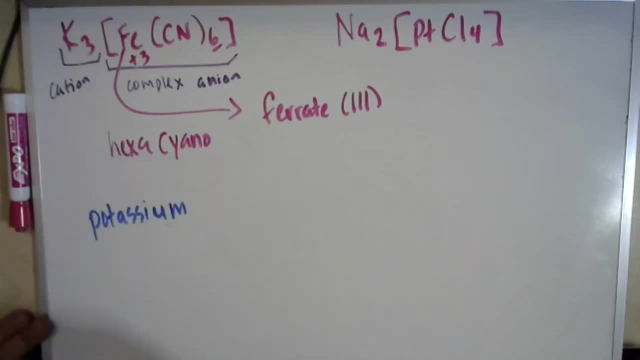 and then we can name our complex anion. okay, so that'll be hexa, cyano and then ferrite three. okay, and that's it. it's themed, all right. um, let's try this one, as we can go through and do the same thing. we only have one type of. 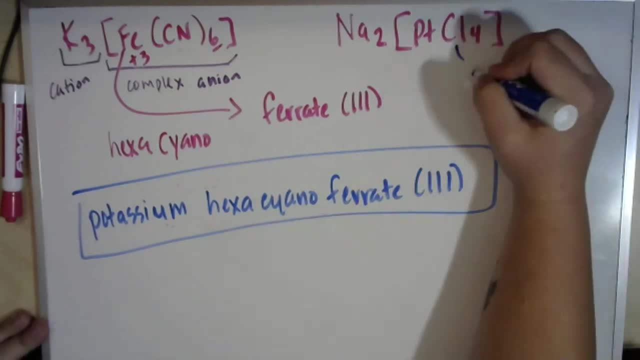 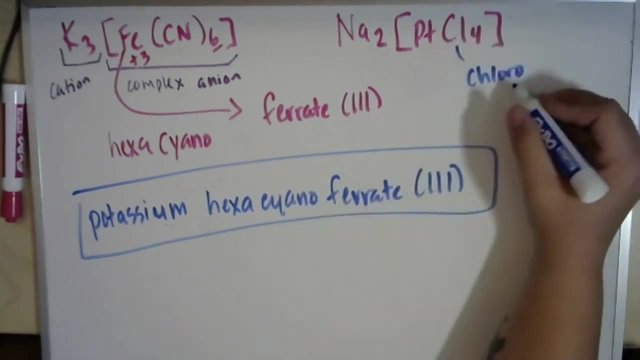 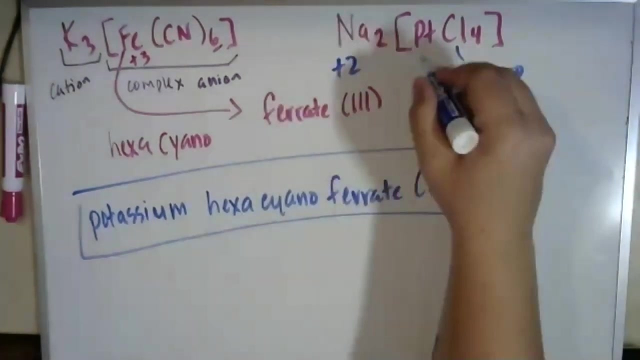 ligand. again here we just have the cl, which is chloro. all right as far as charges go. we have four chlorines, which is going to be negative four total. we have two sodiums, which will be a positive two total. that means that our platinum is. 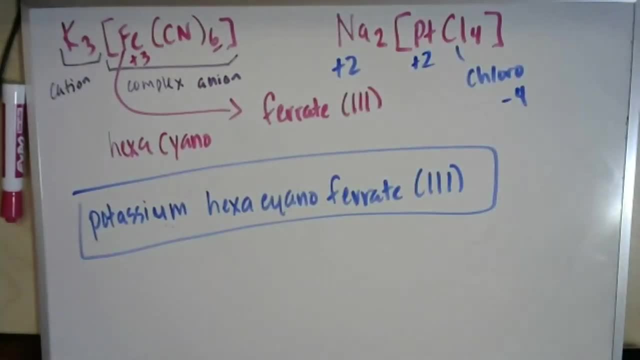 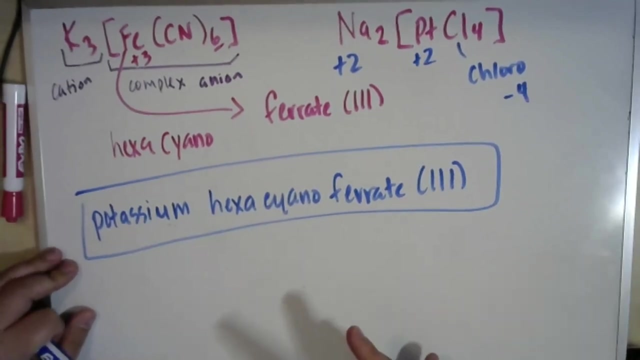 going to be a positive two, all right, um, while we're sitting here and we have both of these examples up, um, let's just take a minute to look at the coordinates. i want to turn this around to just give people so that everybody can see, like who knows? um, and that's in this. 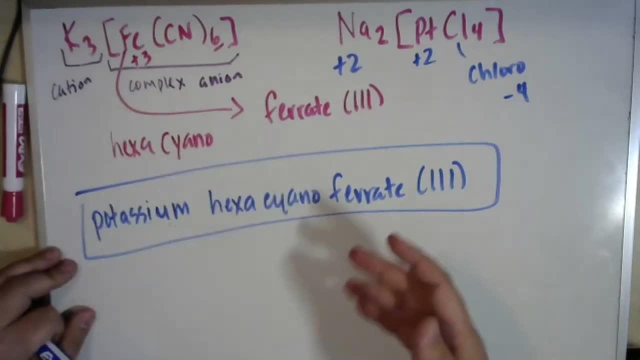 um or bidentate, meaning it has two lone pairs to contribute up to hexadentate, something like EDTA, which has six lone pairs to contribute. Once you know how many lone pairs the ligand has to contribute to the central metal, then you're able to look at the formula and figure out the 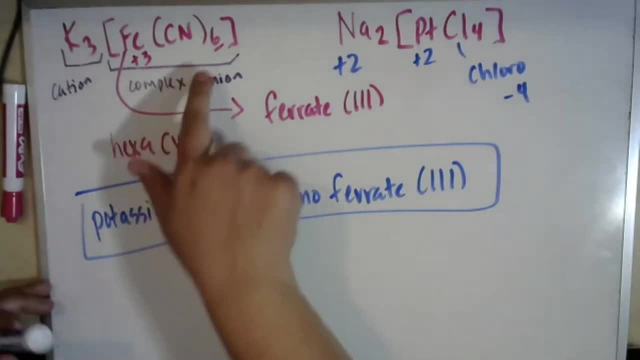 coordination number of that central metal. So for our first compound here we have six cyanide ions attached to that central metal. Cyanide is a monodentate ligand and that means that the coordination number- coordination number of that iron- is going to be six. 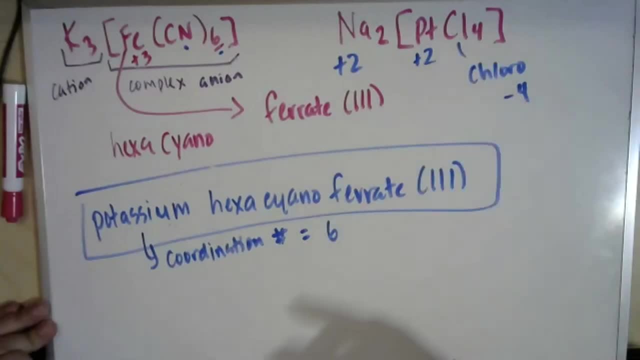 Okay, chlorine is also a monodentate ligand, so the coordination number of the platinum here is going to be four, because I have four chlorines attached to it. All right, I just wanted to point that out, I'll do. I'll do another coordination number count in the next question too, because 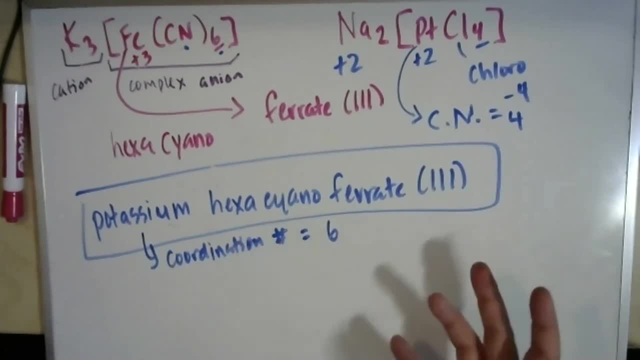 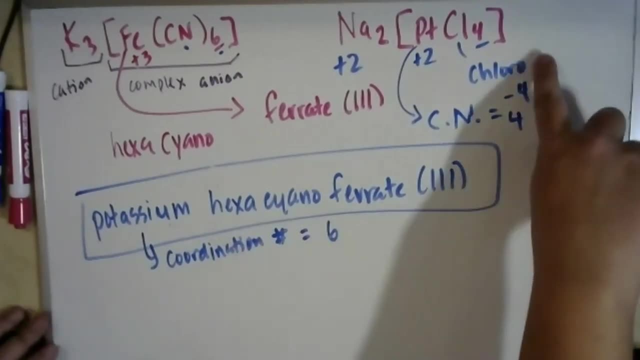 they don't. they don't actually have a question about finding coordination numbers in this list. that I was, that I'm going to be going through. All right, but back on track. We know what the charge is of our central metal. We know what the ligand is. Now we can name this. 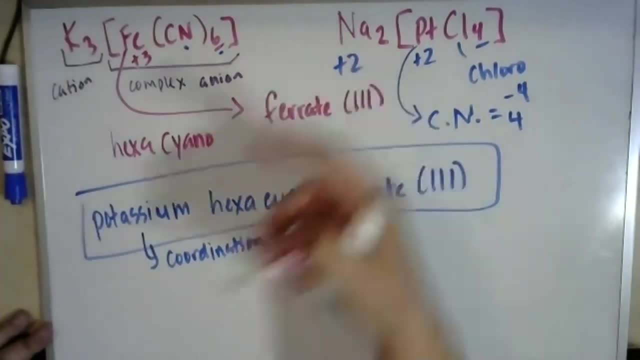 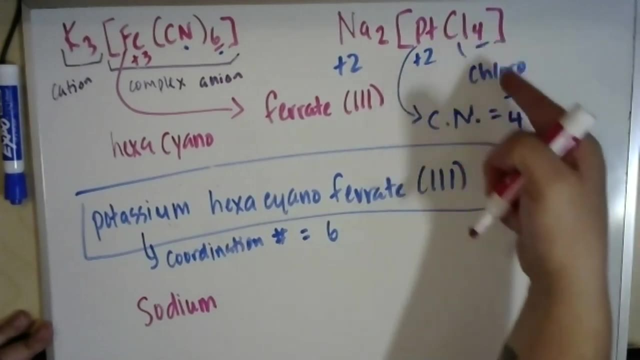 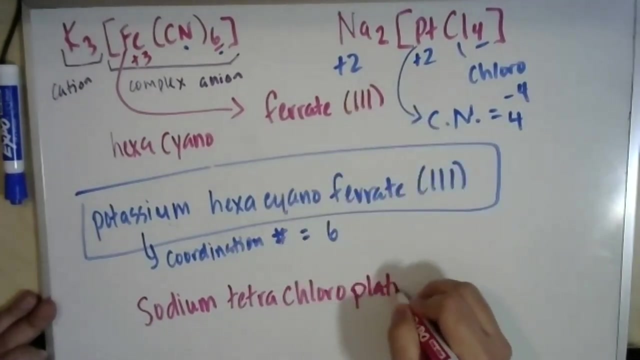 Okay, so we're going to start by naming the metal cation, here the sodium. Then we're going to name our ligand. There's four chlorines, so it'll be tetrachloro, And then we'll follow it by the name of the, the metal. So this one is going to be platinate. 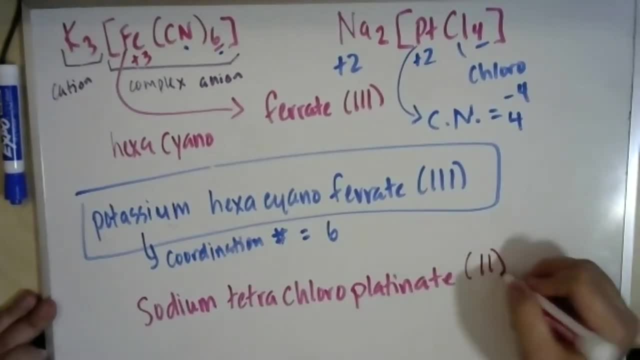 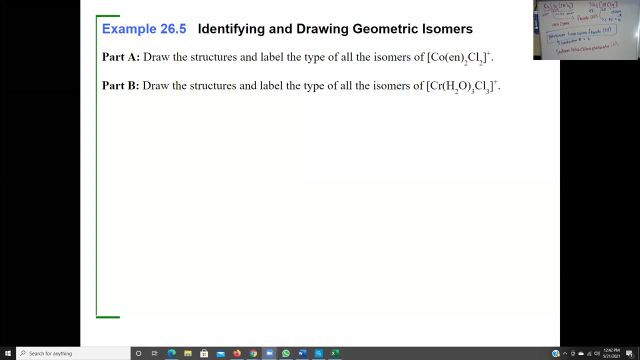 This is where we change that ending and we'll include the charge. All right, I think we'll. I think we'll name these ions too. I'll do it a little bit quicker for the next question, But before we look at the isomers here, 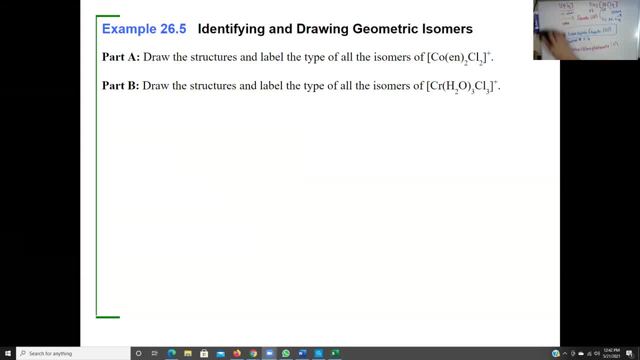 I think that we're going to to just name these, because at least we have some different ligands that they're introducing here that weren't introduced in the last one. So these are just complex ions and you can tell that something's a complex ion versus a coordination compound because it still has a 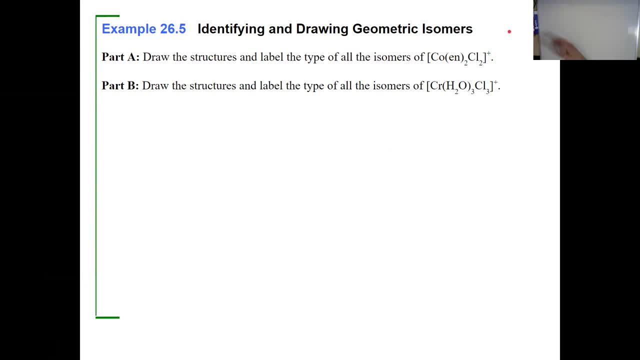 charge on it. Okay, So you can name the complex ions or you could name the full coordination compounds. You just you know, at the end you'd say ion if it's an ion. But let's look through, let's just name these real quick. 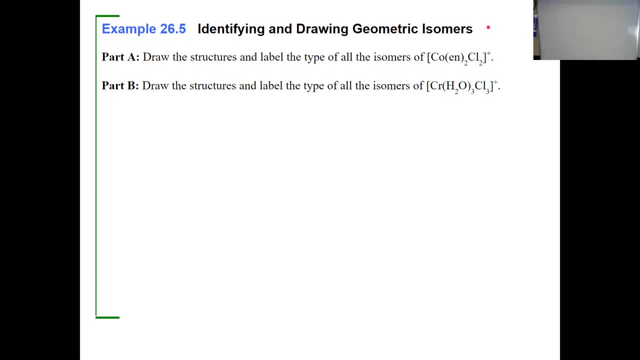 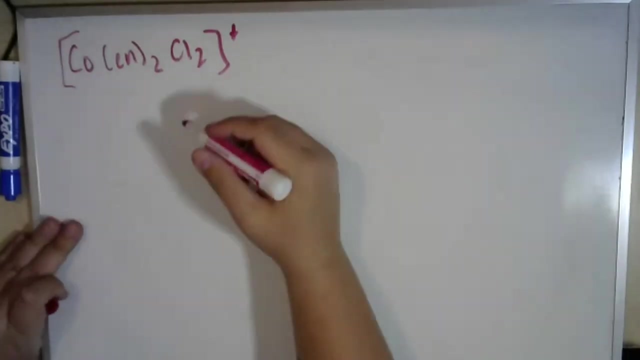 And then we can look at whether what types of isomers they form. All right, And I'll try to help. you see the trend there. So we have COen2Cl2+, All right, Okay. Okay, so over here we have. um, we have a complex cation. we know that because it is a positive one. charge. 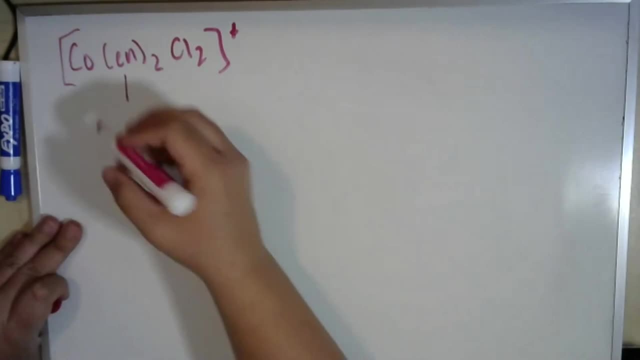 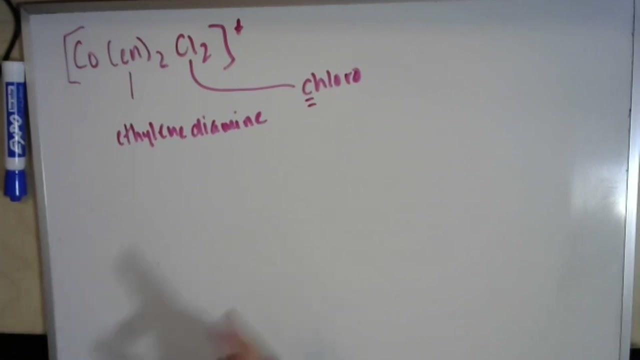 it's got two ligands, two types of ligands. it's got ethylene diamine and chloro. okay, so we're going to want to put that out front. i wanted to name this one, because the other examples don't include the other types of prefixes that you need to use when you run into this specific situation where you have the name. 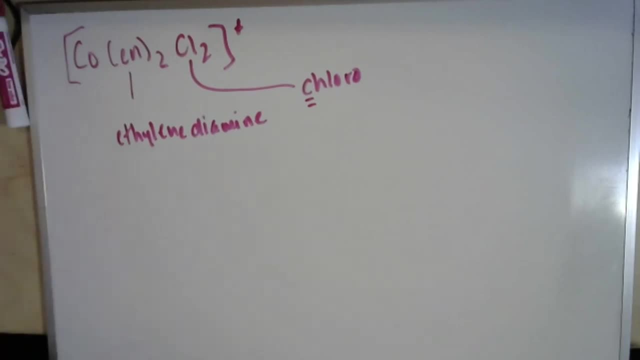 of one of your ligands and within the name itself there's a prefix: okay, it only happens for your list of ligands with ethylene diamine and then the ethylene diamine tetra acetate, the edta. the rest of them are going to be normal, but for your ethylene diamine in your edta. 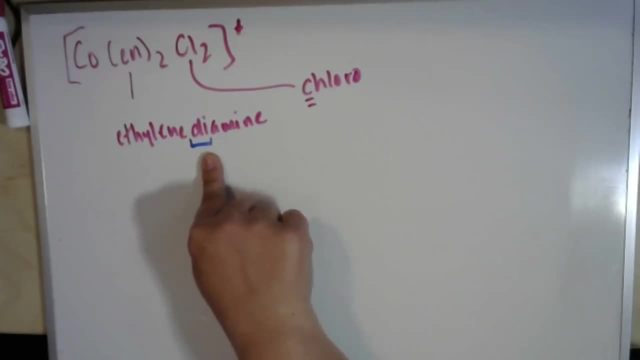 there is at least one prefix in the edta. there's more that's within the name of the, the ligand itself. so they're going to need a different prefix to put out front that indicates that there's more than one of these full ligands. all right, um, but we'll get to that when we're. 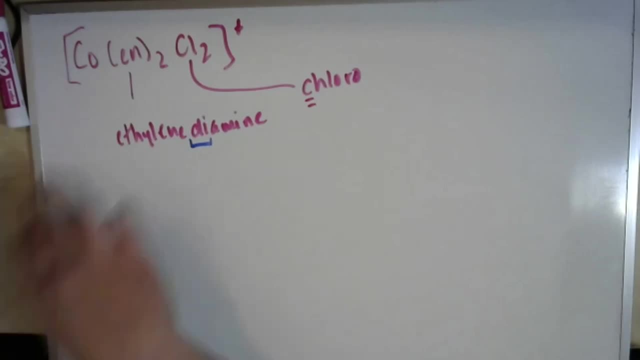 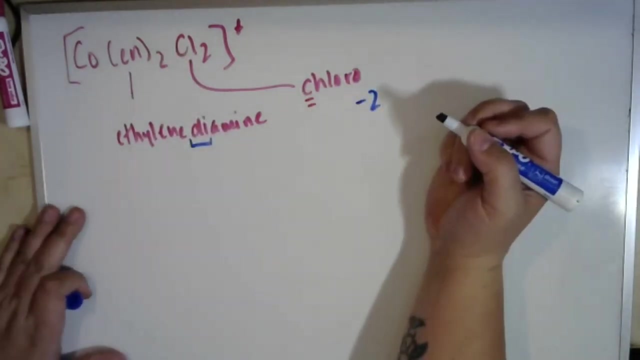 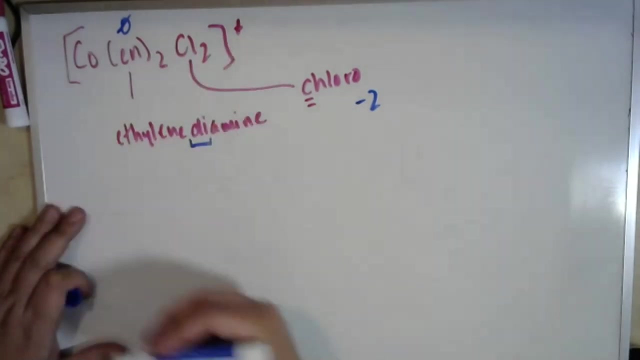 doing the number parts, let's find the the charge on the cobalt. here we know that there's two chlorines, so it's going to have a negative two charge. uh, the ethylene diamine is neutral, so that'll have a zero charge and we have to end up with a positive one charge. 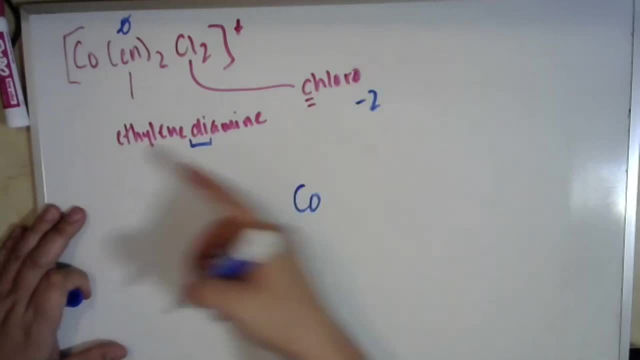 okay. so basically cobalt, the cobalt minus two has to equal positive one, right? because that's the contribution from the chlorine and that's the overall charge on the on the ion: here i like to set it up like little math problems. so the cobalt ion is going to have a charge of plus three here. 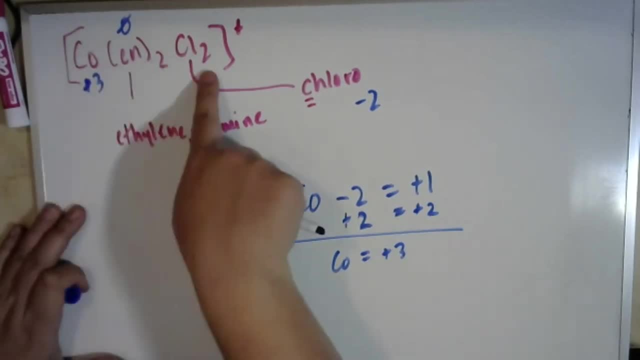 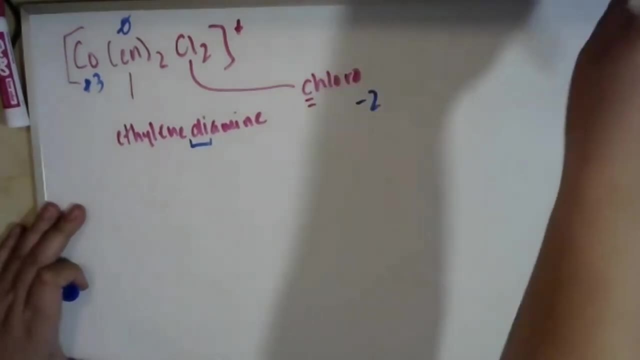 right and that should make sense. right because if you have plus three cobalt and you have negative two chlorine, you're going to have an overall charge of positive one. so with all that information we can name our complex ion. we're going to have two chlorines. 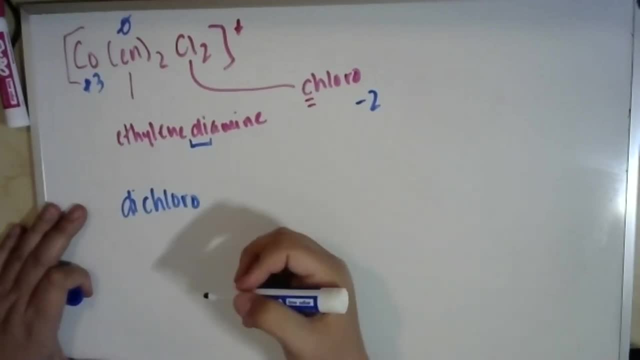 so it's going to be dichloro, and then we're going to have two ethylene diamines and the prefix the. the specialized prefix, meaning two, is this: so you just have to put bis in front of ethylene diamine, okay, and then we'll name our metal. 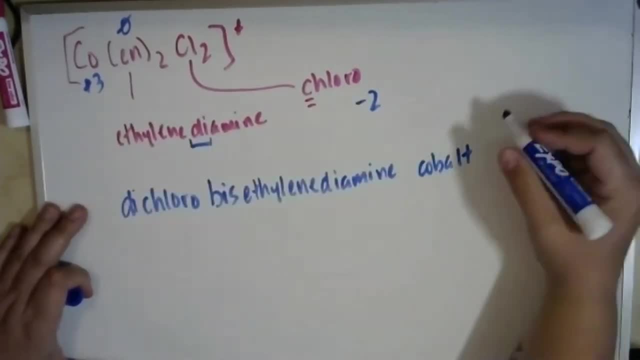 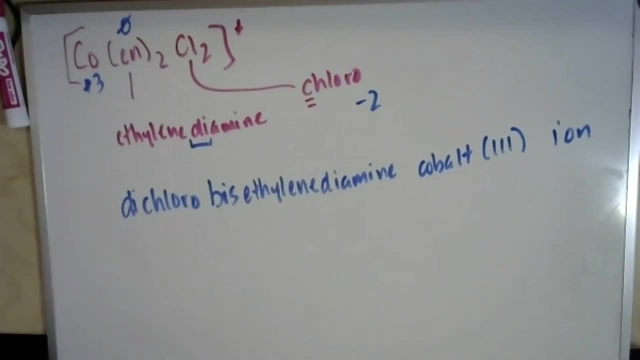 because it's a complex cation. we don't have to change the name of this metal, all right. so i just wanted to throw that in there, because we didn't have any of these specialized namings and the examples that we went through. all right. so now let's look at the isomer, the isomers of this guy. 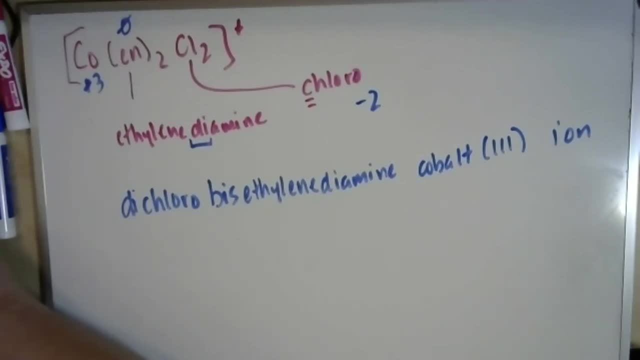 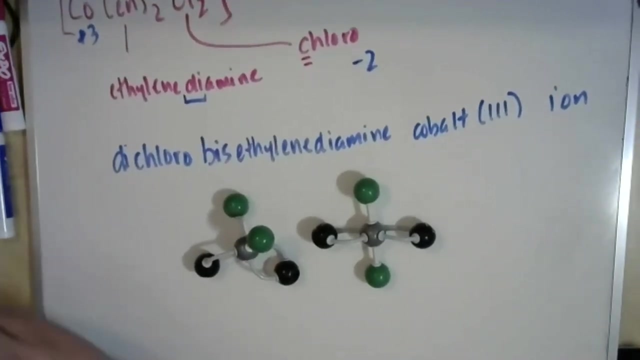 okay now i did my best with this um to try to show um. i did little molecule guys here that we can talk, talk about. okay, to try to demonstrate the different types of isomers. i think sometimes it's a little bit easier to see when you have the um, when you have the structures in front of you, like this: 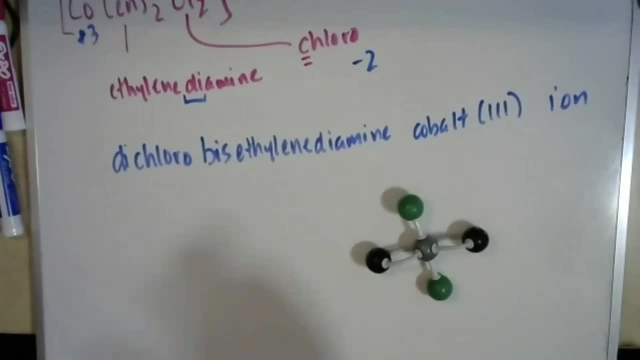 okay, so you're gonna have cis isomers and trans isomers here. all right, um, your your textbook gives you generalized formulas that can like help you identify whether you have cis, trans isomerism or isomerism. okay, so, if you have a type of isomerism where you have, um, it's your central metal. 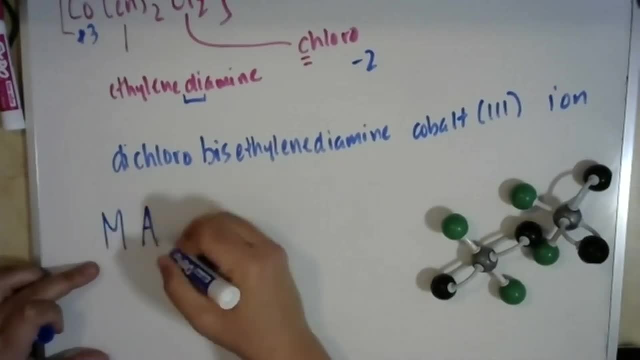 that's what the m is going to represent. and then one of your ligands would take up four spaces and another ligand takes up two spaces. this type of orientation is one that can lead to cis trans isomerism. okay, and with this formula we have two ethylene diamine. 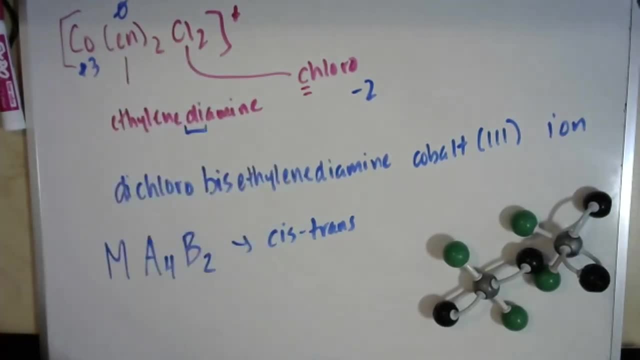 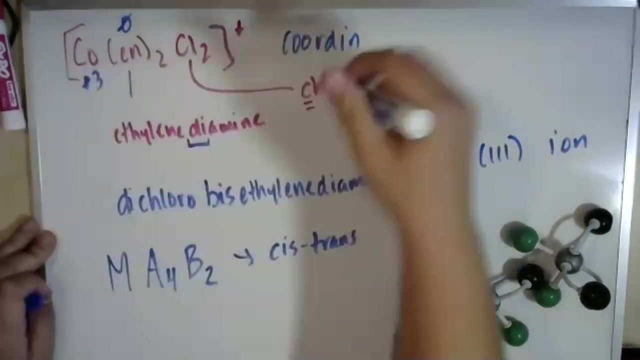 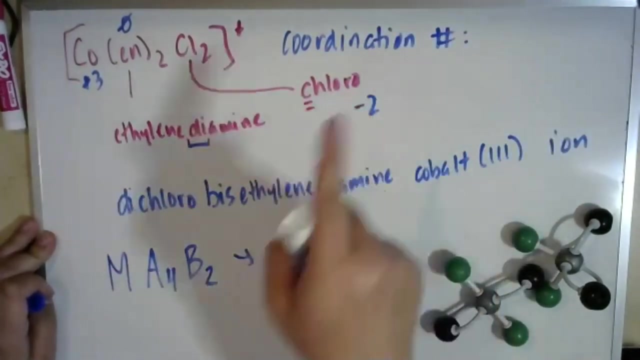 and two chlorines. right, your ethylene diamine is- this is a great question too for coordination- number man, your ethylene diamine is bidentate, so it's going to have two places on the molecule where it can attach to the cobalt. okay, speaking of that, if we were going to find the coordination. 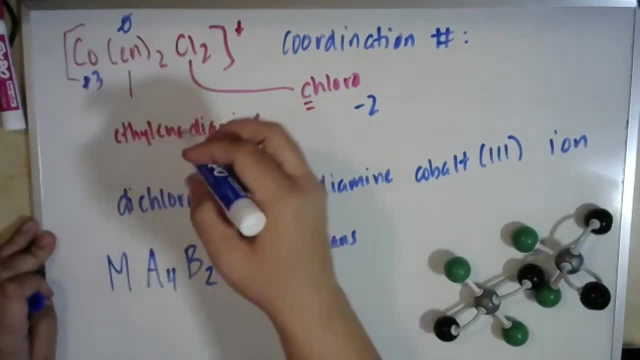 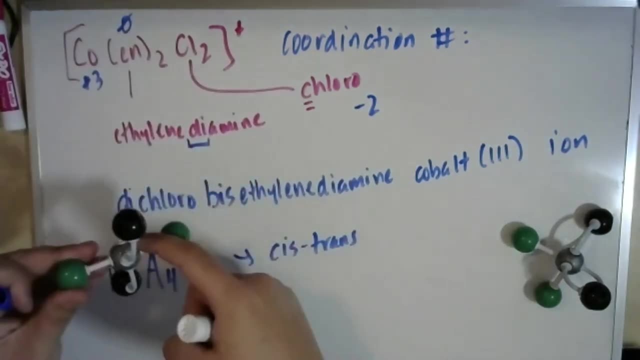 number of the cobalt in this ion. we would have to take into account the cobalt number of the cobalt and the course number of the cobalt in this ion, which we're looking at now, but also in terms of including treatments as a physical structure, as a trapezoidal particle. 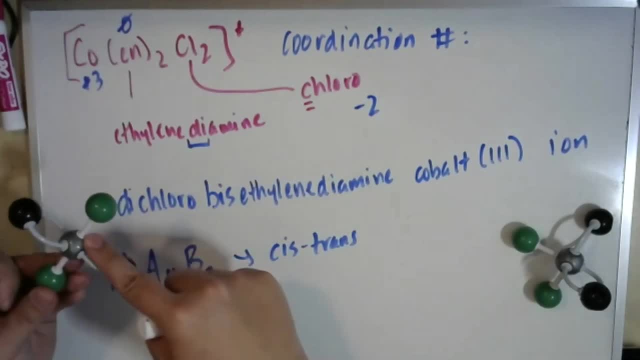 so we're going to come back here and i'm going to start by saying what are the personal lymphatic classic transmittal denominations. so if you have brow oz, uma, we have brain cell comme. in this case, we are fiberwest and supertoxazol. 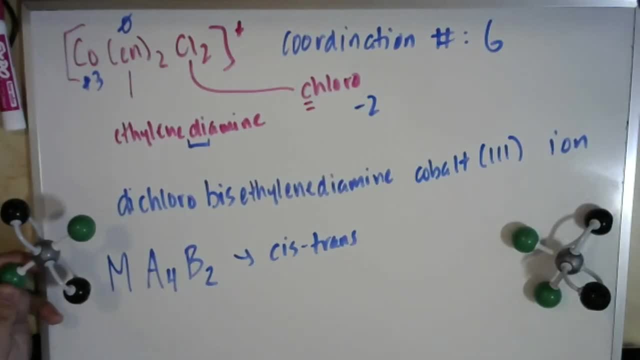 six. Okay. Now, cis-trans isomerism has to do with the location of- I like to think of it, personally, as location of these two things, of the two. Okay, If the two things are next to each other, or if they're across from each other, Okay. So this is an example of the trans isomer. 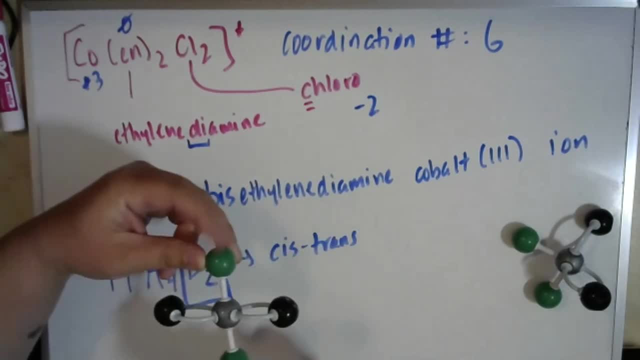 because the two chlorines in this case are across from one another. All right, I think it's easiest to recognize like which type of isomer is trans versus cis, based on whichever you have fewer of. Okay, Once you are looking at the cis isomer. 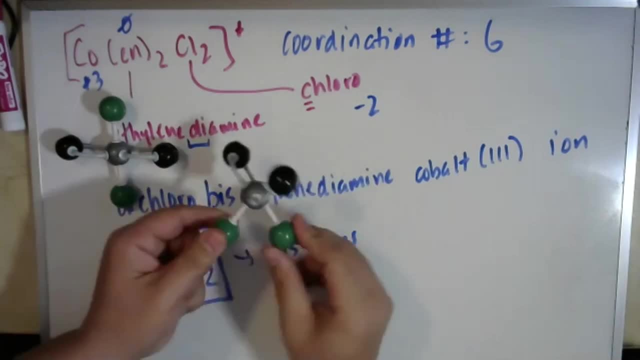 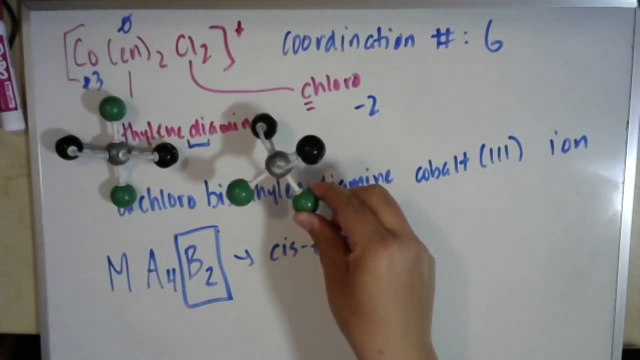 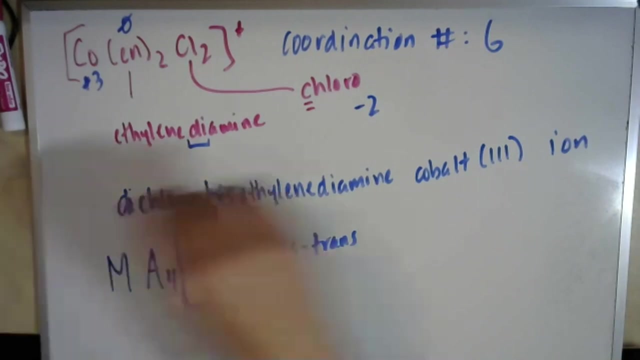 now your two chlorines are going to be right next to each other. Okay, So that's going to be a representation of your cis isomer. Hopefully that makes sense. The second example: what is it? Okay, The second example that they give us is: 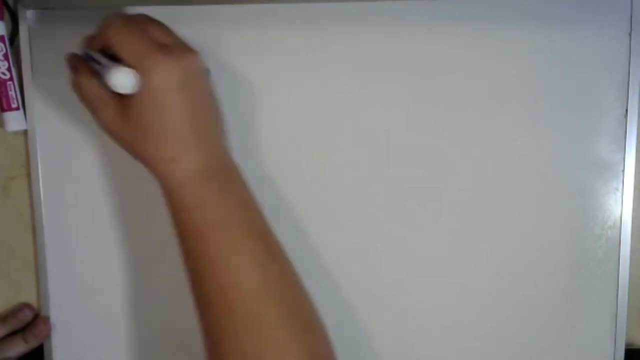 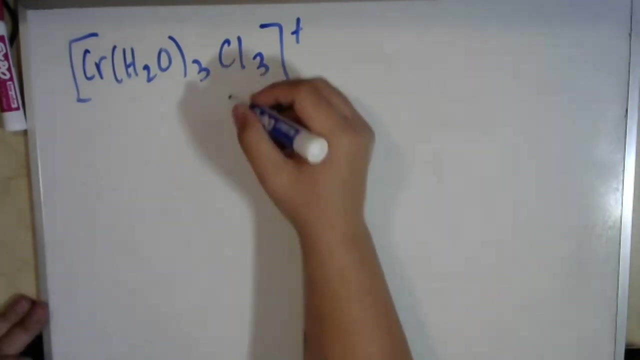 CR, H2O3, Cl3+. okay, I'm going to name this again real quick because I think it's a very good idea to be practicing this. We have three chlorines. That's going to be a negative three charge. 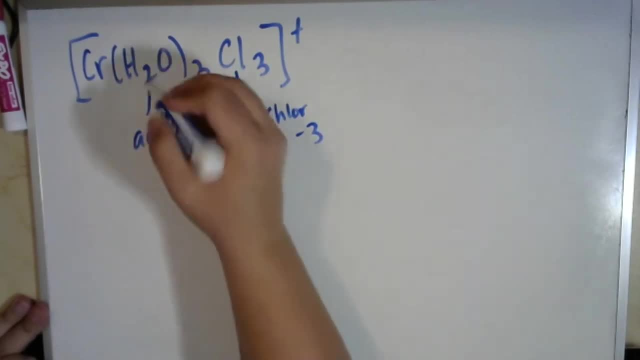 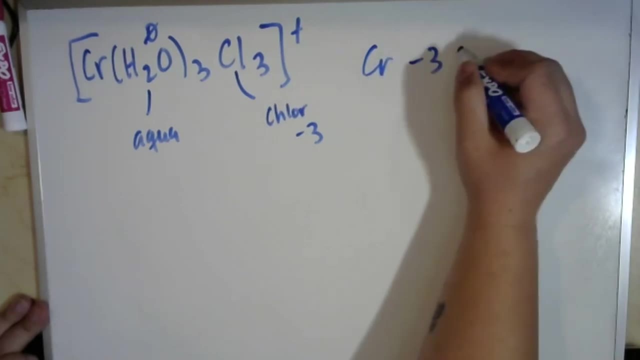 We have three waters. That's going to have a zero charge. So our chlorine, Now that our class is actually positive, 1 chromium minus three has to equal positive one. So our chromium is going to be plus four here. Okay, This is a complex cation, Again, we know, because it has a positive charge up here. 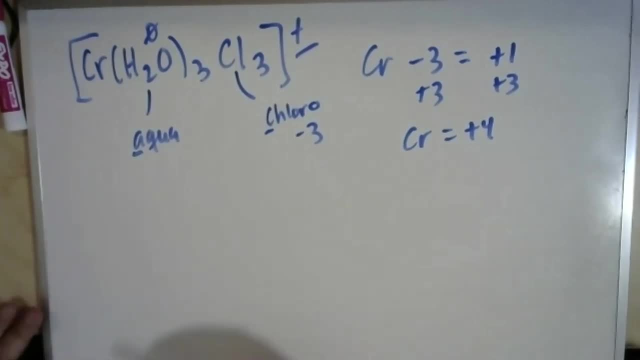 I'm going to have to put my aqua before my chloro, because A is before C. Now I can name that triaqua trichloro chromium ion. okay, We also know that this has a coordination number of six, because there's three chlorines and there's three waters. 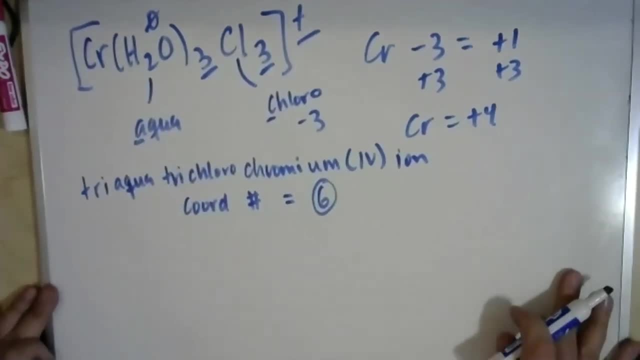 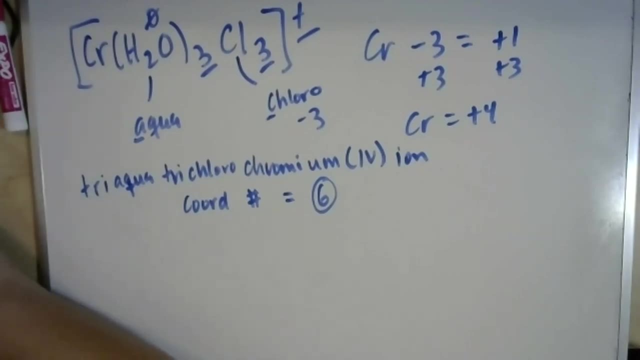 and chlorine and water are both monodentate ligands. All right. now the general formula here is different. okay, What we have here are three of each types of ligand. So the generalized formula is: if M is our central metal, is going to be that we have. 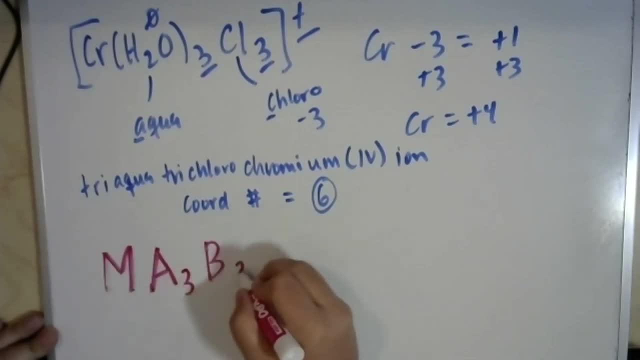 one ligand with three and another ligand with three. okay, This general formula is one that can result in fac mer isomers. okay, three and three. Now it might be. it's sometimes easier to understand what this type of isomer is if you really break. 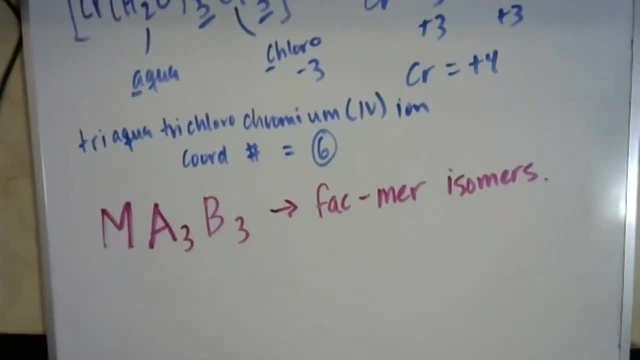 down what the names of these things are. okay, The fac isomer stands for facial, I think, But what this means is that the ligands- like all three of one of these ligands- are going to take up one face of your octahedron. okay, 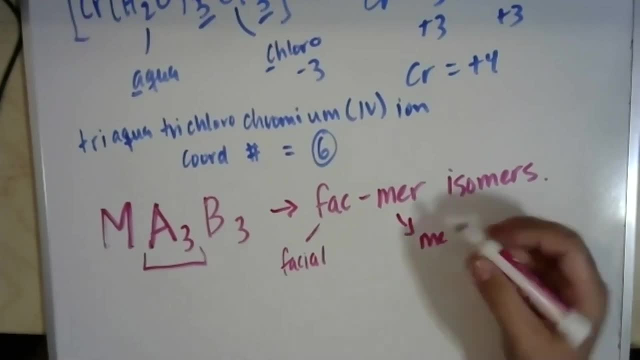 The mer stands for like meridian or meridional or something, And in this version of the isomer, three of your ligands are going to kind of they. they make an almost an arc around the middle. Okay, And that's where, like, the meridian term comes from. 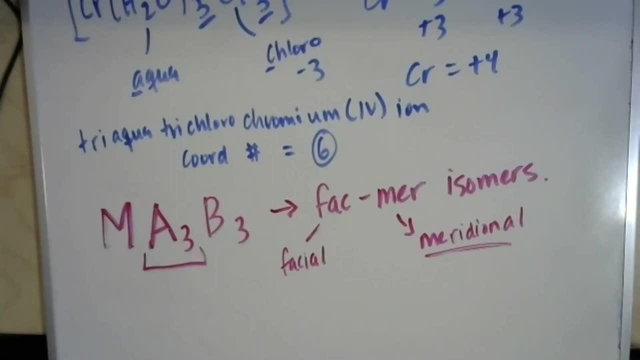 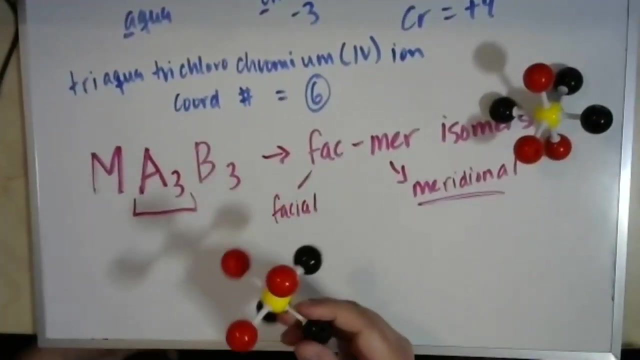 So I kind of let's see, are they over here? I was trying to create these before I started this video so that we could look at them. Okay, so we're going to have. we have two types of isomers. This would be considered the- the fac isomer, the facial isomer, because you have all three. 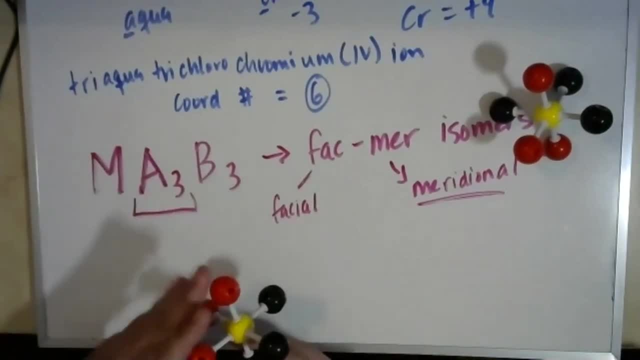 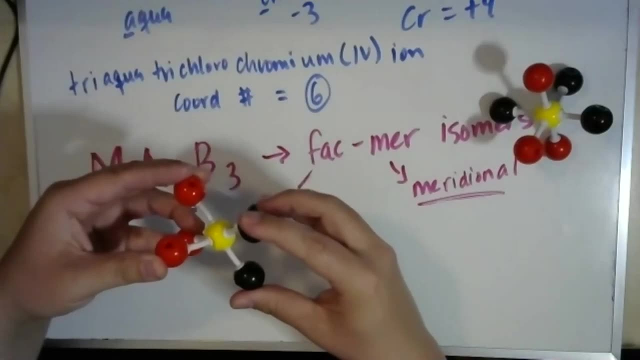 it doesn't matter whether you're calling these the, the chlorines or the waters, right, But all three of these ligands are grouped on one side and all three of the other ligands are grouped on the other side, So one face of your octahedral is just going to be, I don't know, chlorines. 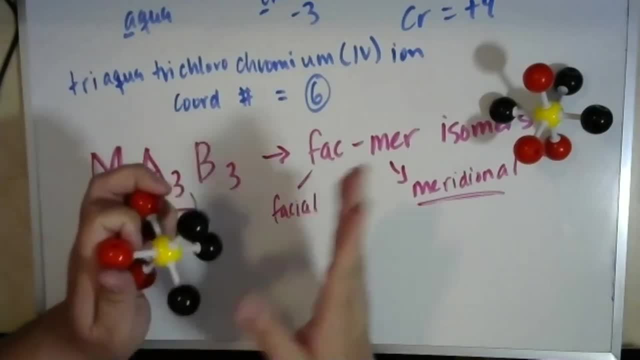 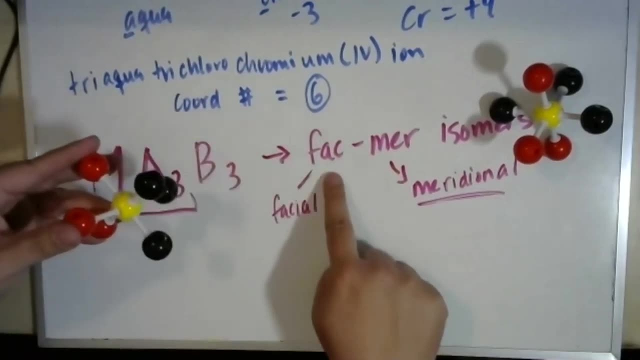 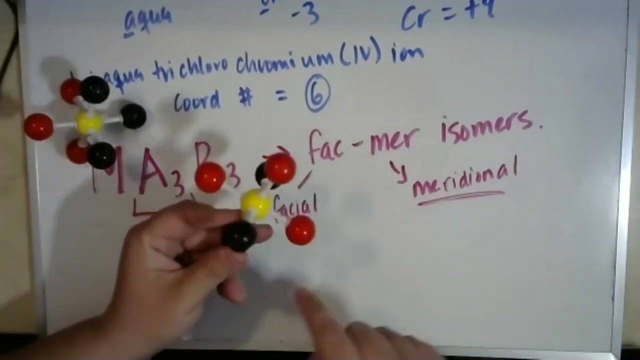 the other face is going to be the waters. All right, So you're going to see the cluster of, of the, of three, each next to each other, for the fac isomer, For the meridian isomer, the arc that I'm talking about happens because 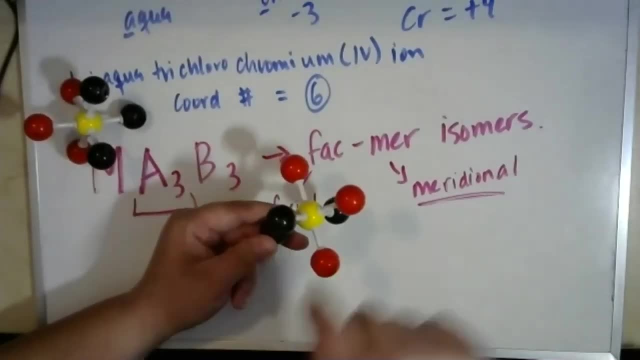 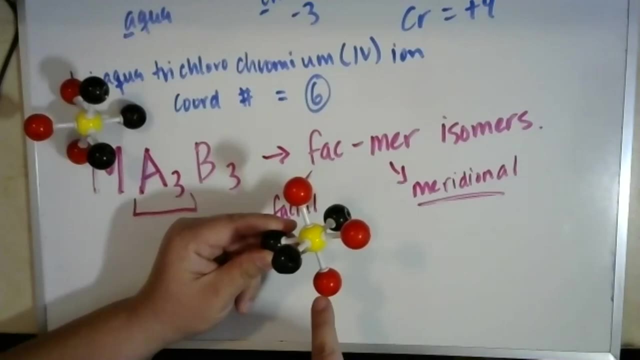 you see, you have let me sort of: yeah, like this, see, this is like the middle of your, this is like your central plane here. And what do we have? We have an arc around the middle. Okay, So the three, the three ligands, are not grouped in a way that puts them on the same face. 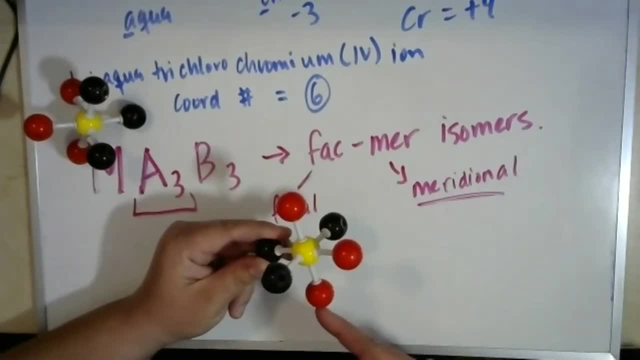 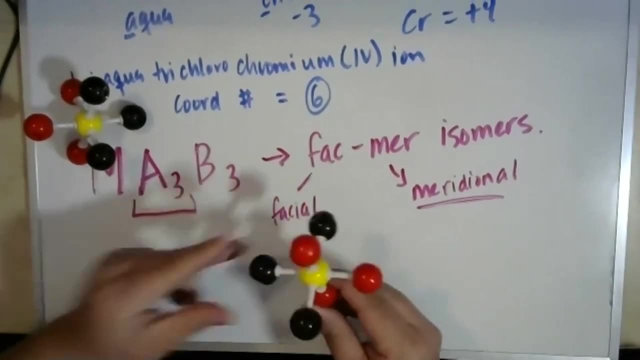 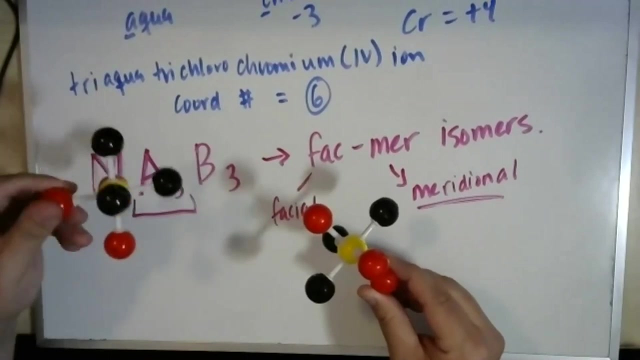 Instead, they're lined up so that they're crossing the middle of the structure. All right, Um, you're gonna notice that when you have your your fac isomer here, like no matter what way I'm holding this, I always end up with different. 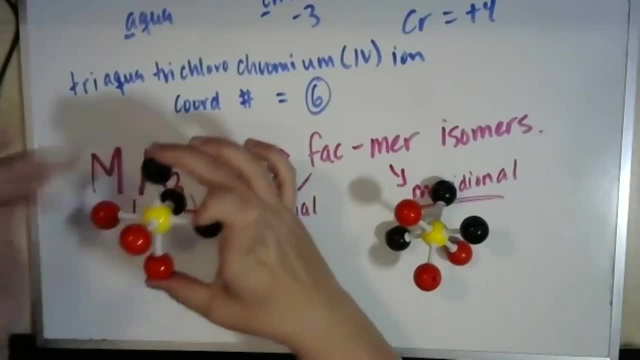 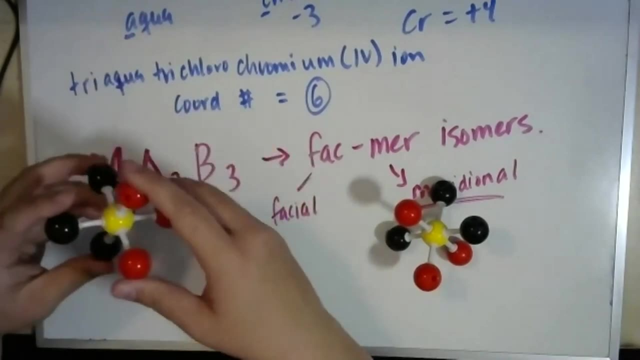 ligands on the top and the bottom. Okay, It doesn't matter which way I put it, I'm always going to have different ligands on the top and on the bottom. Yeah, the top and the bottom. and that's because, all you know, they're grouped in a way that puts them all. 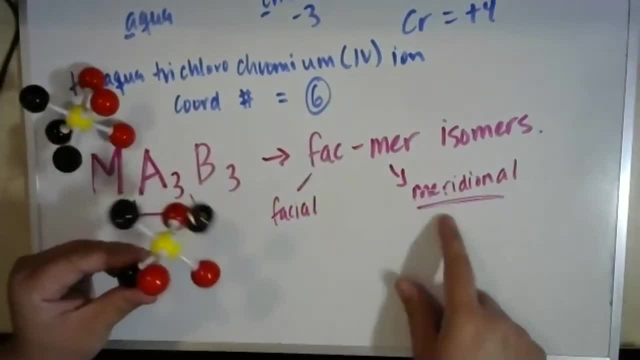 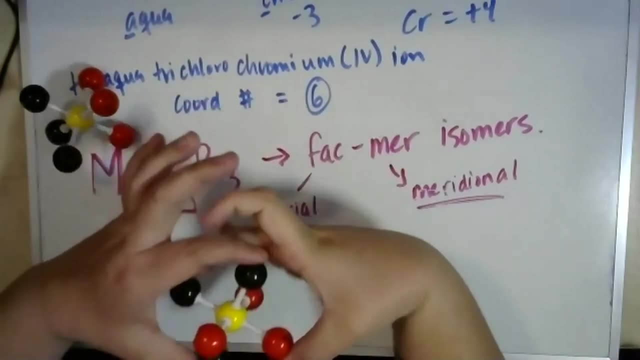 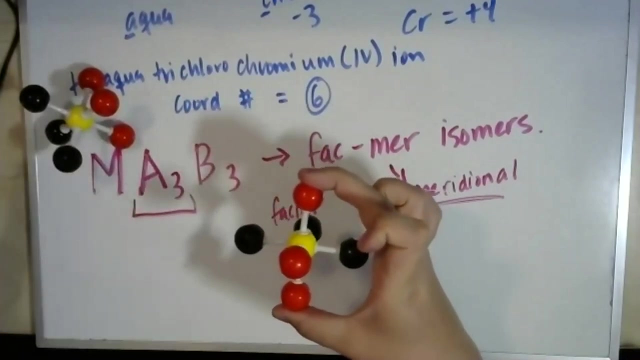 next to each other in my meridian. I can orient this in a way. I mean, I definitely it's not every way, but I can spin it and orient it in a way so that I have two of the same ligands. okay, I have the option of that here, or I don't have the option in the other one. okay, but I do see that my my. 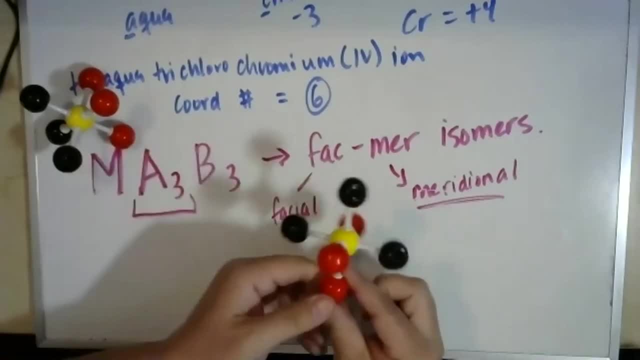 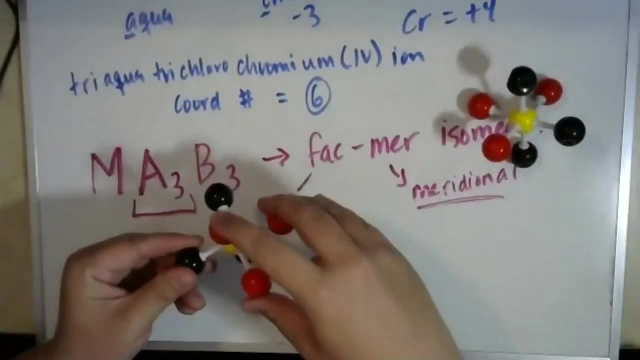 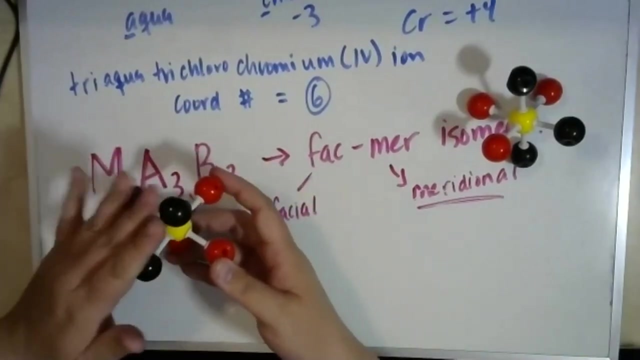 ligands form this, this arc along the center. okay, arc along the center, that's the meridian isomer, and then this is the fac isomer. so that's going to be a face, right, they're all grouped together like that. this is going to be another face. they're grouped together like that. 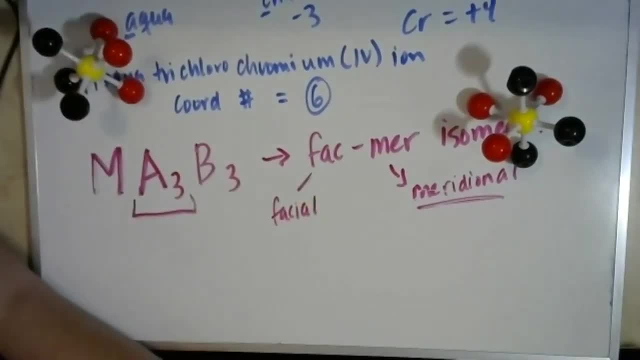 all right. um, I hope that visualizes. I hope that visualizes it better. I have a lot of trouble seeing the isomers, so I do feel for for people when they're trying to learn this. um, I'm definitely a person that when we were doing um optical isomers in gen kevin in organic 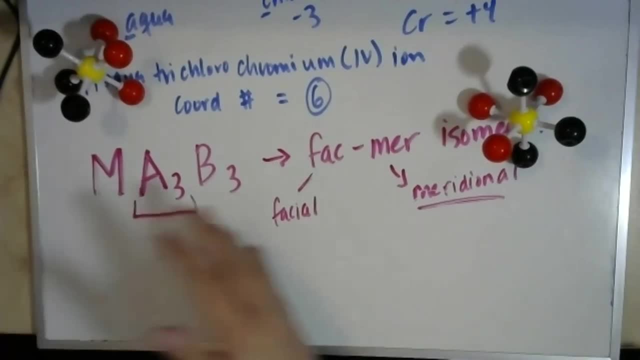 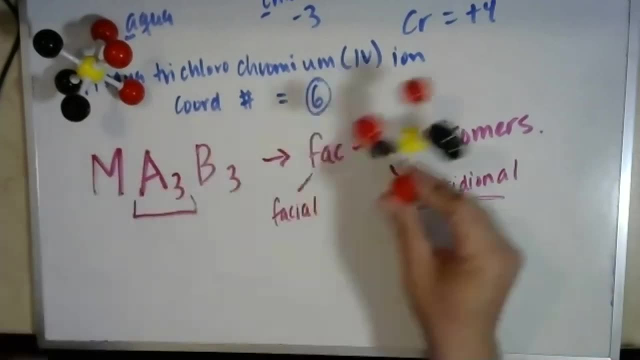 chemistry. I needed the model kit because I couldn't just see them like some people can. you can describe this to someone and they can see it, and I can't see it like. I have to be like holding it in my hands and looking at it. but that's all right, you know. 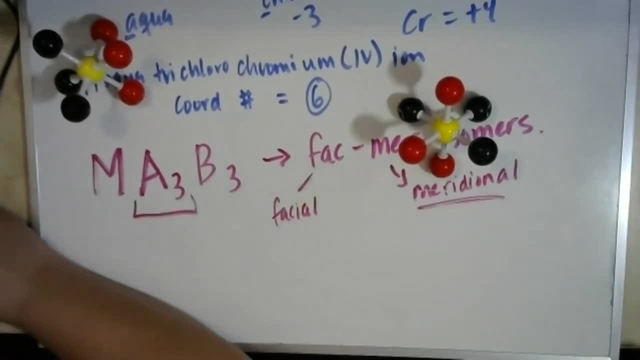 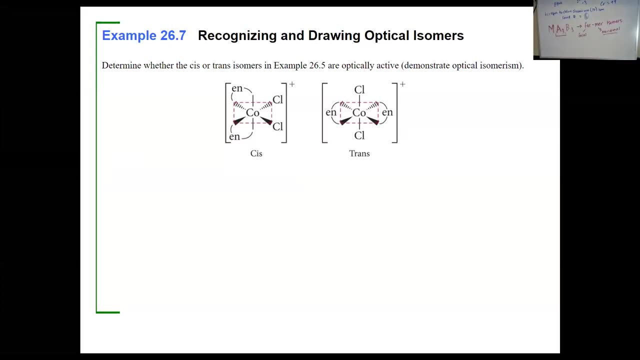 okay, that's why you got to figure out what works for you. basically, we're going to look at that first isomer and we're going to decide whether it's optically active. now, okay, we'll bring these ones back in here. um, I didn't have enough to make two of the trans isomers. 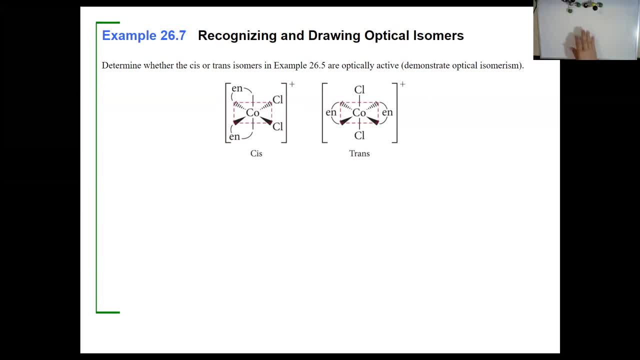 we'll talk about the the cis isomers first. um, but I'm hoping that you can kind of: yeah, then we'll do the the trans one. all right, so they want us to look at the cis and trans isomers here and decide if they're optically active. 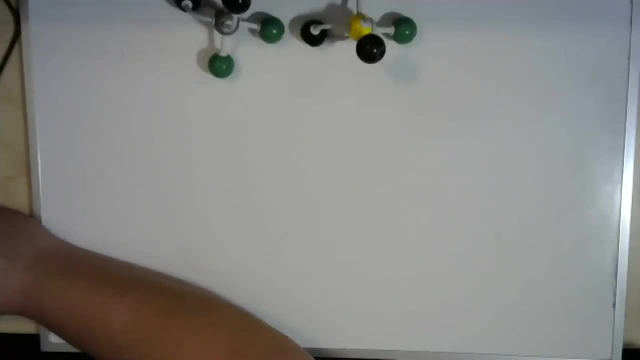 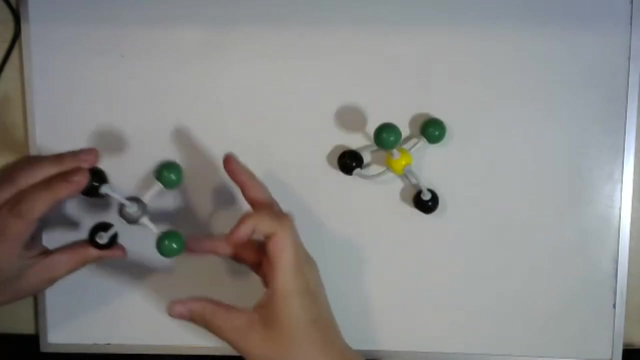 okay, something is going to be considered optically active if they they do not have a super imposable mirror image. that's the wording of it. okay, so we're going to talk about what that means. so this is a cis isomer. remember, we have the two chlorines next to each other and then the two 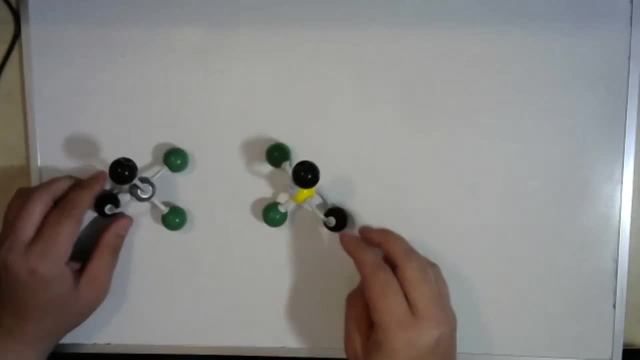 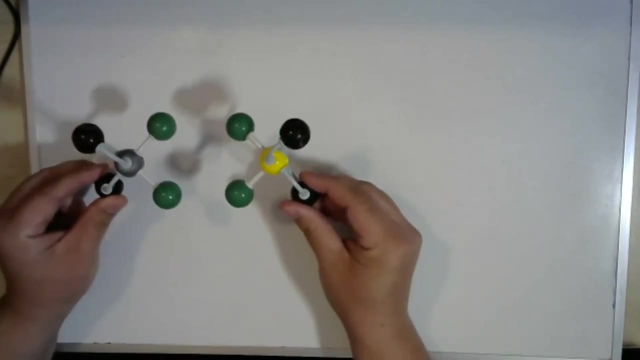 ethylene diamines next to each other. so, to start with, when you're deciding whether something is a optical, optically active, or not, you have to kind of imagine them like they're staring at each other in the mirror. okay, so like everything's the same, they're looking at each other. 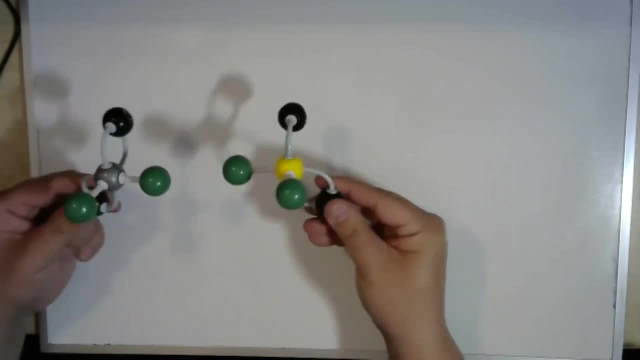 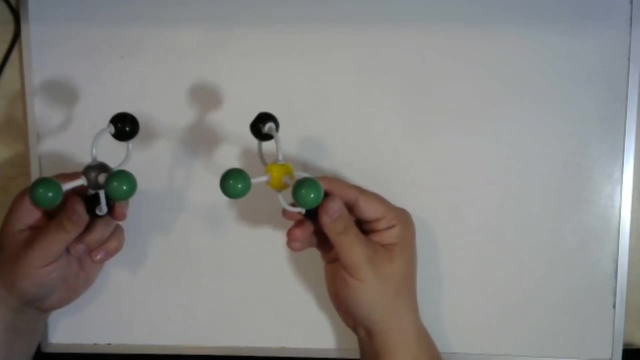 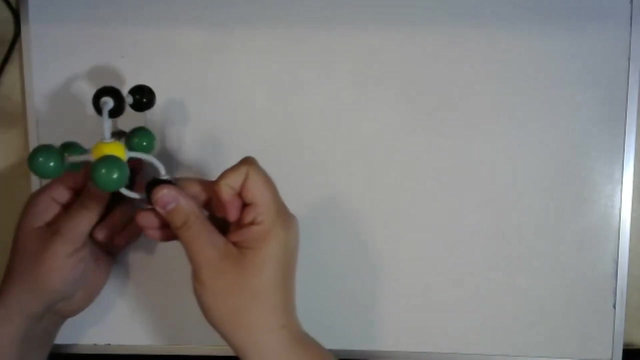 and then you have to flatten out that mirror image, all right, then you have to take that mirror image and you have to put it on top. okay, when you put it on top- and i know this gets a little bit harder to see because you know we're not- i don't have like. 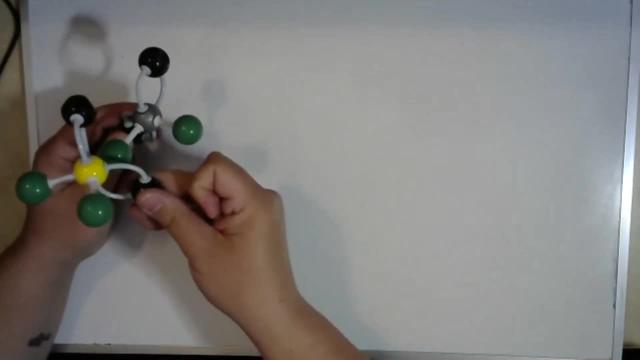 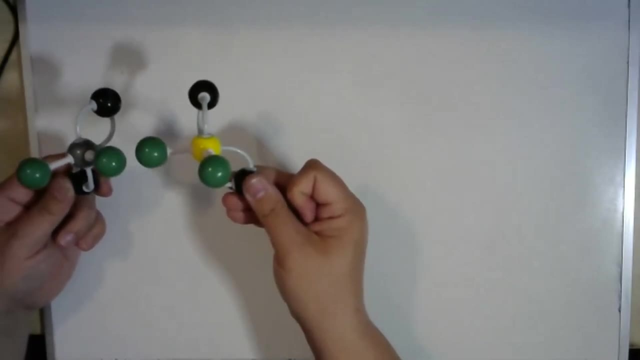 we're not in person or anything and i don't have like a good 3d screen, but when you put it on top, if the orientation of all of your atoms is identical, then there's no optical activity, and then you have to take that mirror image and you have to put it on top. 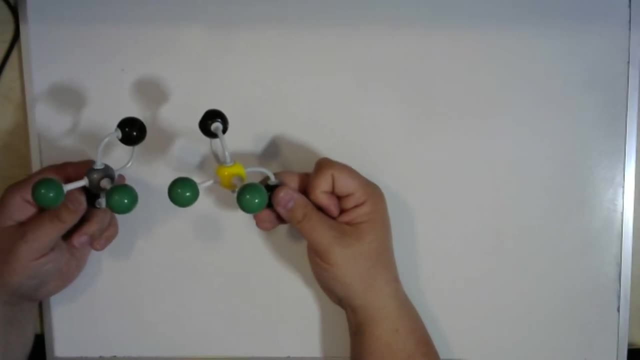 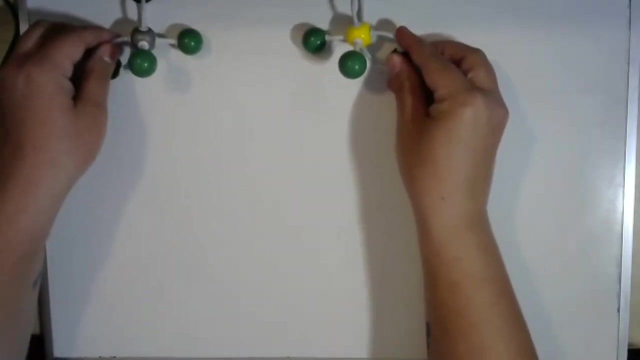 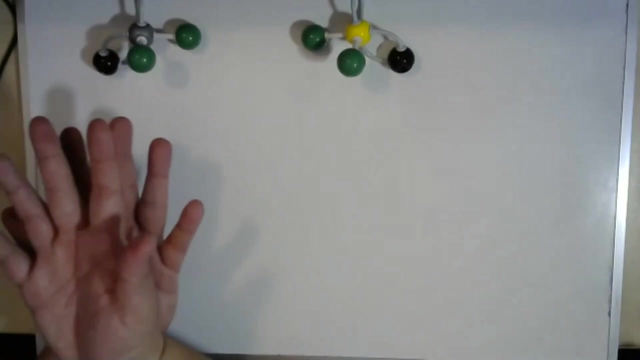 if there's any differences, though, then there is optical activity. okay, now the the i. the idea that you can use your hands, um, is often talked about here, because, like you, could say that your hands are mirror images of one another. and then, if you flatten your hands out and you put one hand on top, 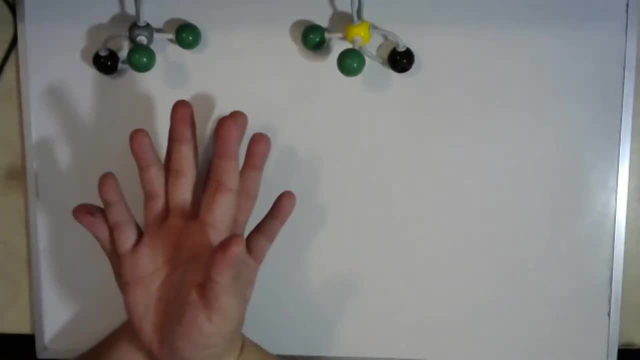 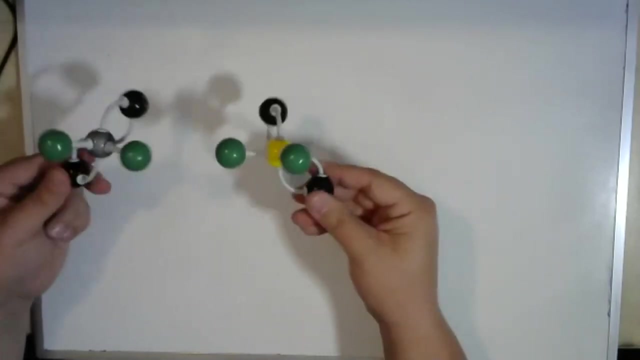 of the other, like your pinky and your thumb. well, there are over here and that's not going to change, right? there's no way you can, like, rotate your hand, um, within the same plane and make them the same. all right, that's what we're looking for here. so when we take our mirror image, we flatten it out. 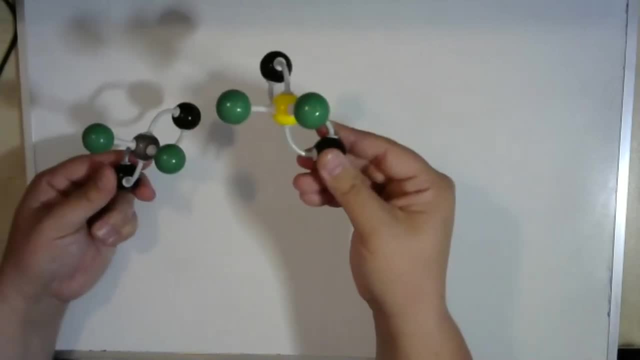 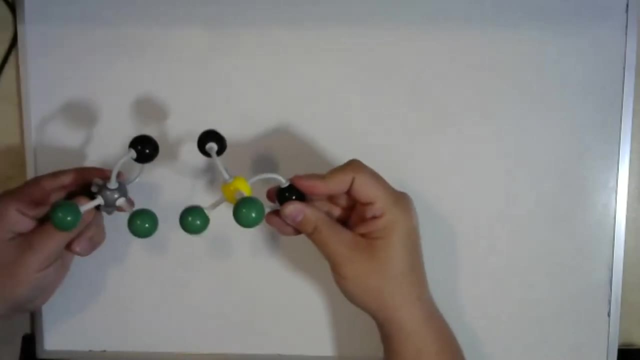 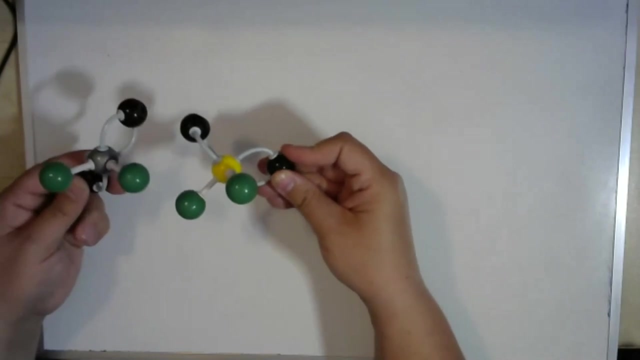 and then we try to put this, this um, flattened out image on top of the other one. there's differences. okay, the orientation of these is different because these two- i'm just banging them together- these two things are going in different directions in space. okay, and even if i rotate it, okay, even if i rotate. 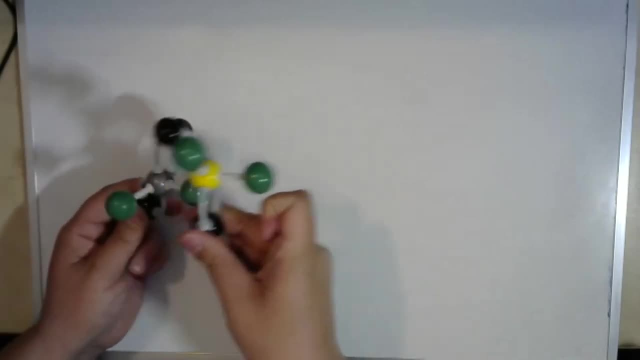 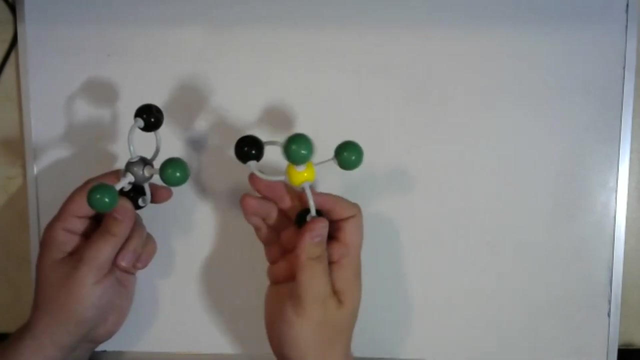 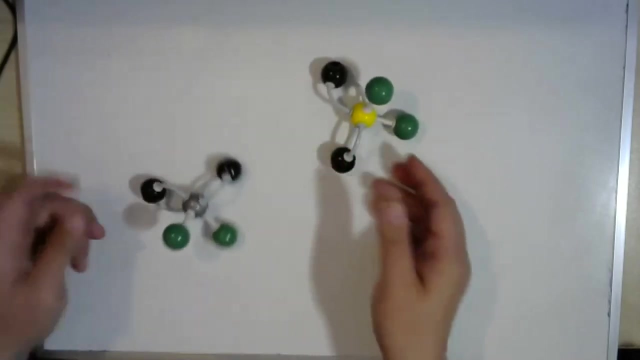 this molecule, i still have a different orientation. it's still not identical. no matter what way i rotate this in the same plane, i am never going to be able to make the cis isomer fit directly on top of of its superimposed image and and make it so that the the both shapes are the same. 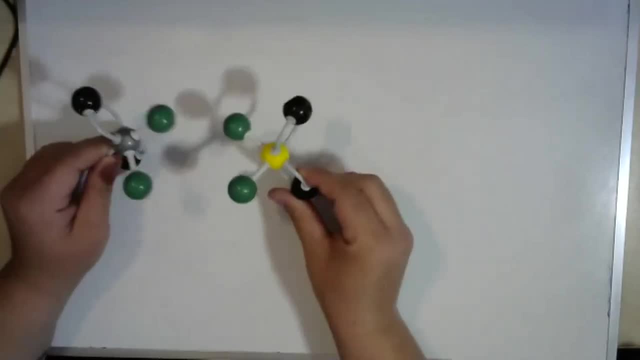 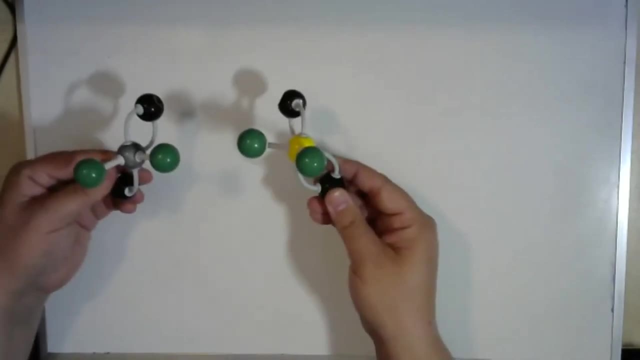 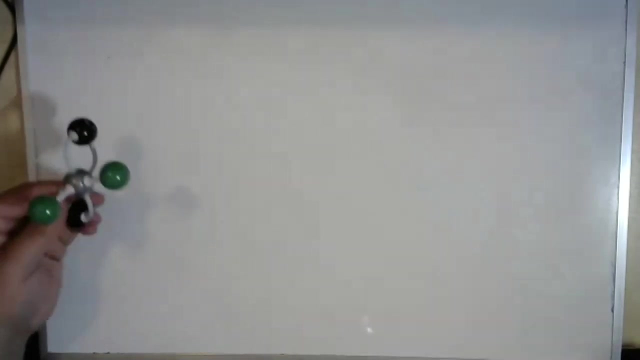 okay, when that happens, that causes optical activity. okay, when you can't make the mirror image sit on top of each other- perfectly, that's what causes optical activity. now let's look. look what happens in the, the trans isomer. okay, i just have to rearrange this real quick. 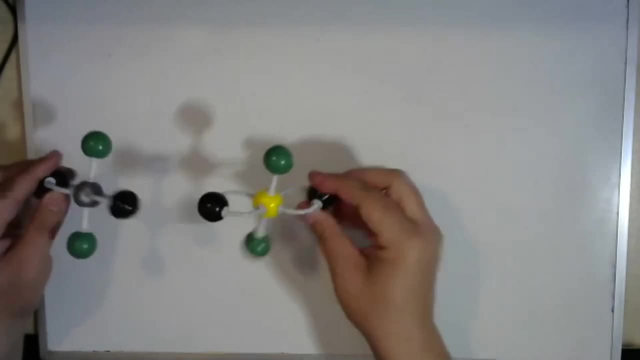 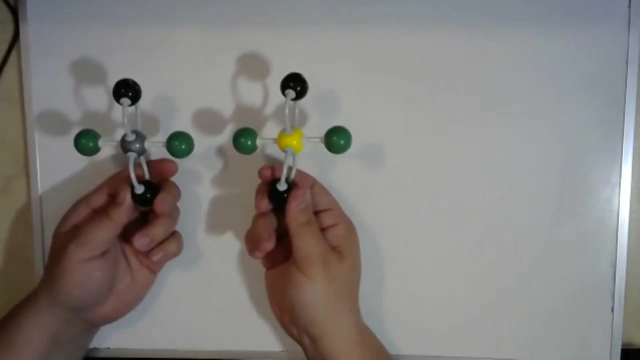 okay, i use a different color central atom, just so we can keep track of them. right? so they're looking at each other in the mirror. okay, we flatten them out, and now i put one on top of the other. this is exactly the same. see, like there's no difference. 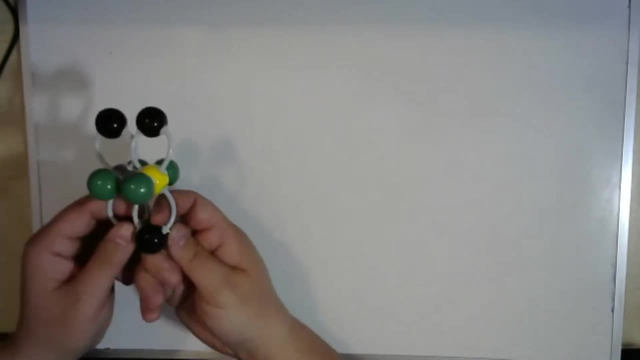 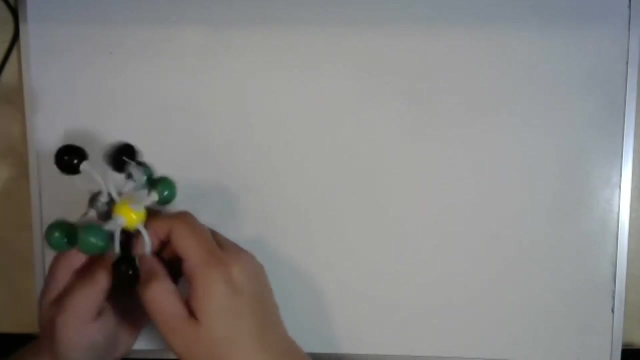 there, everything's in the same plane. they're perfect. no optical activity here. this one is not optically active. all right, so those are the differences that you're looking for when you're trying to decide whether something is optically active. um so, hopefully that's a little more helpful than the just the two-dimensional pictures in the textbook. 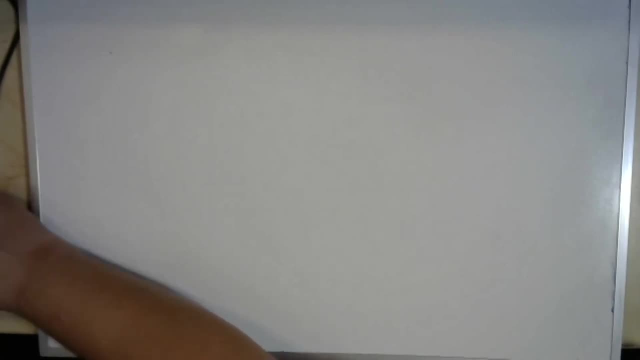 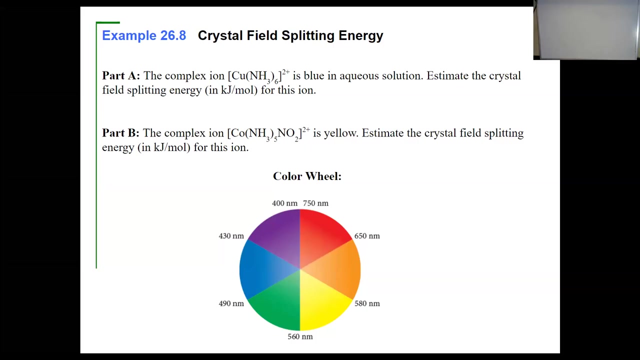 all right. the next question is going to bring us back to some math. okay, i included the color wheel in this question, um, as a guide, because i think that if you saw a question like this, um, something like a color wheel would probably be included for reference, um, so you could pull out the appropriate wavelengths from these. 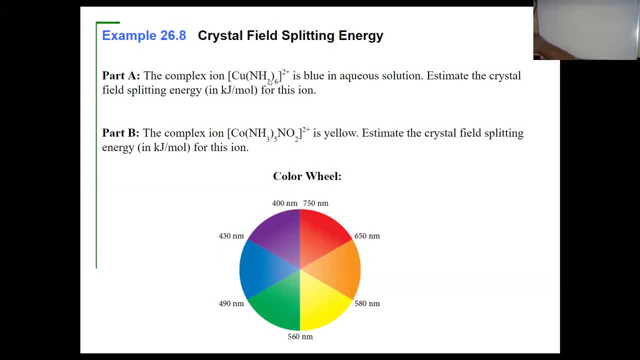 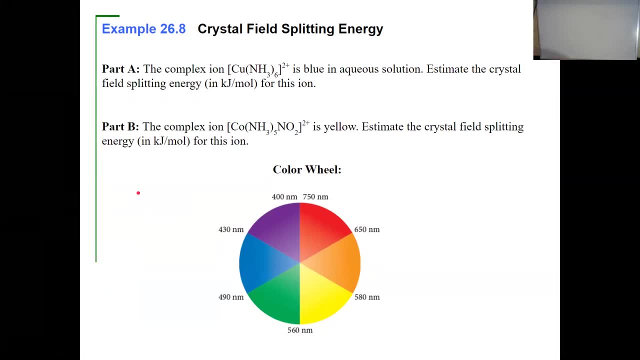 so the first question says that the complex ion for cunh362 plus is blue in aqueous solution. we're going to estimate the crystal field splitting energy in kilojoules per mole for this ion. kilojoules per mole, okay, so let's write that down: kilojoules per mole. 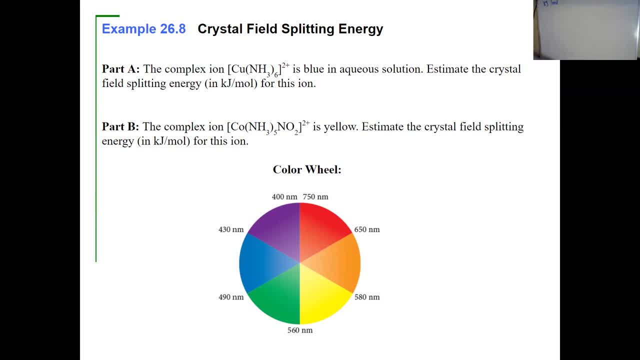 okay, now there's a few things that you have to be able to pull out of this question. first of all, they're saying that the the solution itself is blue. if a solution is blue, that means it's absorbing its complementary color, right? so if, if a solution is showing blue, 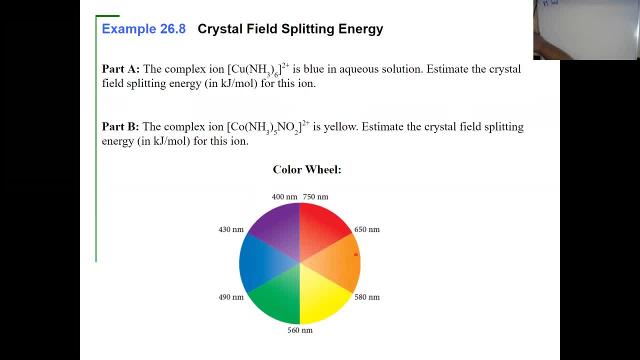 that means it's going to be absorbing orange. all right, so that's the first association we have to make here. we have to know that it's absorbing orange And because we're estimating the crystal field, splitting energy, here we can, we can guess that the wavelength for, like the middle ground over here will be somewhere like maybe six. let me just take- oh, there it is, I'm just going to take an average. 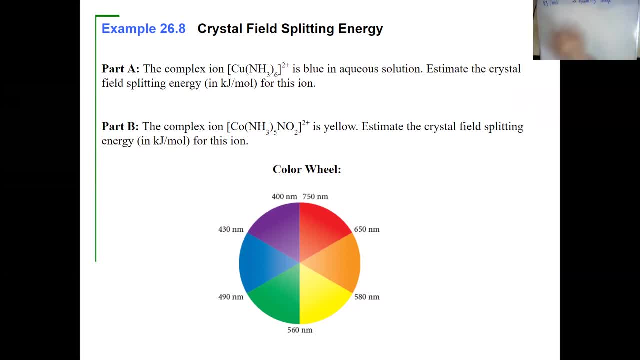 All right, 615.. So we're going to say that the wavelength of the of average orange light, which is right in the middle here, will be like 615 nanometers, And that is all the information that we need to answer this question. 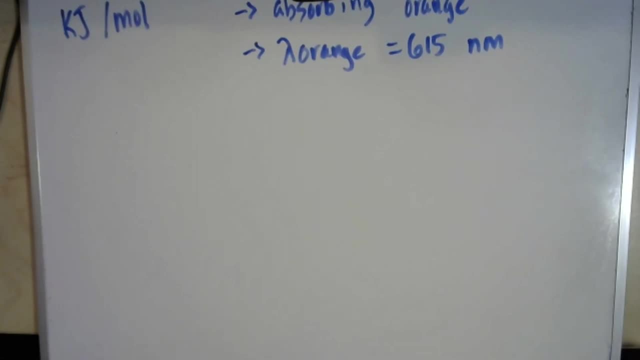 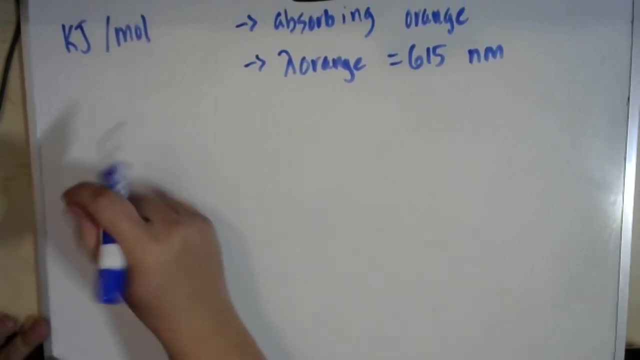 Okay, We have a formula Back from chapter eight again that allows us to find the energy Right In in that chapter we talked about finding the energy of a photon. In this case, we're going to be, we're going to kind of rename it. 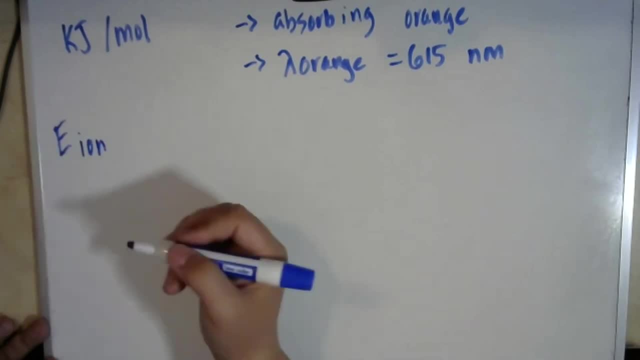 Okay, but it's the same idea. We're going to call it the energy of an ion. Okay, And the energy of an ion is going to be equal to HC divided by wavelength. Okay, so you might have to remind yourself of what some of these values are. 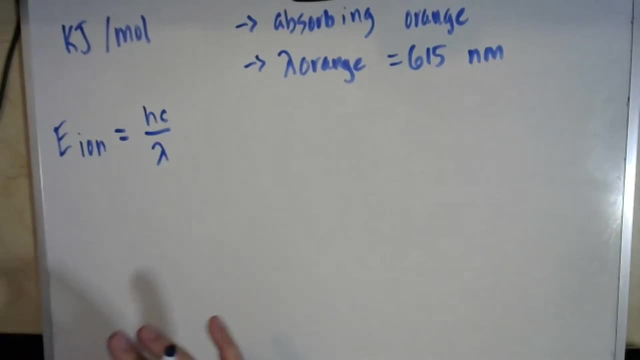 Now, luckily they are on the constants list in the in your textbook. Okay, H is Planck's constant. That's going to be 6.626 times 10 to the negative 34.. Okay, So that's going to be 6.626 times 10 to the negative 34.. 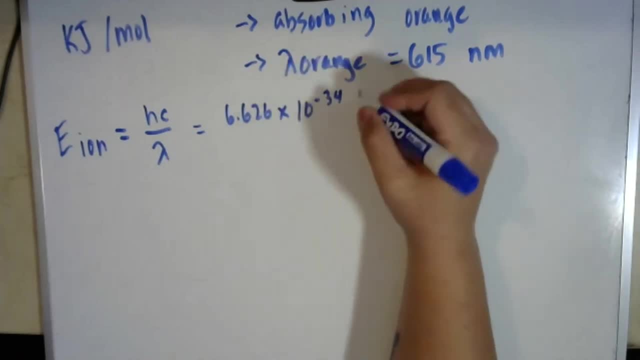 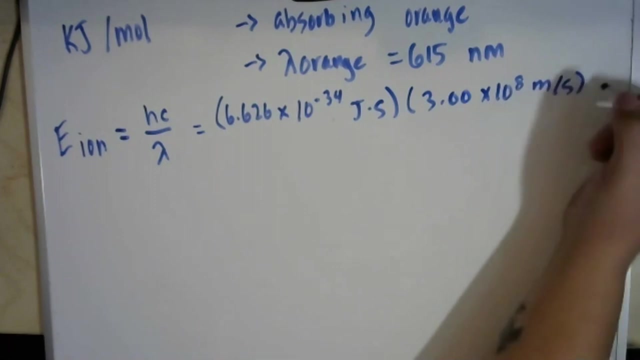 So that's going to be 6.626 times 10 to the negative 34 joules per second. joules times seconds: Okay, C is the speed of light in terms of meters per second. Okay, And your wavelength: because our speed of light is in terms of meters per second, our wavelength has to also be in terms of meters. 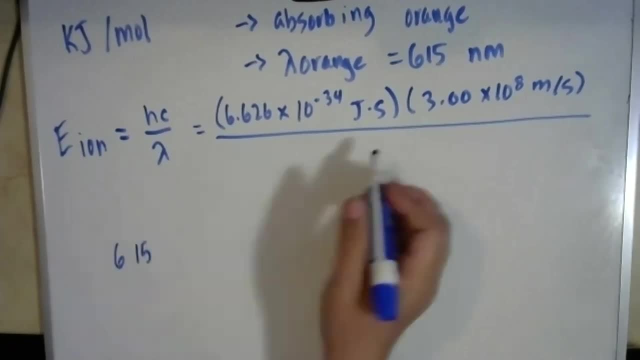 So it might be a good idea to, before you plug it into your formula. if you have 615 nanometers, we know that there are 10 to the 9 nanometers in one meter. Okay, so now we can plug that value in and it will already be in terms of meters. 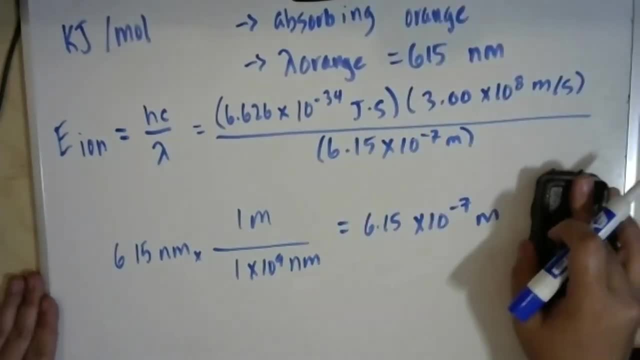 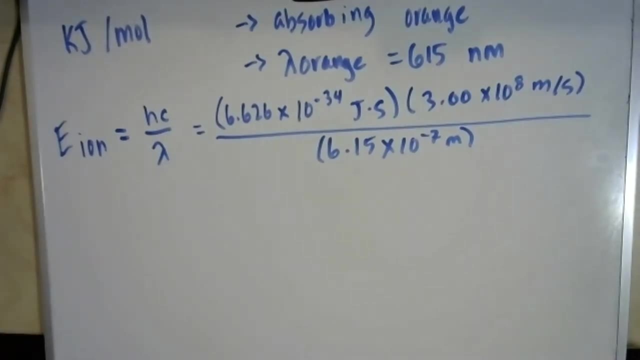 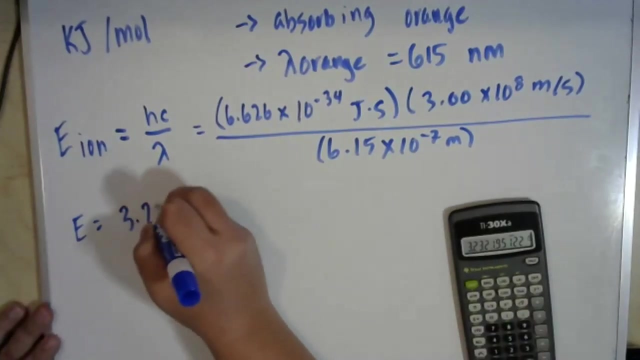 All right, Now we can calculate the energy, the crystal field energy, of one of these ions. All right, And we get 3.23.. All right, And we get 3.23.. Times 10 to the negative 19 joules. 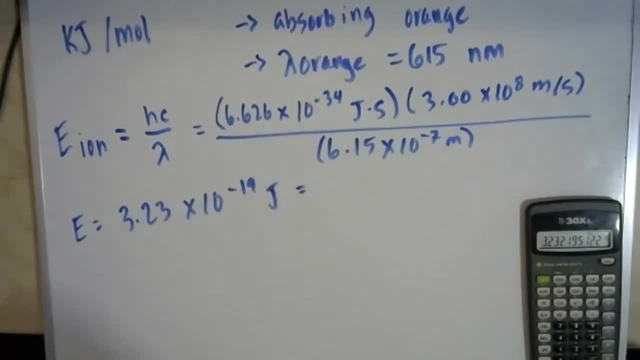 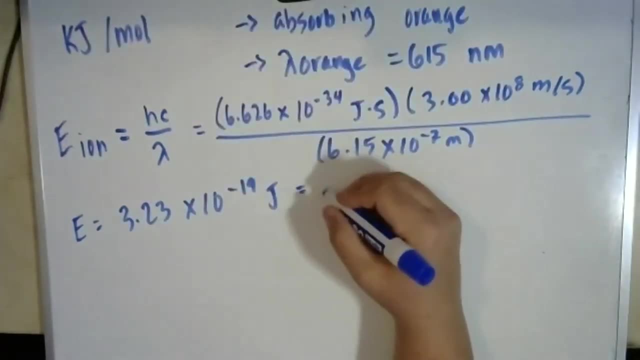 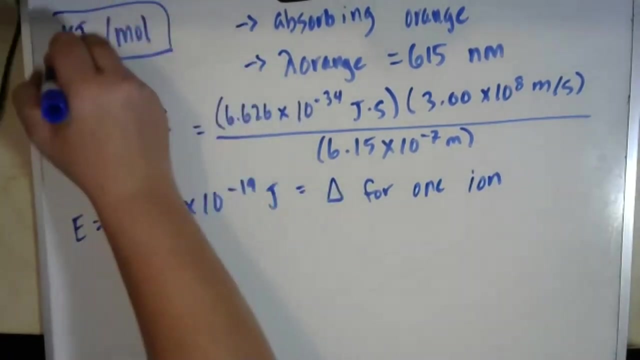 And that is going to be our crystal field splitting for one ion. And remember that little delta sign. that's what this chapter uses to note crystal field energy. Okay, That's a delta for one ion. We want a value in terms of kilojoules per mole. 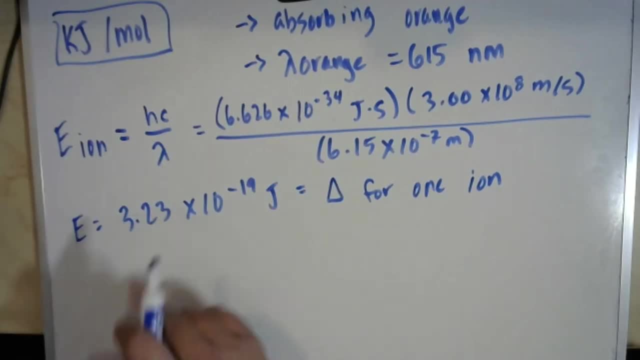 All right. So I have to do a couple of things here. I have to divide this by 1,000 so I can turn it into kilojoules. Okay, And I'm going to have to. yeah, kilojoules per mole. 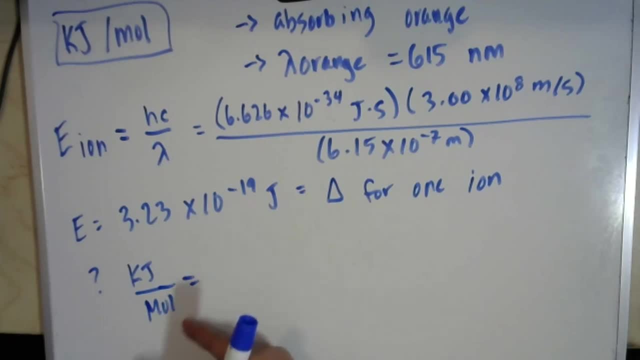 And I'm going to have to use Avogadro's number to get me in terms of moles instead of just one ion, Because right now I know that I have 3.23 times 10 to the negative 19 joules for every one ion. 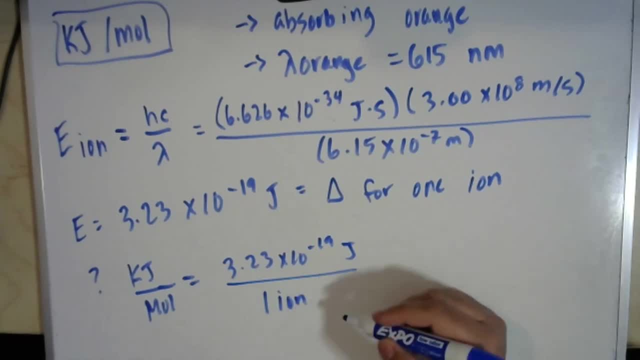 Okay, But that's not going to cut it for the value that I need to calculate, Okay. So instead I'm going to say: well, I know that there are 1,000 joules in one kilojoule, Right. 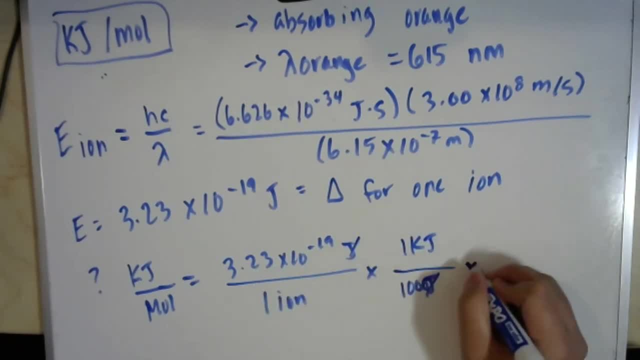 So that is going to allow me to divide by 1,000.. And I know that in one mole there are 6.022 times 10 to the 23 ions. Okay, So now I'm going to be left with kilojoules. 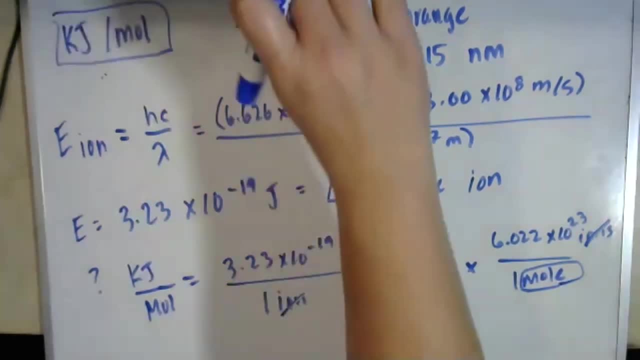 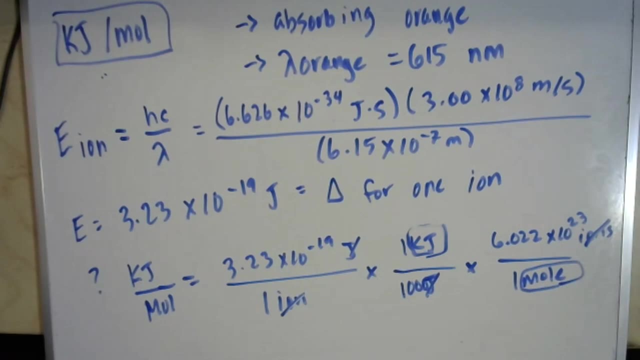 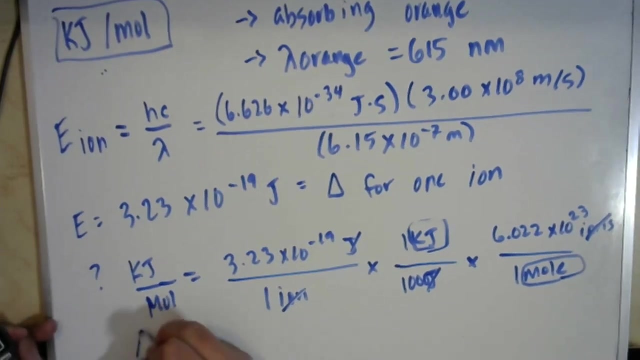 And I'm going to have to use Avogadro's number to get me in terms of moles instead of 10- to the negative 19 joules over moles, which is what I want. All right, So I end up with a crystal field splitting energy of 195 kilojoules per mole. 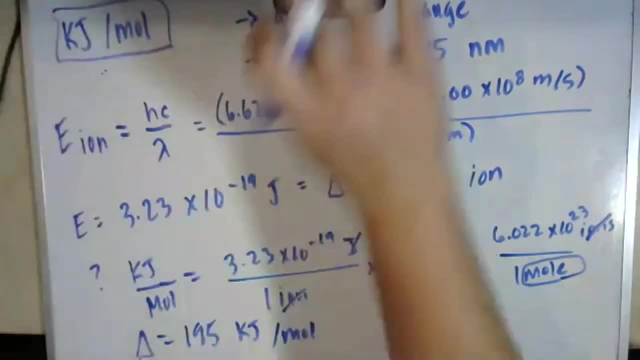 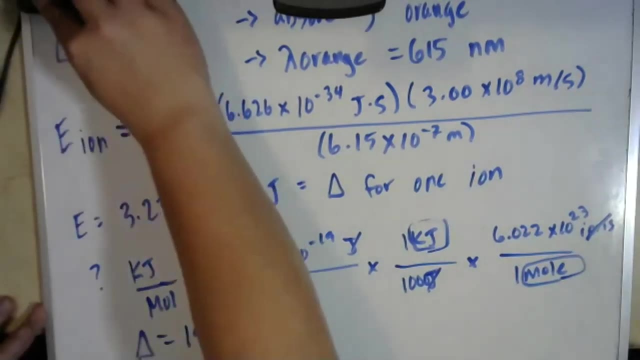 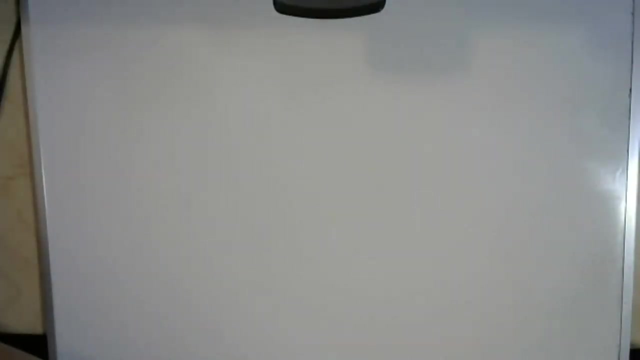 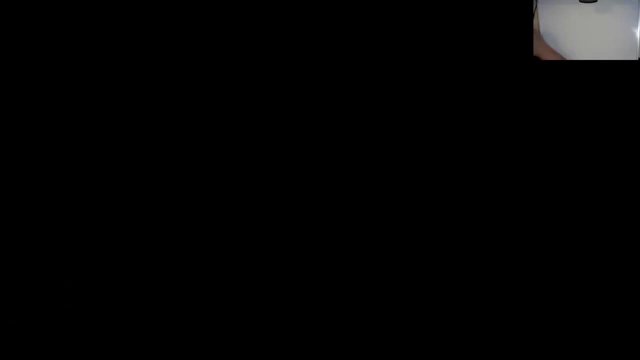 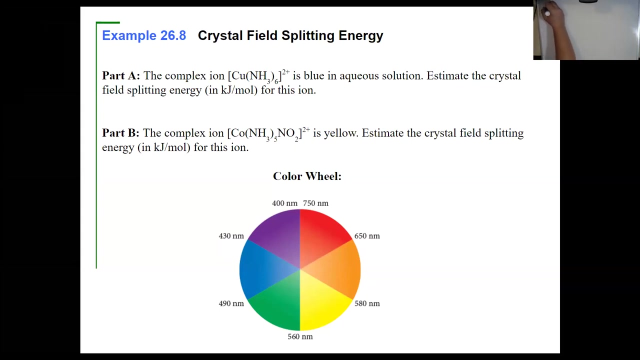 The second example says that our complex ion is yellow And again we're going to be estimating the crystal field splitting energy. So we see that if it's transmitting yellow light, that means it's going to be absorbing violet. Okay, So probably the average of our violet light over here is going to be around 415 nanometers. 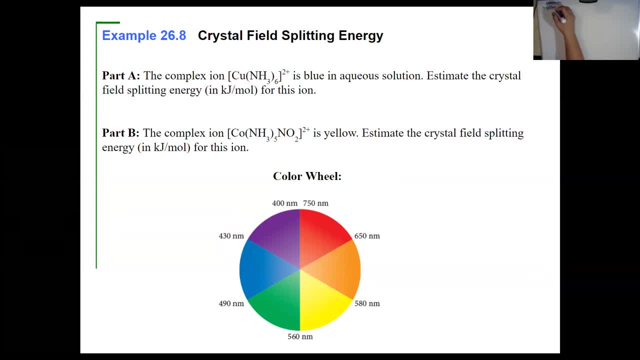 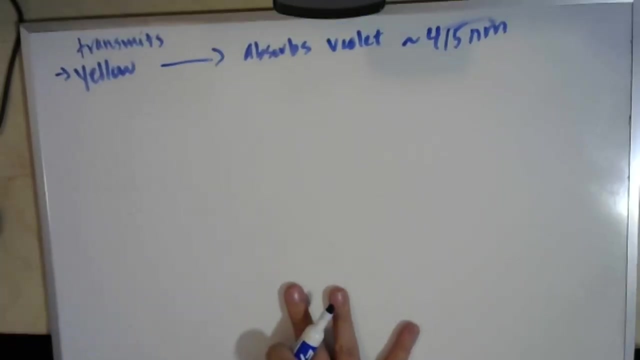 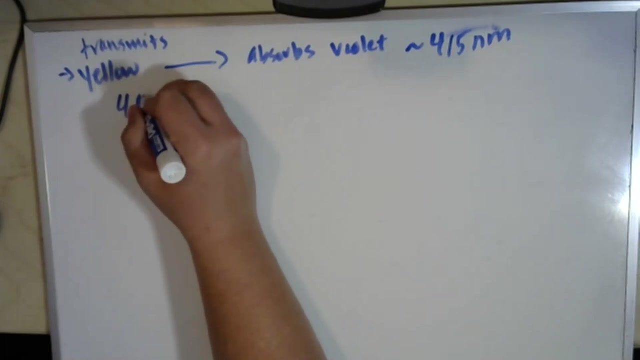 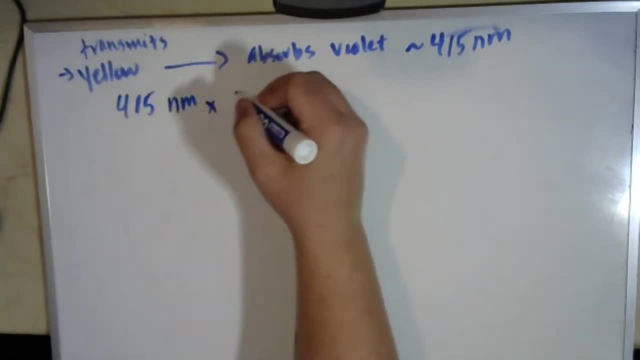 Very good, Very good, Very good, Yeah, Yeah, All right, So this one's the uniquities. an image, Okay, Uh-oh, Okay, Okay. So let's see what we got here in thismir: tiene a nitride. My comment begins with this: The principle of a new planet is that various times light is flashing magnetic beams, So meter value is incredibly important. It's not necessarily the same number of meters that we are also accepting for our work world. We know that will need this number in terms of meters. 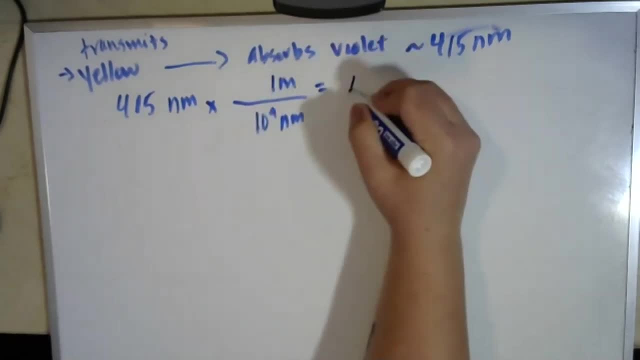 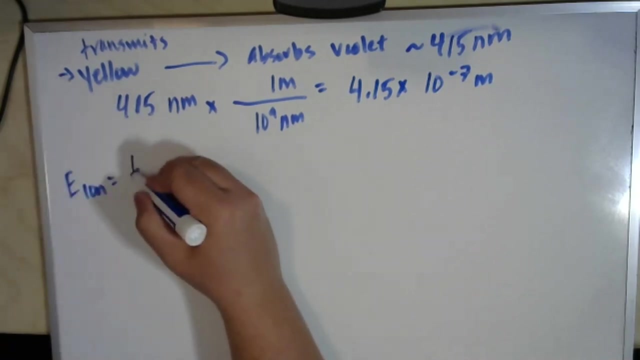 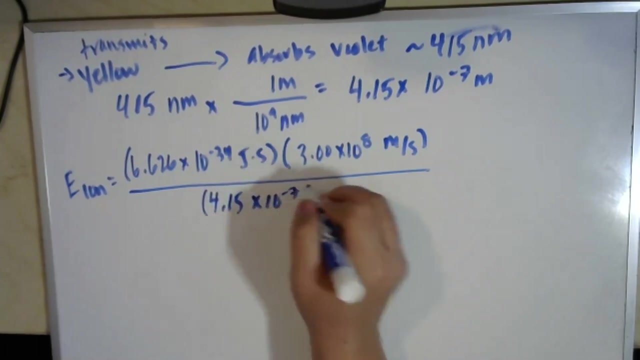 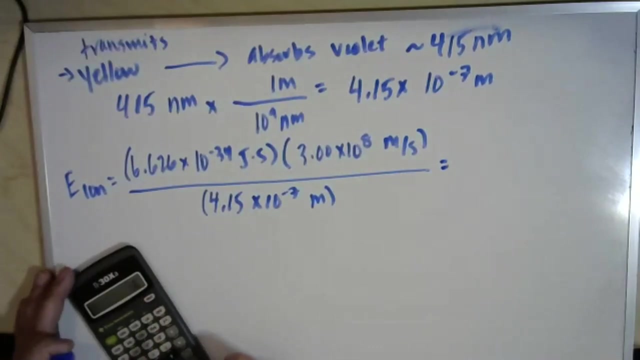 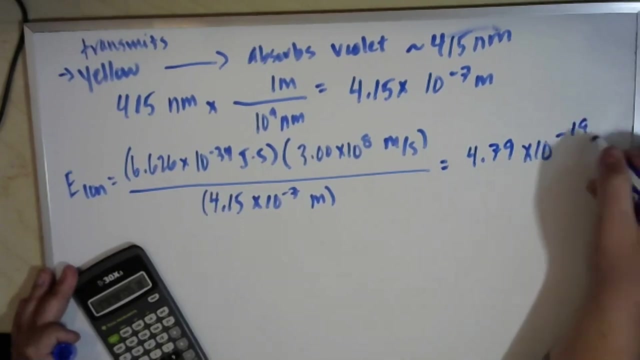 The reason, toying it on one incident of Strawberry到了. Okay, now we can find the energy of an ion using Planck's constant times, the speed of light divided by our wavelength in terms of meters. Okay, so we get 4.79 times 10 to the negative 19 joules per ion. 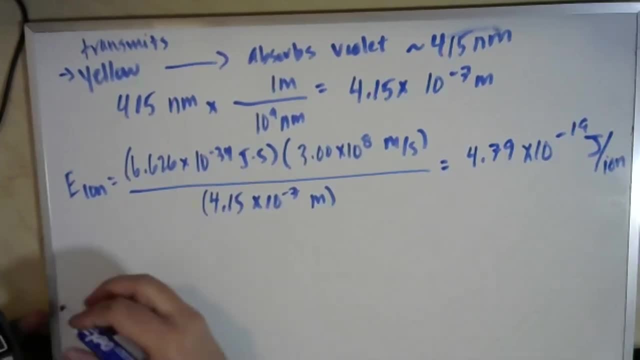 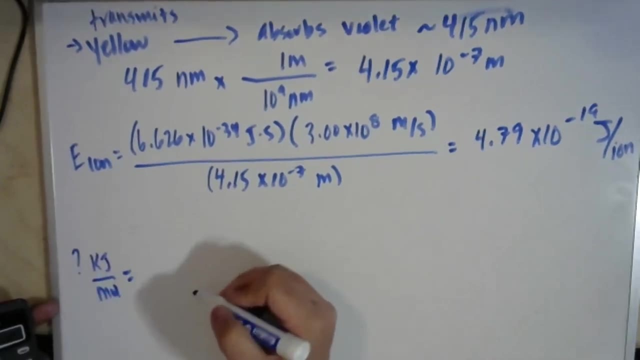 Okay, now we're going to look at that in terms of kilojoules per mole. So how many kilojoules per mole equals 4.79.. 4.79 times 10 to the negative 19 joules per ion. 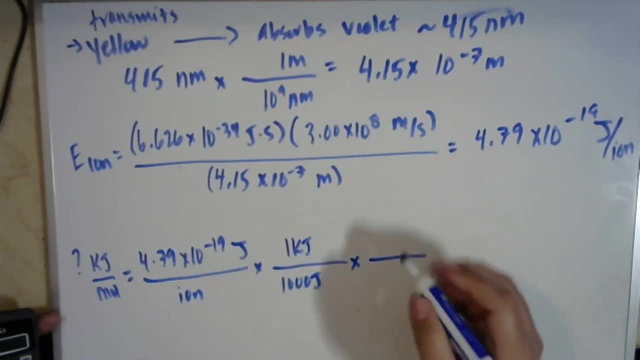 1,000 joules in one kilojoule. In one mole, I have 6.022 times 10 to the 23 ions. Okay, so I end up with 288 kilojoules per mole, And that is my crystal field splitting for this ion. 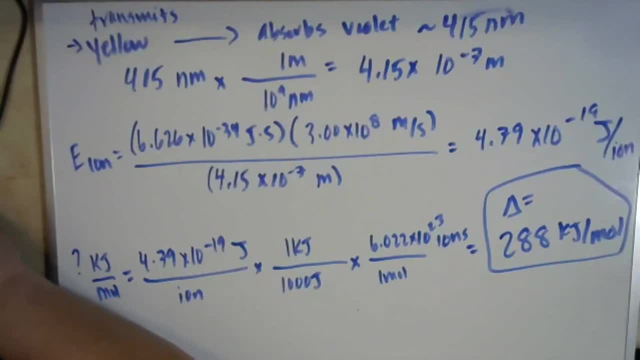 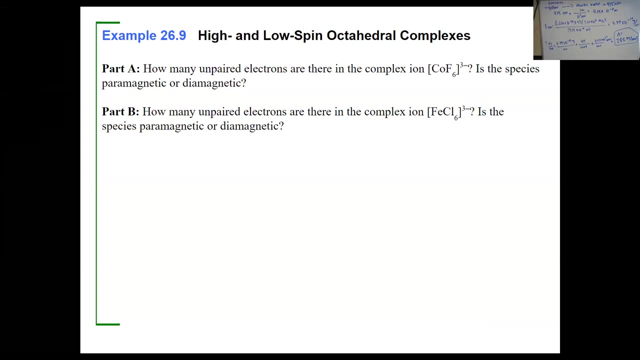 Okay. Next question has us going back into these diagrams. Okay, high and low spin octahedral complexes. So this is where we have to start using the ion configurations that I was talking to you about before. So we're going to be looking at COF63-. 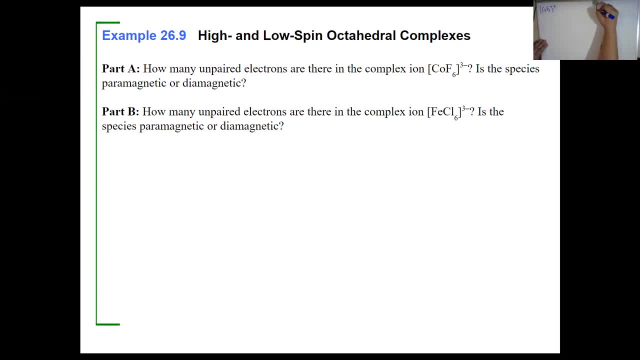 and then FECL63-. Both of these are common, So we're going to be looking at COF63- So we're going to be looking at COF63- And these are complex anions, right, Just to be clear. And what we're looking for is unpaired electrons. 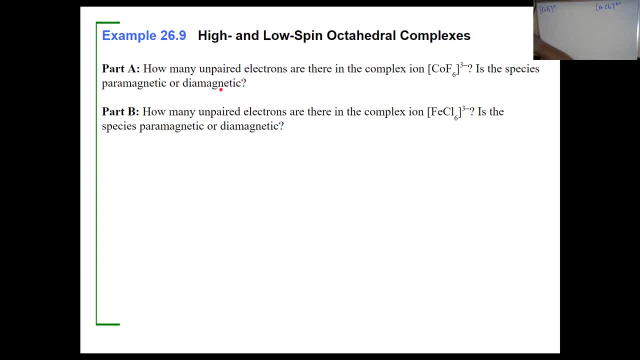 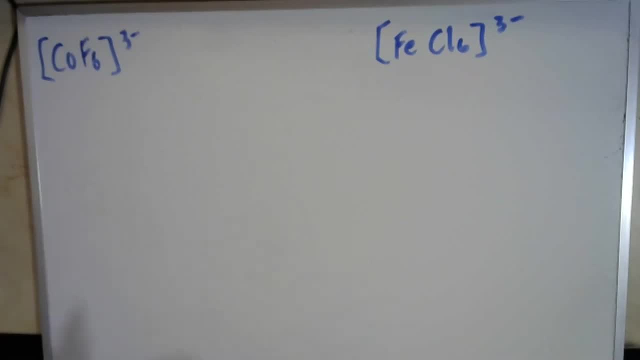 and whether the species is paramagnetic or diamagnetic. All right, So you're going to start any process like this by figuring out how many electrons the central metal has? Okay, so for cobalt, we know that the cobalt ion here is going to be CO3+. right? 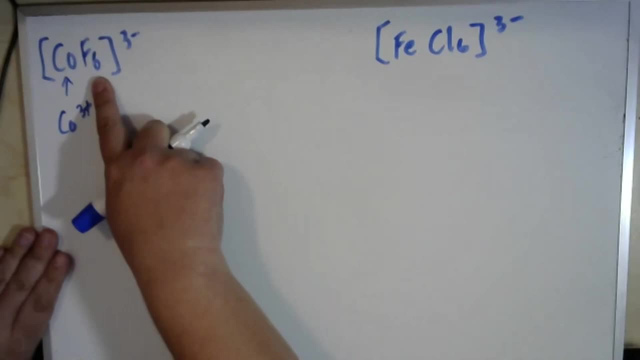 Because there are six fluorines. each fluorine is a negative one, which is a total of negative six. So cobalt has to be a positive three so that they can add together to get negative three. Okay, so now we're going to have the. we need to get the electron configuration for the CO3+. 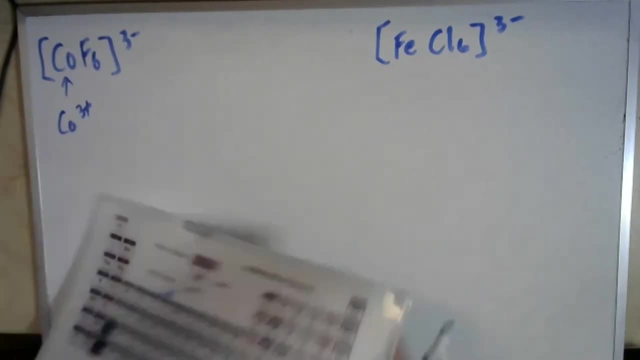 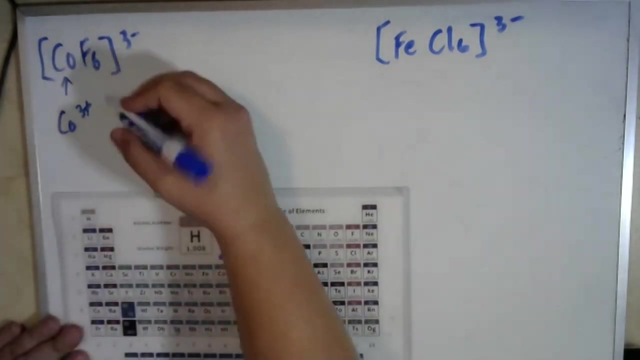 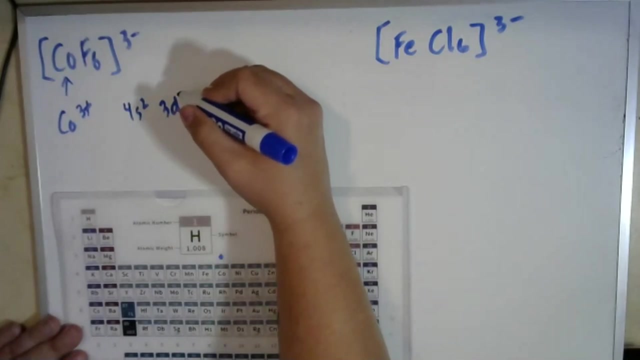 Okay, so we can look at our periodic table. Cobalt's over there, number 27.. Neutral cobalt is going to be 4s2, 3d1,, 2,, 3,, 4,, 5,, 6,, 3d7.. So I'm going to take off these two electrons. So I'm going to take off these two electrons from my 4s because it's the higher energy level. I'm going to take off one of those, So I'm going to be left with three, with six 3d electrons, right? 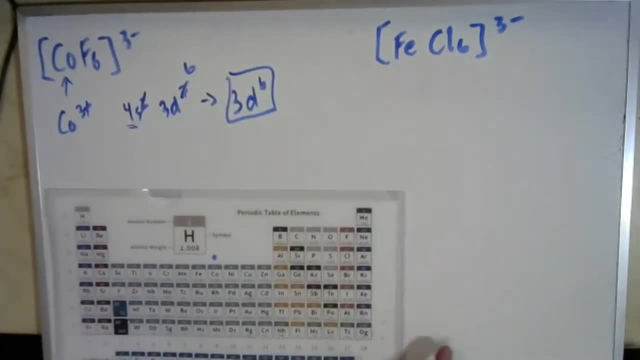 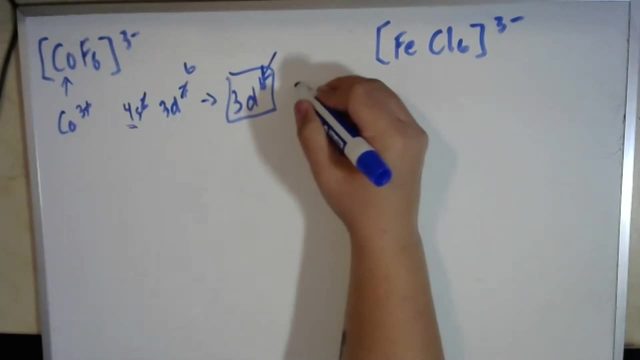 That's going to be what's left over, 3d6.. And that six in the superscript that tells you how many electrons you have to work with. So we have six electrons, All right. Our octahedral complex is talking about the orientation of the five d orbitals. 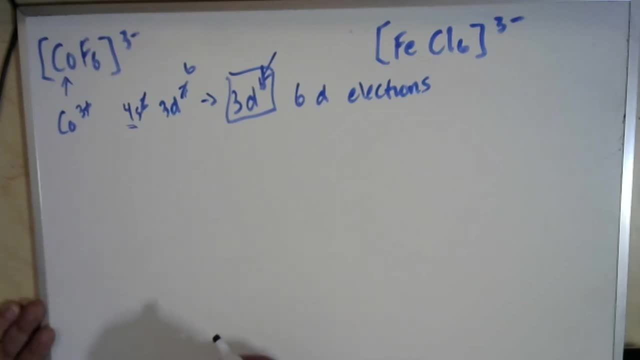 Okay, remember that our d sublevel has five orbitals And, in an octahedral orientation, three of those orbitals are going to be on a lower level than the other two. Okay, Okay, So the distance between here, this is your delta value. 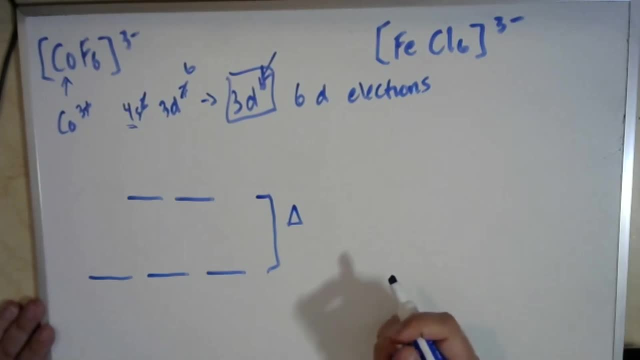 That's your crystal field splitting energy. Okay, All right, When your crystal field splitting energy is small, let's say if, if delta is small, your electrons are able to spread out, because the energy difference between the two levels is negligible And so your electrons can just kind of spread out and follow their ordering rules from your. you know that you've already learned about. 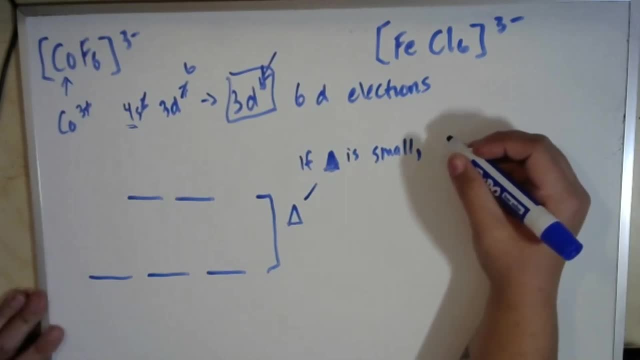 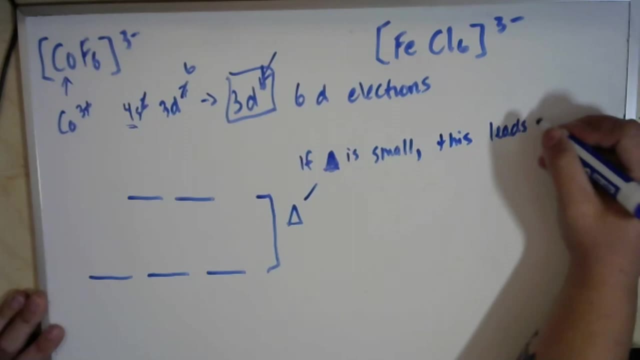 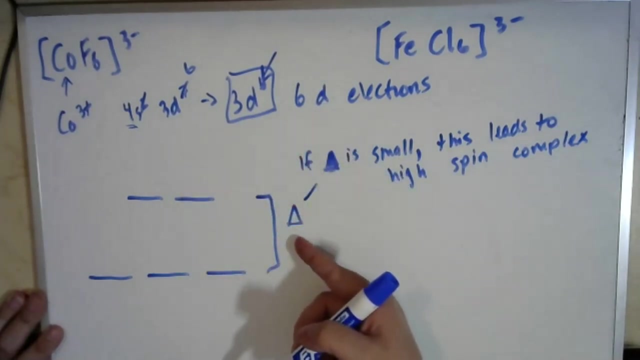 And you end up with what are called high spin complexes. And they're called high spin complexes Because, say that you have six electrons here, right? So if your delta value is very small, then the six of those electrons are just going to, they're going to, like, spread all the way out as much as possible. 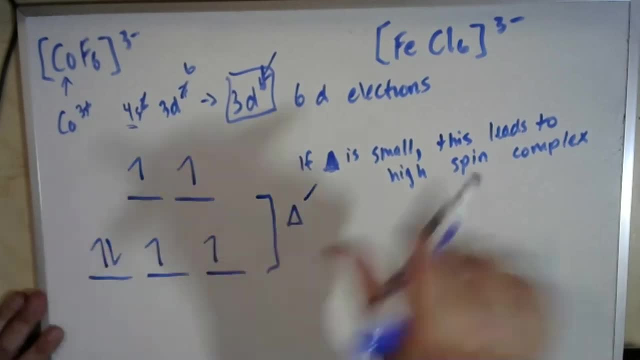 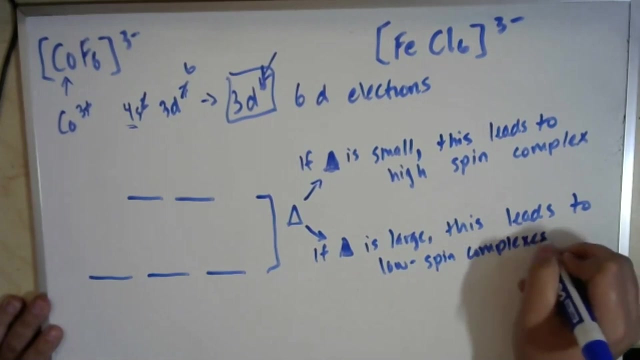 Right, But if your delta value is large, Right, I don't know why I called it and I just wanted to. If delta is large, This leads to what are called low spin complexes. Okay, and that's because electrons- I told the one of the other groups this to electrons- behave a lot like people. 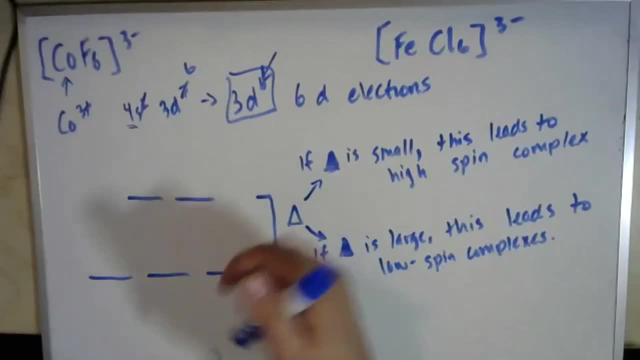 If this delta value gets very big, When that fourth electron has to fill a spot, If the energy is too high, it's going to look up like this giant staircase it has to climb to get up here and it's going to say, no, thank you, I'm not going to go up there. Instead, I'm going to go back to the beginning. 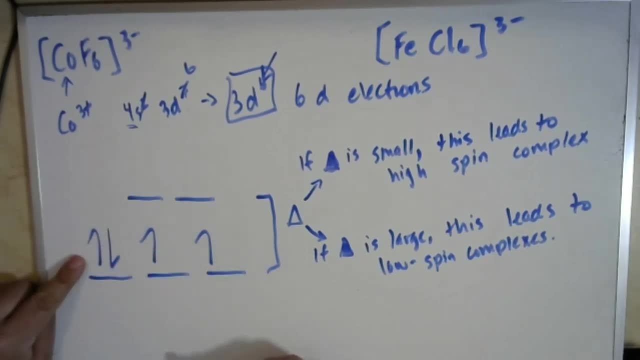 And just sit over here with this guy, because I don't feel like making that climb. Okay, so six electrons in a low spin complex. We'll try to stay on the bottom level with the low energy. So you see how I only end up with one unpaired electron here. 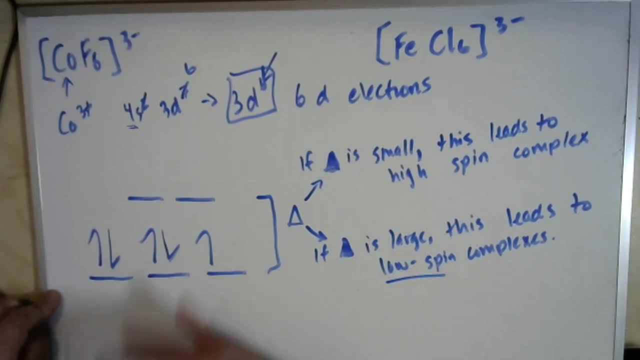 Right, that's why it's called low spin. When all my electrons were spread out, I had four electrons with no pairs. That's high spin. The more single electrons you have, the higher your spin is. The more paired electrons you have, the lower your spin is. 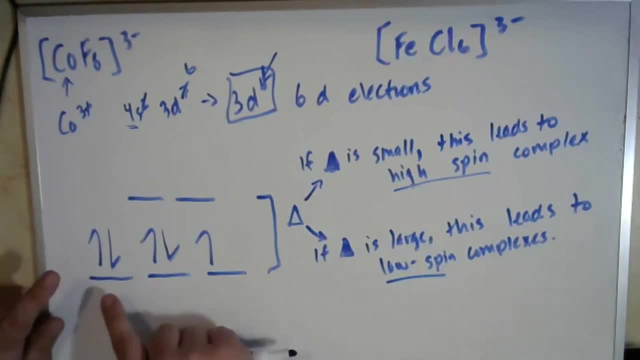 Because when you have two electrons together, Their spins cancel each other out. Okay, Now you, very reasonably, might ask: well, how am I supposed to know if the delta value is big or small? And the answer goes back to this chart that you were given. 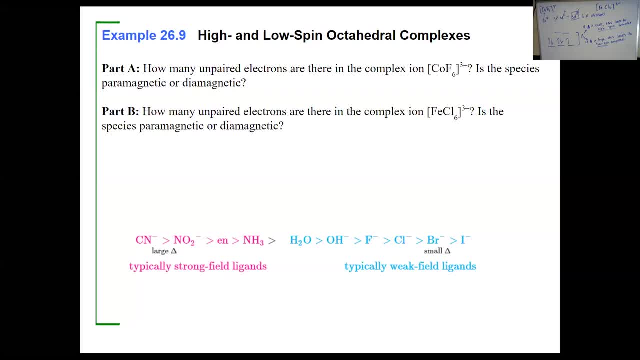 It's in your textbook And it's in your your handouts that Professor Sheehan gave you. Okay, The type of ligand attached to your central mass, To your central metal. Okay, And remember, in this case, in the example we're doing now, the ligand is fluorine. 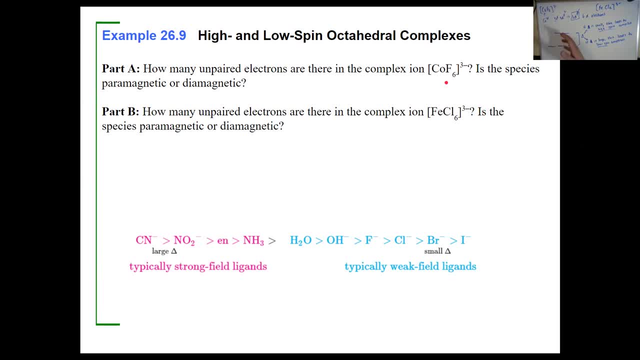 The type of ligand depends whether you have a big delta value or a small delta value. So you see these ligands over here. They're called strong field ligands And these have a large delta value If your central metal is attached to a strong field ligand. 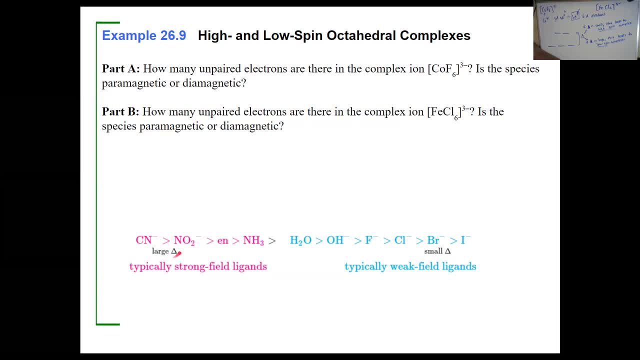 Then they're going to have a low spin complex Because you're going to have such a large space between those energy levels And that top level is going to be at a much higher energy than the lower one If your central metal is attached to a weak field ligand. 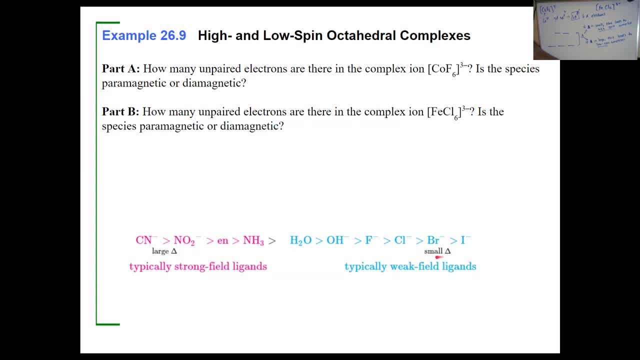 Weak field ligands are going to have a small delta value, A small crystal splitting energy, And that means that the electrons will be able to spread out. Even though you have a like a low level and a higher level, They're still close enough together. 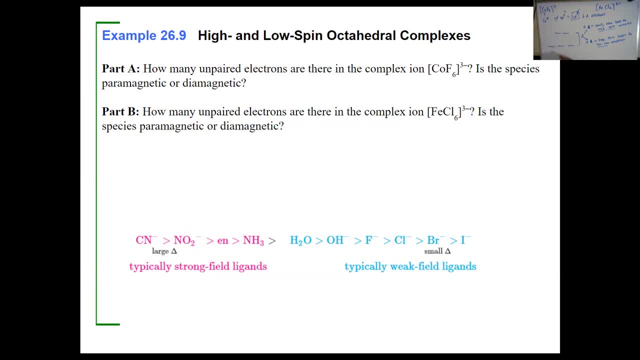 It's like taking a step up a curb Versus climbing up three flights of stairs Right Like going up. one step is not a big deal, And so electrons are able to like spread out in that manner then. Okay, So we have to look at the ligand that's attached. 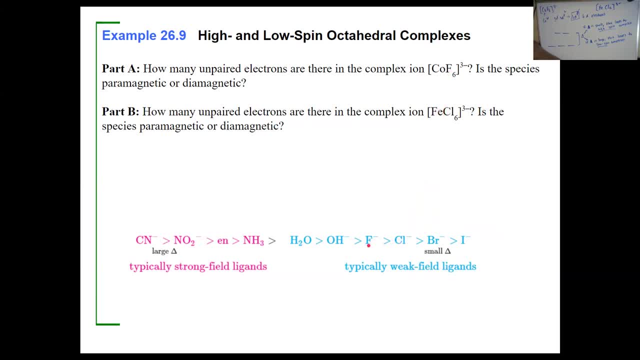 In this case fluorine. We have to find it on the list. Here it is. It says fluorine is typically a weak field ligand, So fluorine is going to have a small delta value. All right, Knowing that We can now distribute our electrons. 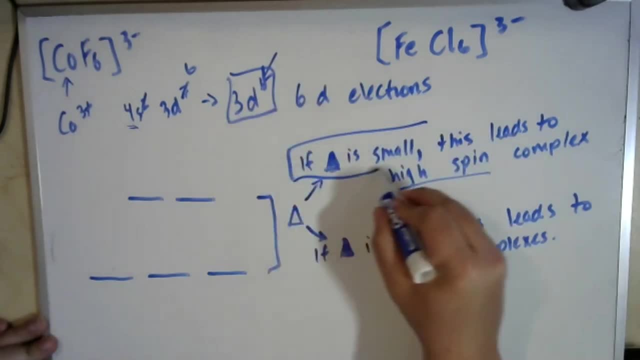 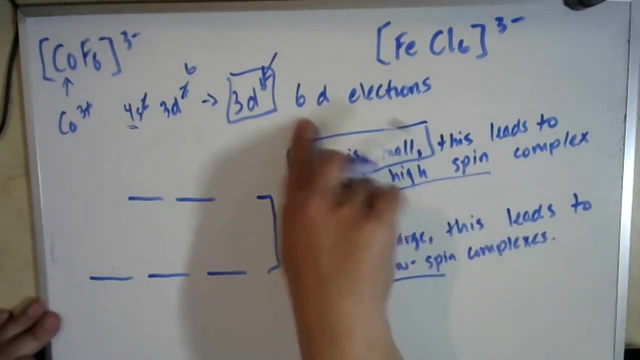 According to this Rule up here, If Delta is small, we're going to have a high spin complex. So our six electrons are going to spread out as much as possible: 1,, 2, 3.. 4,, 5,, 6.. 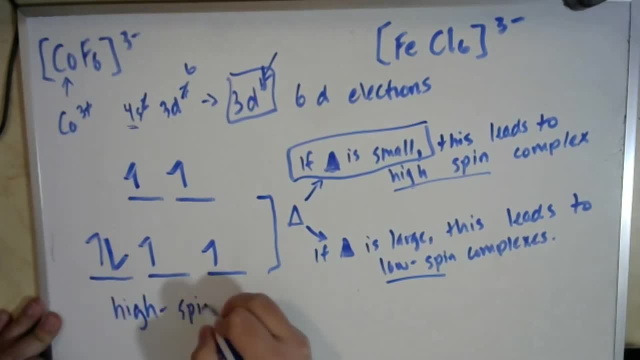 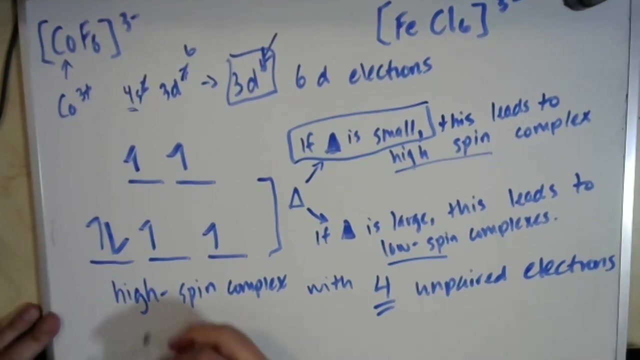 So we're going to have a high spin Complex. Okay, We have a high spin complex With Four Unpaired electrons. When we have any unpaired electrons, This means that our Species is going to be considered para magnetic. 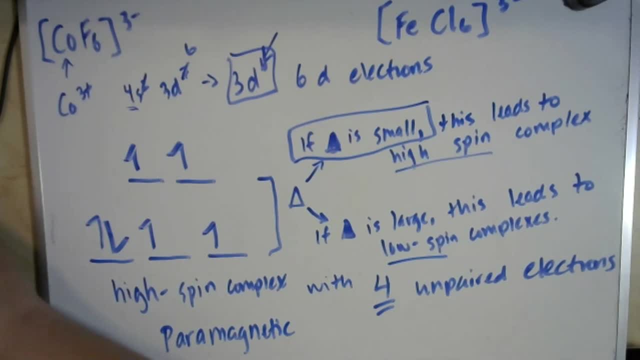 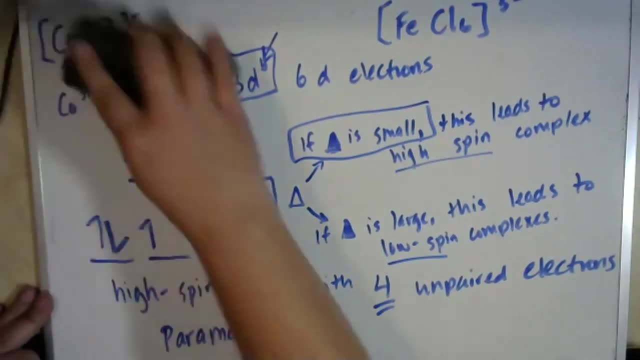 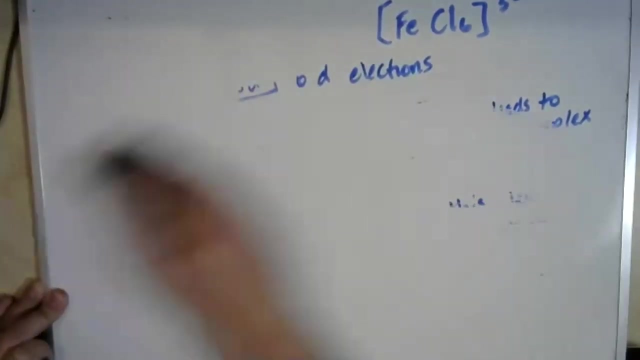 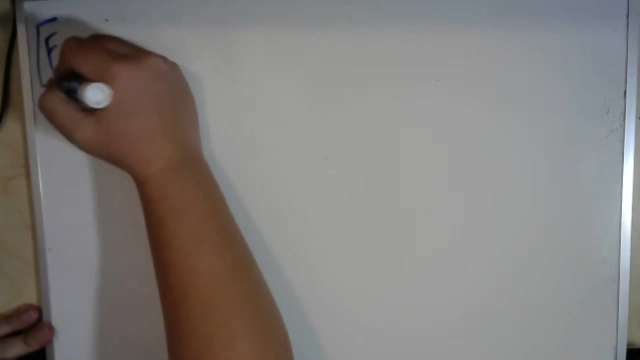 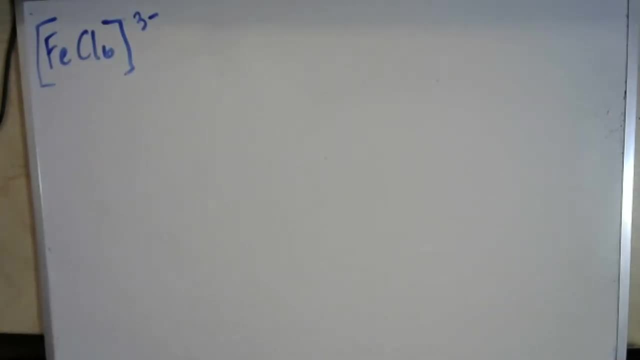 Okay, Okay, Okay, Okay, All right. So right off the bat I'm going to want to figure out What my charges over here. I have six chlorine. That's going to be a negative six. I have a negative three charge overall. 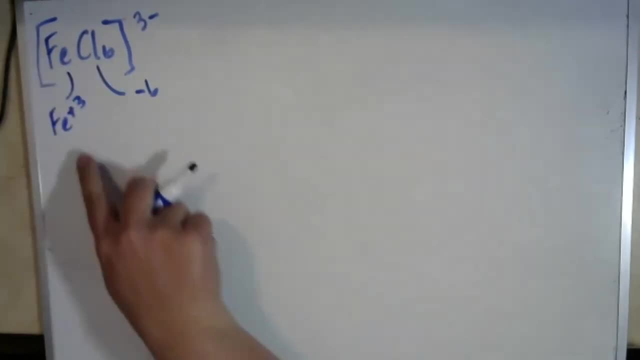 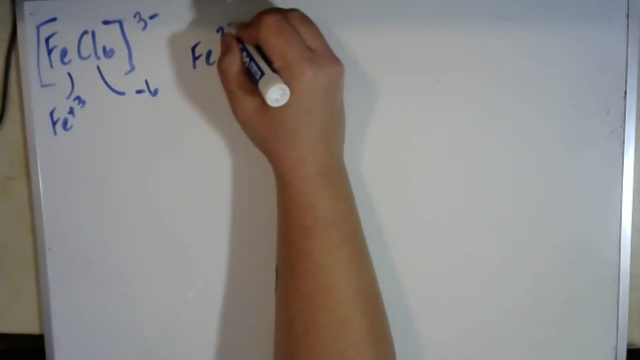 That means that iron is going to have to be a positive three, Right Cause positive three and negative six equals negative three. So I have to find the electron configuration for the F? E three plus ion. So I have to find the electron configuration for the F? E three plus iron. 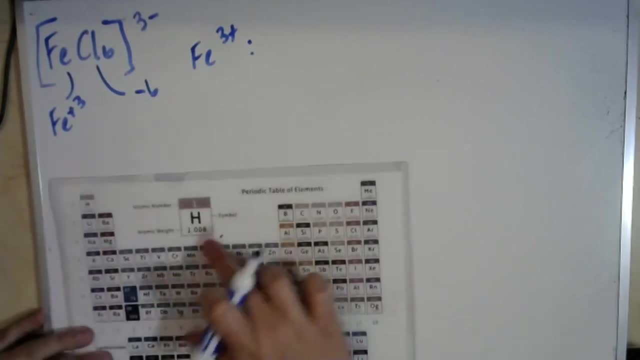 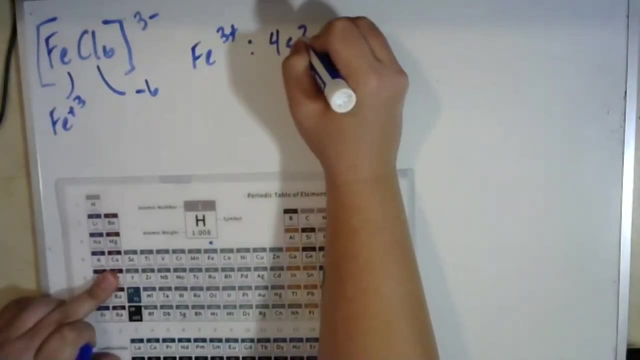 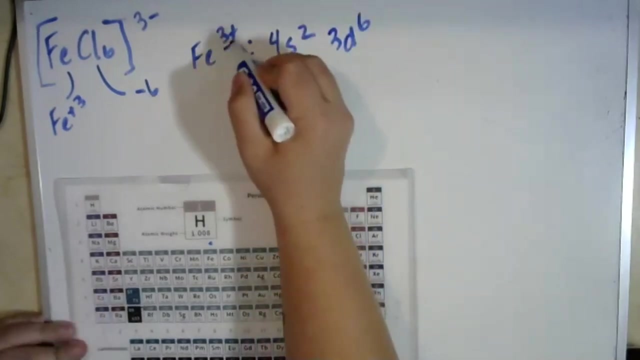 okay, go find iron. it's number 26, so neutral iron is going to be 4s2. 1, 2, 3, 4, 5, 6, 3d6, and i'm going to remove three electrons. so i'm going to remove these two. 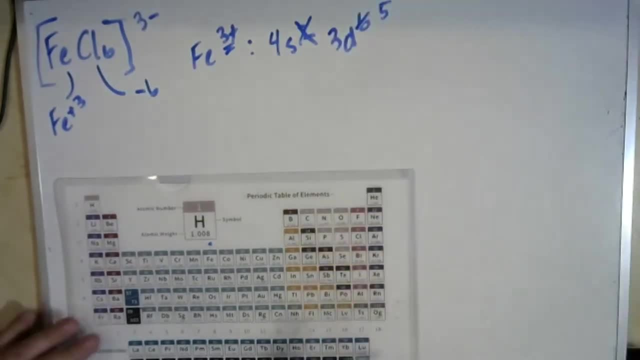 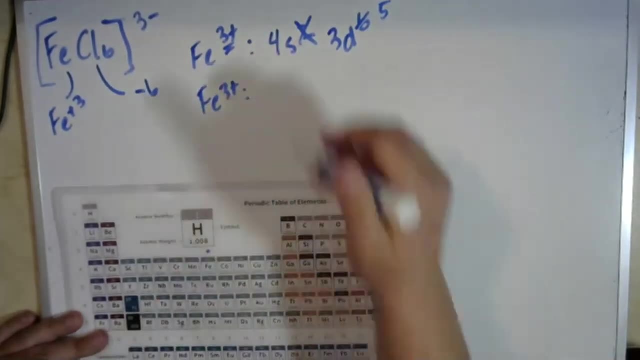 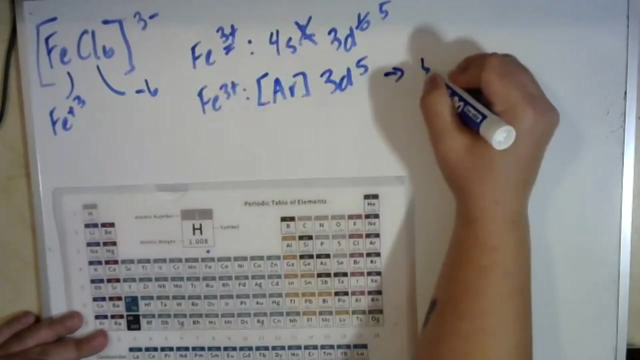 and then one of these. okay, so my fe3 plus is going to be- if we want to be, make it official, put the argon out front- ar3d5. but what we're concerned with is that we have 5d electrons, because those are the 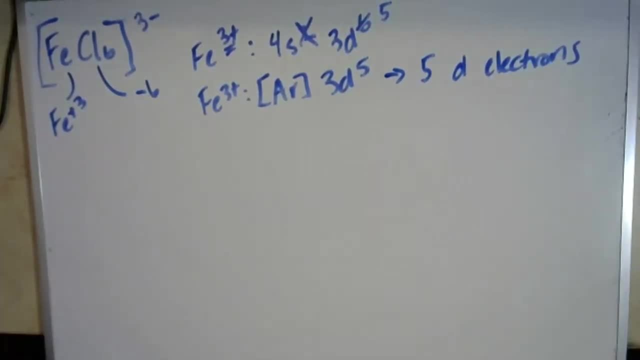 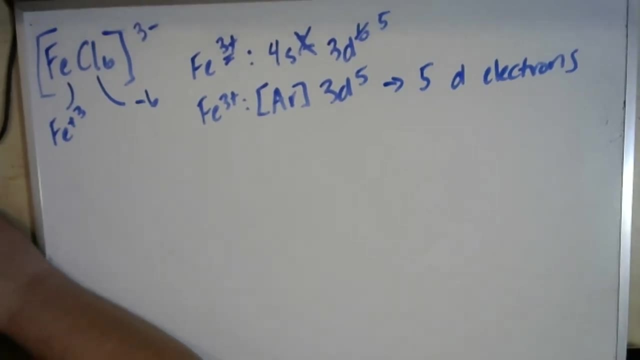 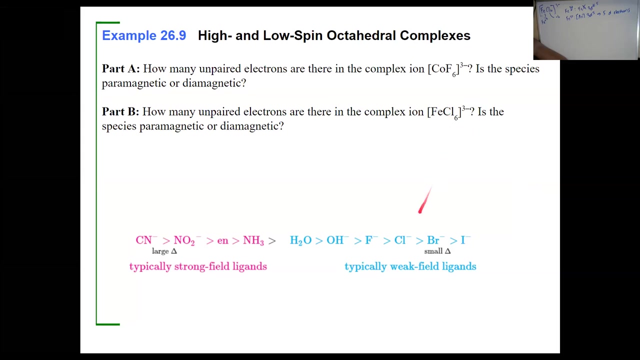 electrons that we're going to distribute in our octahedral array and what we can also see right away- i'll share the screen again so we can look at it together- is that our iron is attached to chlorine, and chlorine is typically a weak field ligand, so 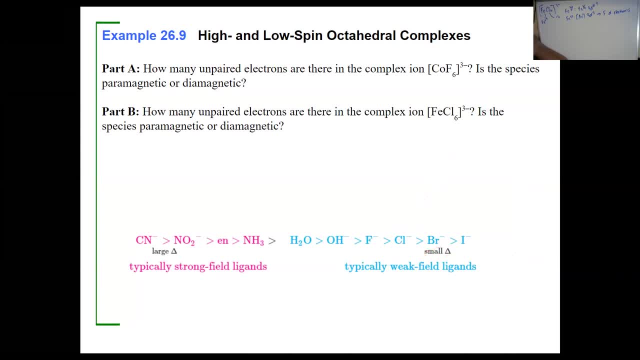 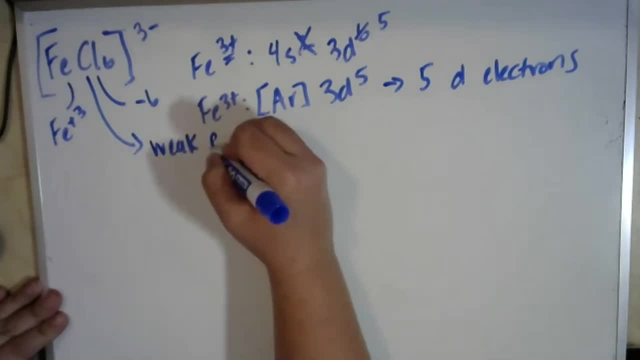 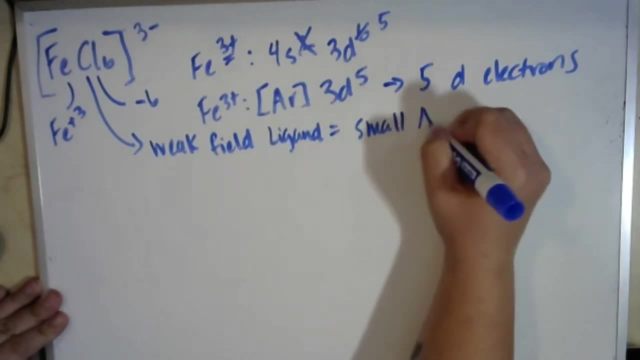 it's also going to have a small delta value, all right, so we have to keep that in mind. weak field ligand, small crystal splitting energy, small delta value. so now, when we are going to set up our octahedral diagram, we have 5d electrons to distribute. we have a small delta value. 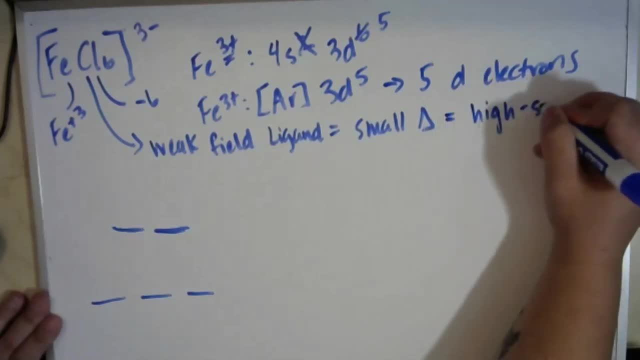 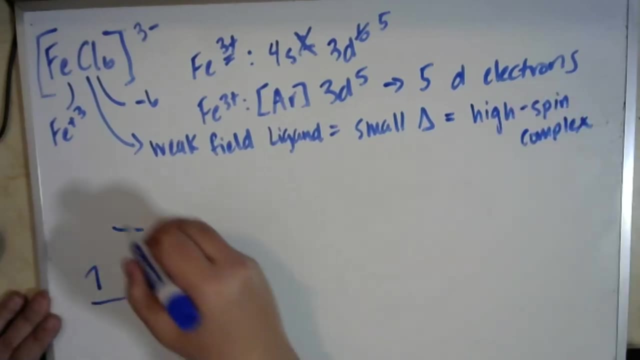 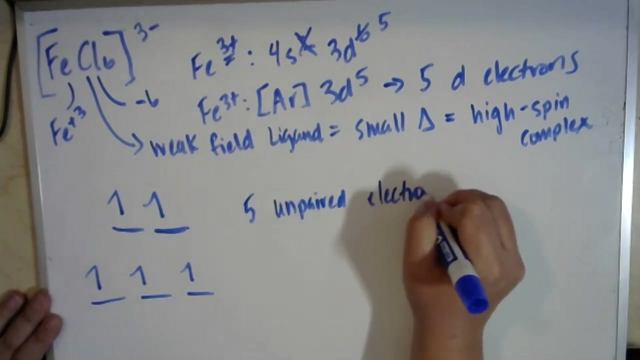 that means that we're going to have a high spin, complex one, two, three, four, five, right? so what we end up with is 5d electrons, right? so what we'reating in the vraiment mass gap is 7d pluralities, which is the necesity figure, because it's from possible. 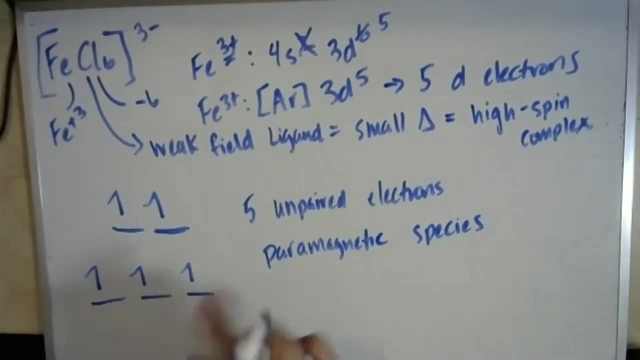 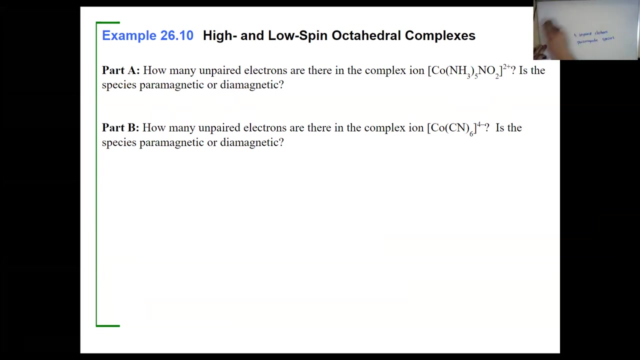 first, 5d is square or scale, so we're going to use seven. seventh here, inows. And let's look at two more examples of this. I did not want that, Oh well, Share screen, Okay. so we're gonna look at two more examples. 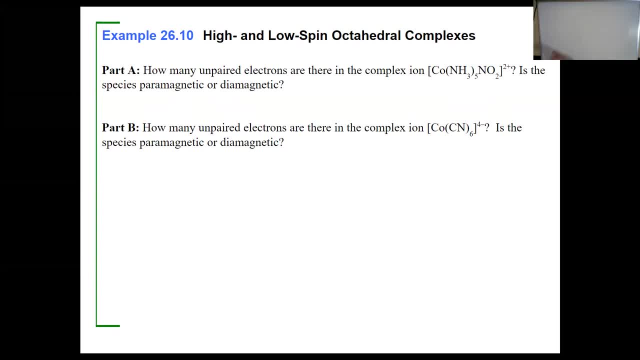 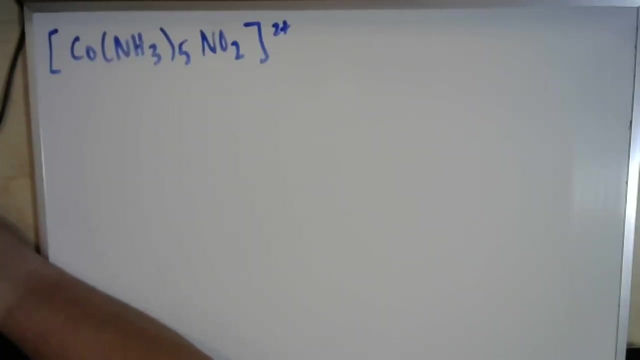 Unsurprisingly, they're giving us strong field ligands to consider now so that we can see how it's different. So we're gonna have, we're gonna start with CO, NH3, 5,, NO2, 2+. Okay, so I want you to go through and first of all, 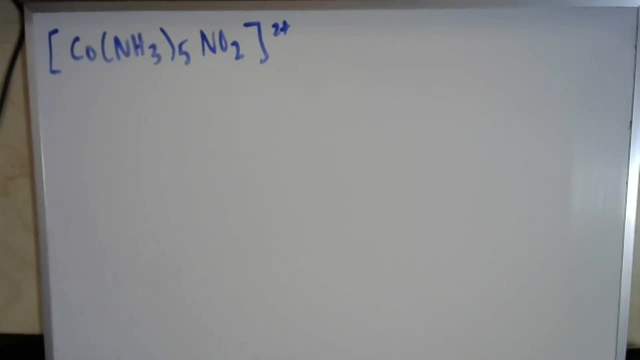 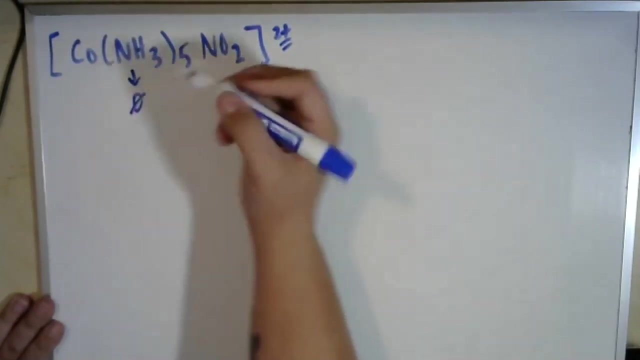 figure out what the charge is on the cobalt here, Because we're gonna need to do that before we can distribute the electrons in our diagram. We know that the overall charge is positive. 2. We know that the NH3 has a charge of zero. 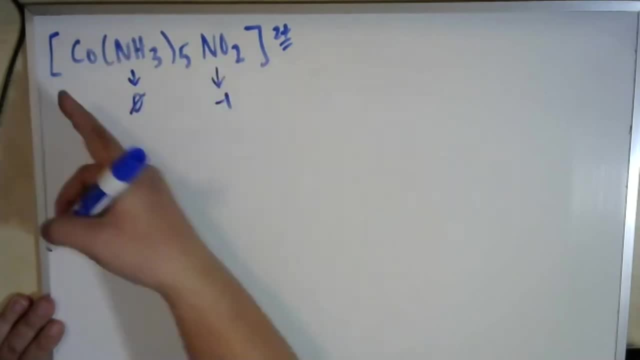 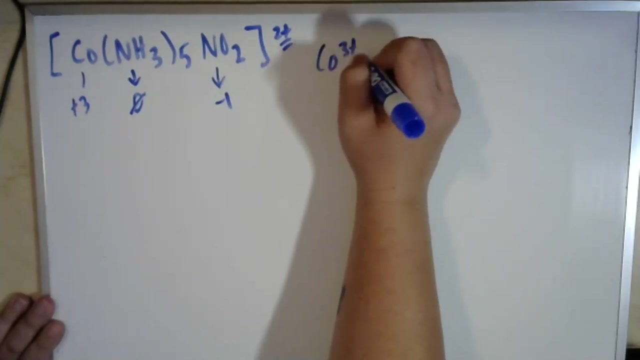 and we know that NO2 has a charge of negative one. That means that the cobalt is gonna have to be positive three for us to get a positive two charge back out. Okay, That means that we have to find the electron configuration for that. 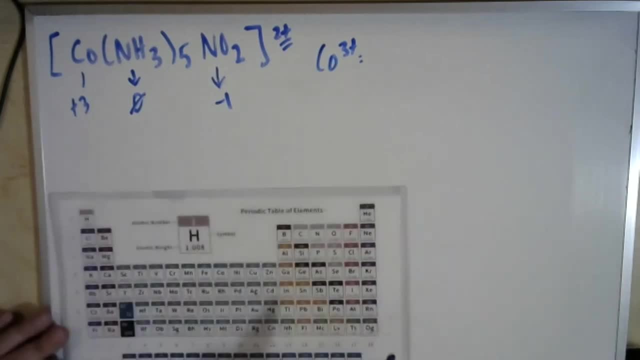 Where did it pick up here? Okay, so we're going back to the cobalt which starts here. Okay, so we're going back to the cobalt which starts here. Okay, so we're going back to the cobalt which starts here. 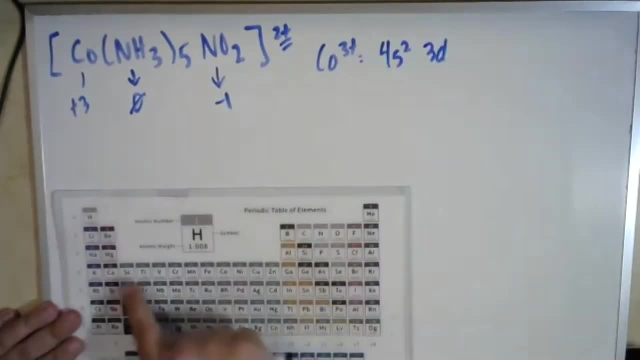 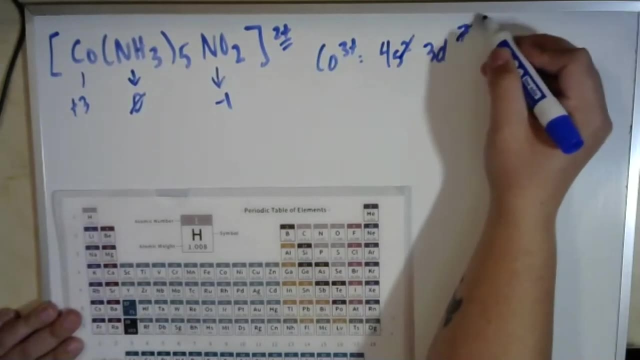 Starts with four S2, three D. one, two, three, four, five, six, seven. We're removing two electrons there, one electron here. Okay, so we're three D, six again. So we have six D electrons. 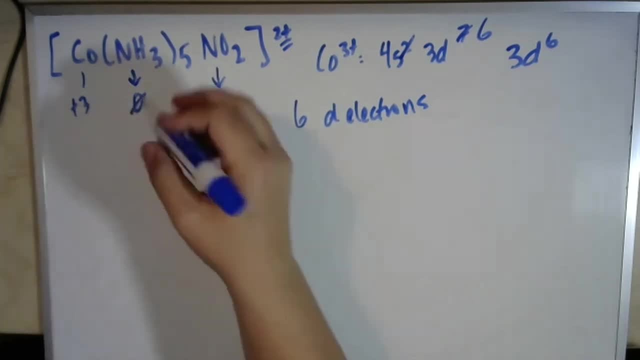 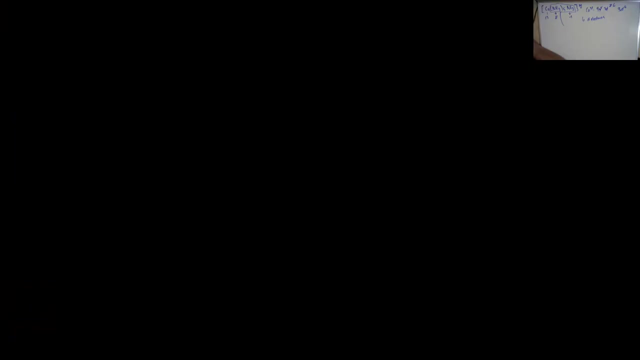 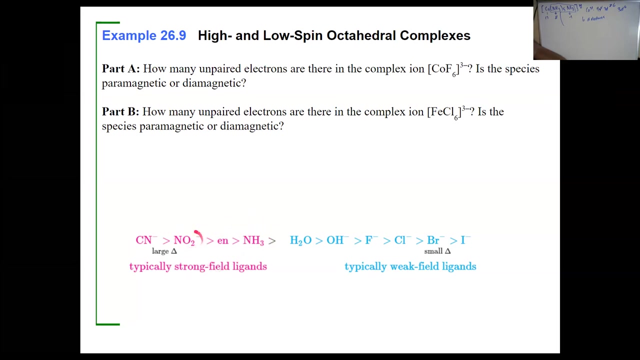 All right, What we have here terms of our ligands. We have NH3 and we have NO2.. If we look back at our list, okay, we're sharing it again now. NH3 is a strong field ligand, NO2 minus is a strong field ligand. 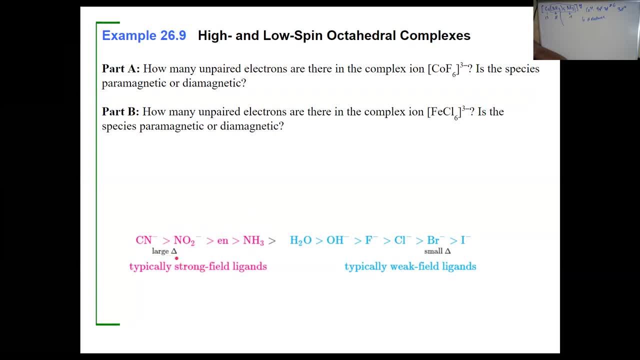 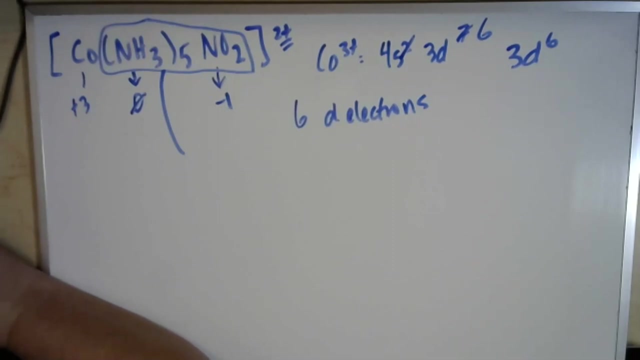 Both of these have a large delta value. okay, So we're going to end up with a very big difference between energy levels of the bottom level and top level When we have a large delta value. this is going to favor your low spin complexes, So let's draw this out. 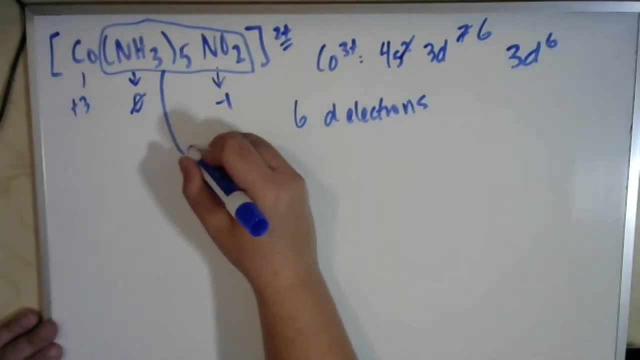 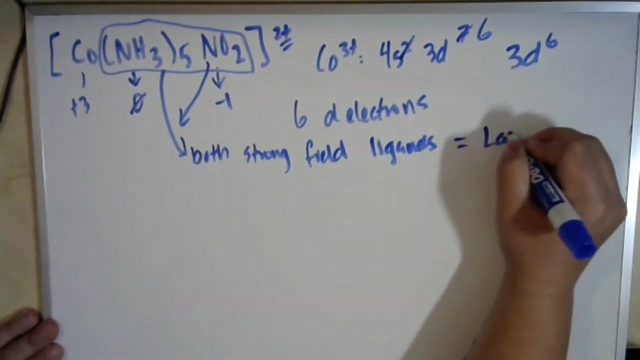 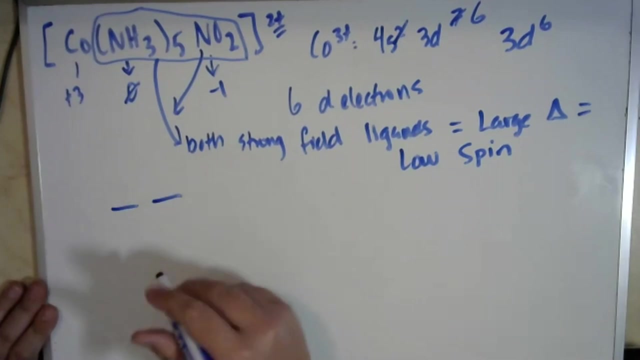 Okay, So we have sometimes, when I'm drawing this out, I like to make it like dramatically different, so it's like like that's your top level and then like your bottom level will be like down here, so you can like really see the large delta value. 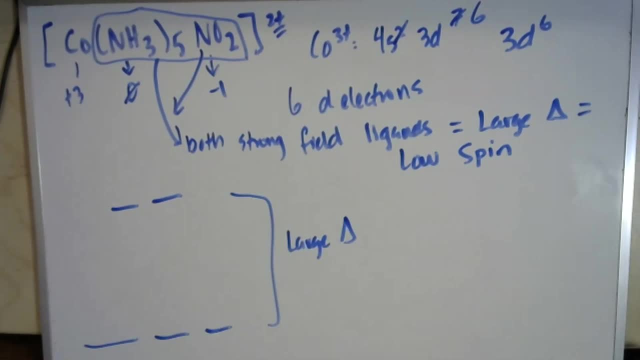 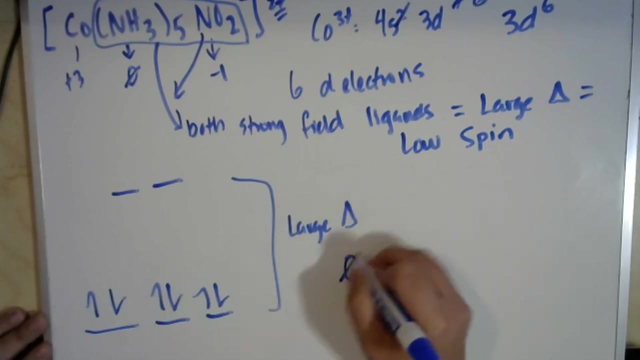 okay, we have six electrons here, so they're going to go one, two, three, and then that fourth electron is going to look up there and go. nope, let's go back to the beginning. four, five, six. okay, this is a case where we finally see a diamagnetic species. here we have zero unpaired electrons. 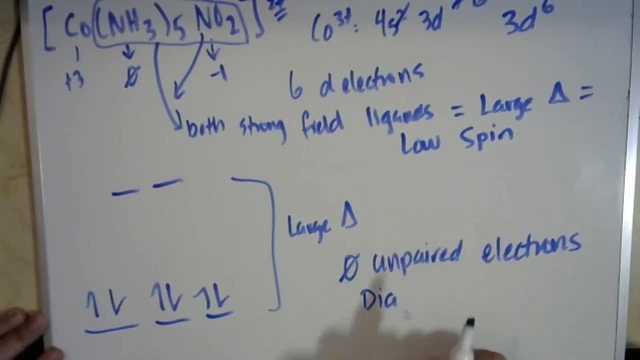 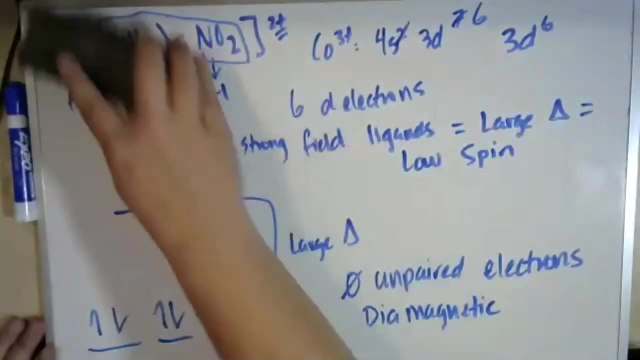 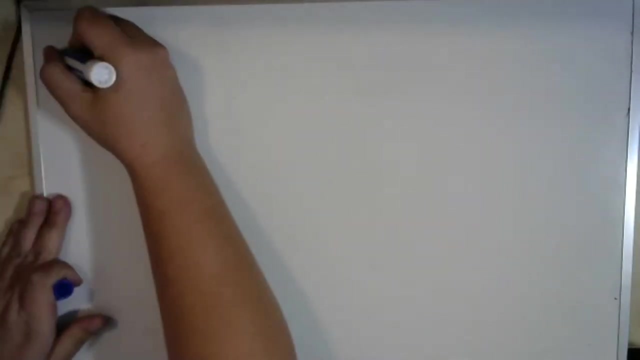 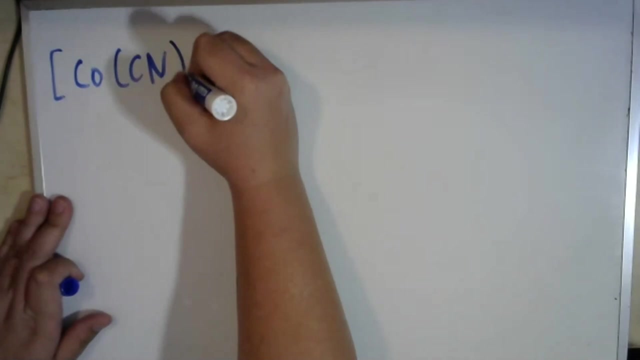 and our ion is diamagnetic. all right, so let's go again at one more example. This one's going to be C O C N, 6, 4 minus. Okay, right away we should be able to look at the cyanide. Cyanide is a strong field ligand. You have to know all of. 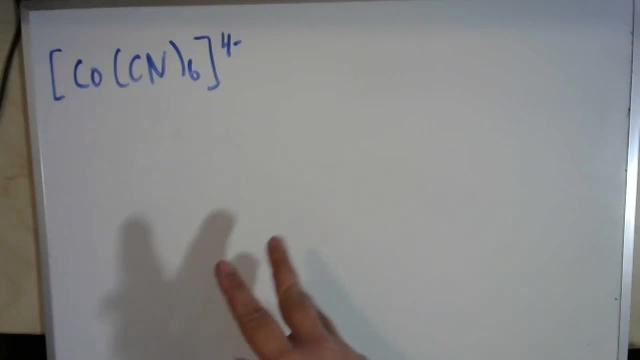 your strong field ligands and weak field ligands by heart. You're not going to have that list on the exam. So take the time you know. if you just want to remember what the strong ligands are so that you can be confident that the other ones are weak, that's fine, But you have to be able to. 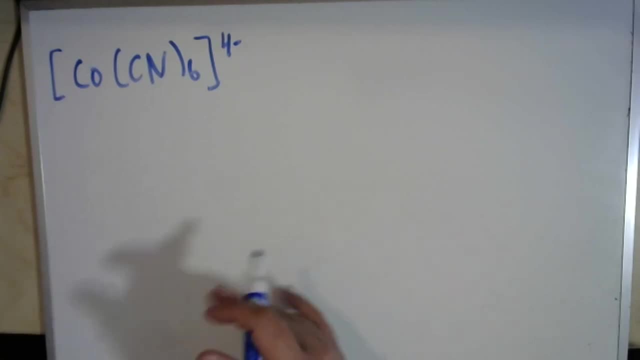 pick out the strong field ligands from the weak field ligands. Okay, so we know that cyanide is a strong field ligand. So, again, we're going to have a large delta value and it's going to favor a low spin orientation, if it has the choice- You don't always have a. 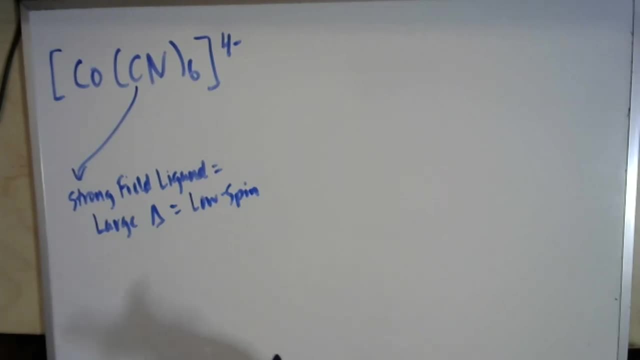 choice with it. Sometimes there are too few electrons or too many electrons and the electrons are forced into a certain orientation, Okay. but if it has a choice, it's going to choose a strong field ligand. So again, we're going to have a large delta value. 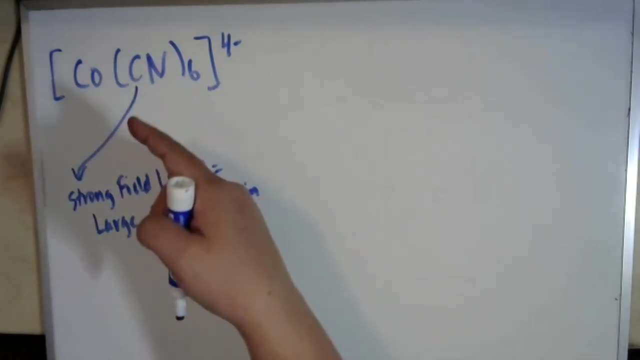 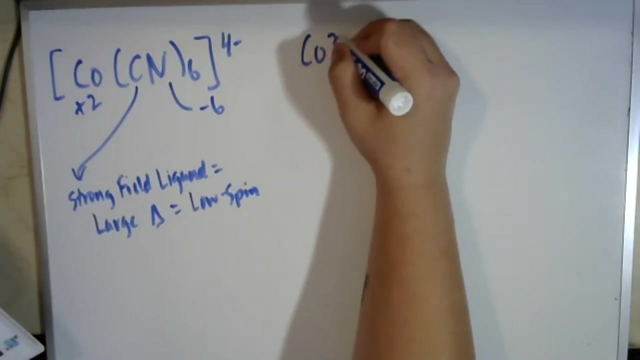 and it's going to favor a low spin complex. As far as the charge, we have a negative six total from the six cyanides, an overall charge of negative four. That means our cobalt is going to be positive two. So again, you know I'll rewrite this every time, just. 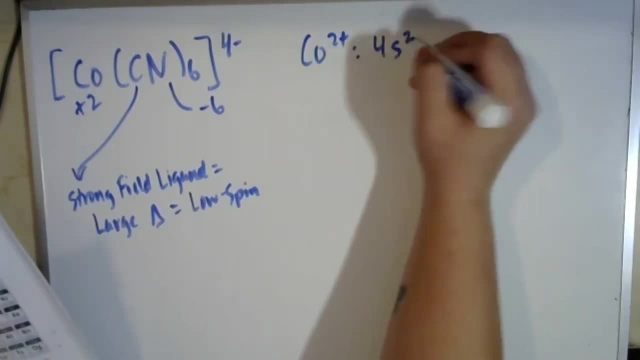 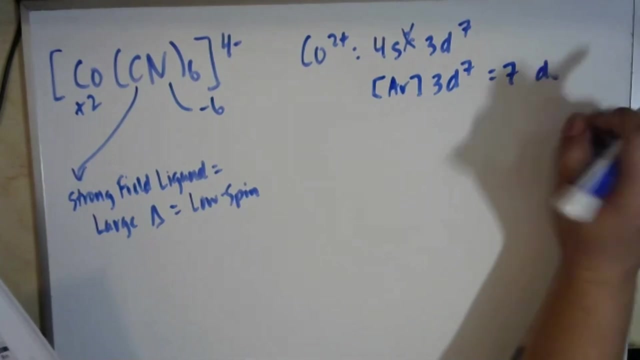 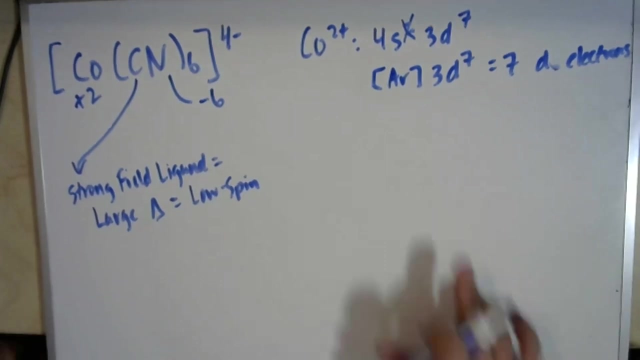 so we're all on the same page. We're going to start out with 4s2, 3d7, and we're going to remove these two electrons, So we're going to end up with 7d electrons. Okay, and if our 7d electrons are going to be trying to fill, 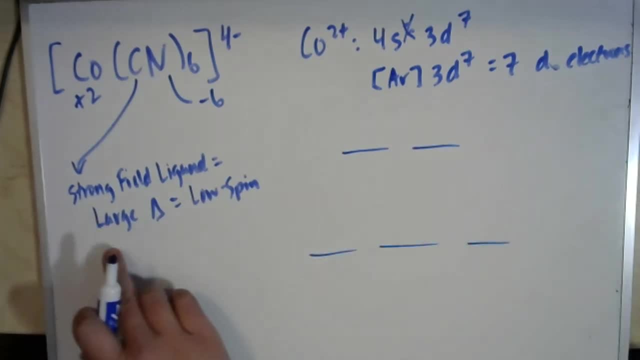 this strong field orientation, with this very again large delta value. here your electrons are going to go: one, two, three. electron number four is going to say: I'm staying down here. four, five, six, and in this case that seventh electron is going to be forced up top because there's nowhere for it to go. 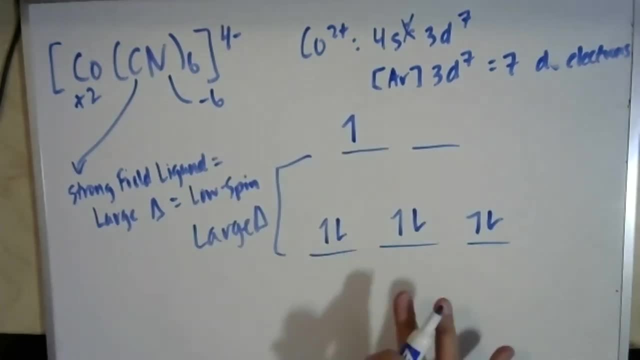 so when all of our electrons are distributed in this low spin complex, we end up with one unpaired electron, which gives us a paramagnetic species. it's still a low spin complex because it still has many electrons that are paired, but it does have some magnetism.